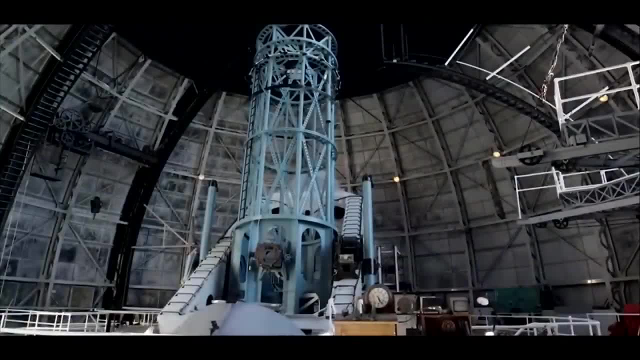 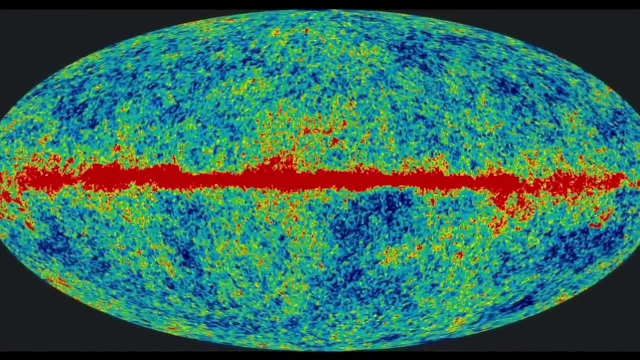 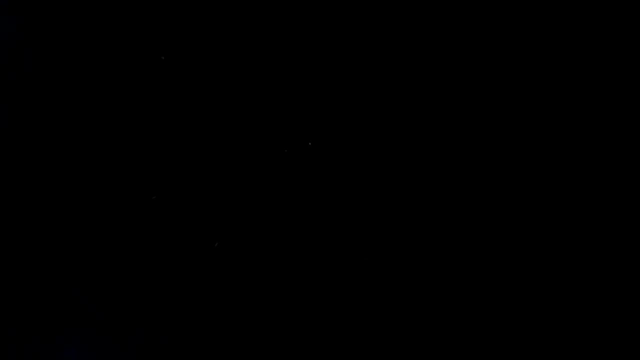 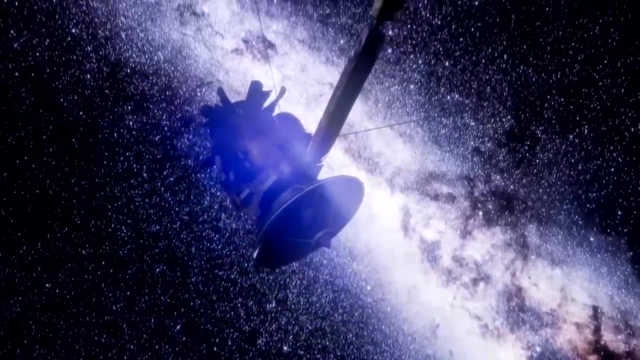 about observing distant objects in space is that the light registered from these objects today has traveled throughout the universe for a long time and, in actual fact, was emitted an extremely long time ago. thus, objects located at cosmologically large distances are objects that have existed since the beginning of time and emitted the light that we register very 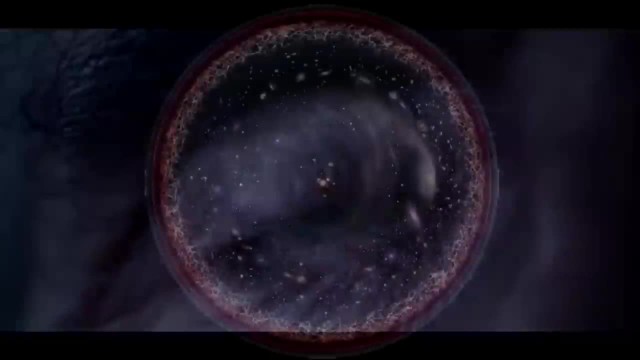 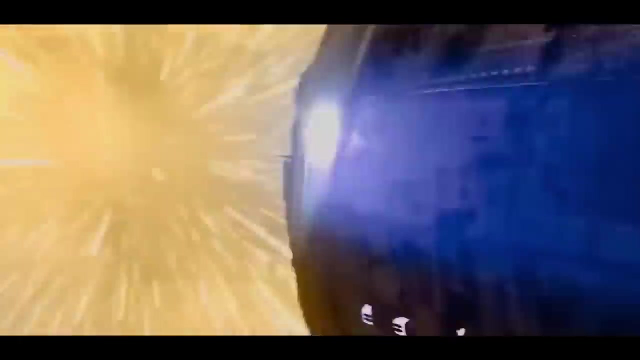 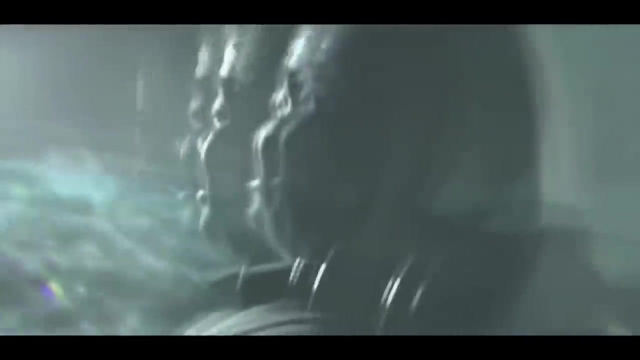 very early on. the very earliest signal, of which we are aware and have studied well, is the extraordinary cosmic microwave background radiation, which appeared in the era of hydrogen formation, when there were no galaxies or stars. at that distant time, the universe was a billion times denser and photons. 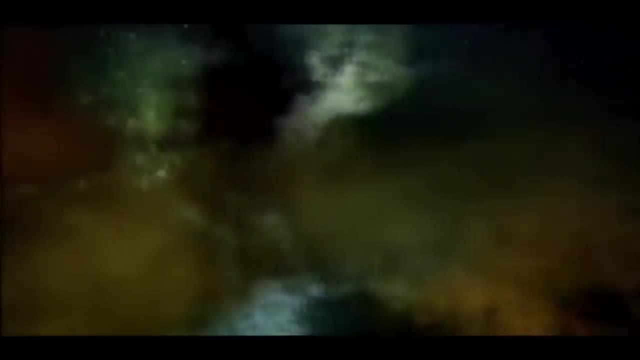 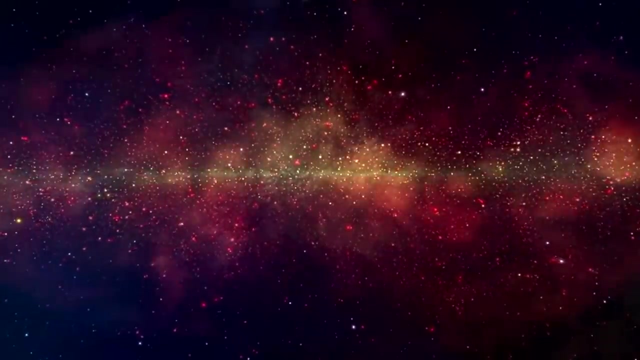 were a thousand times hotter than they are today. as these photons spread throughout the universe, it was expanding. by reviewing microwave research, information can be obtained about the characteristics of the microwave radiation and the radiation of the microwave radiation, characteristics of the expansion of the universe, its composition and 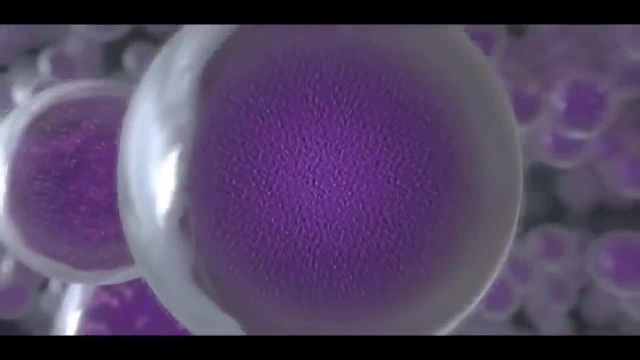 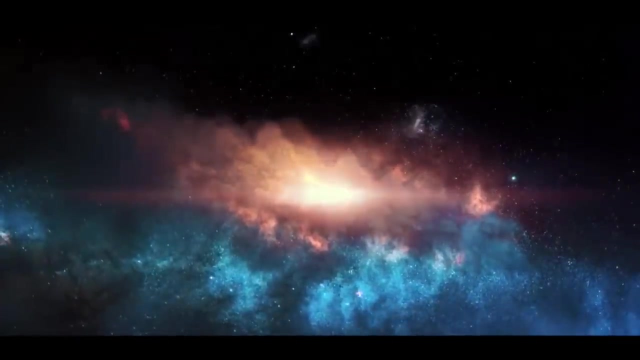 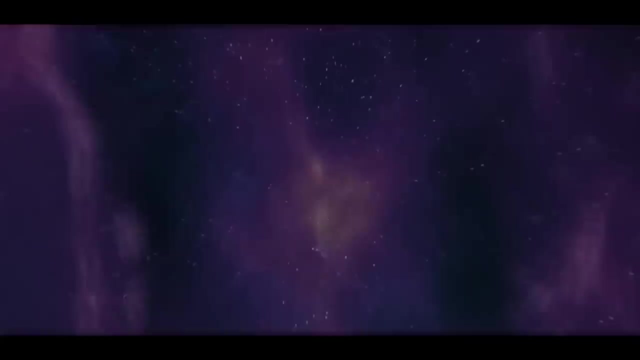 internal structure. the most distant region that is possible to see and distinguish is the last scattering surface. it is from there that the cosmic microwave background photons emanate. this is the so-called surface of the last scattering beyond this region is what is not yet subject to study by our 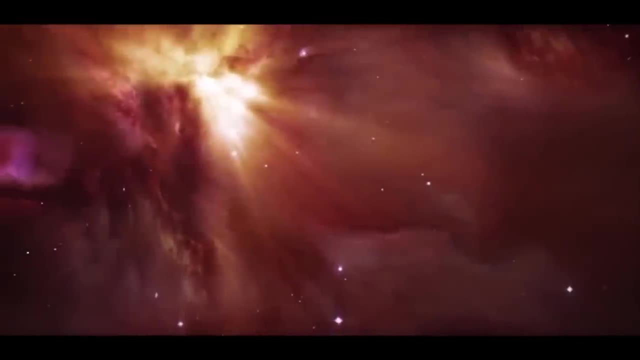 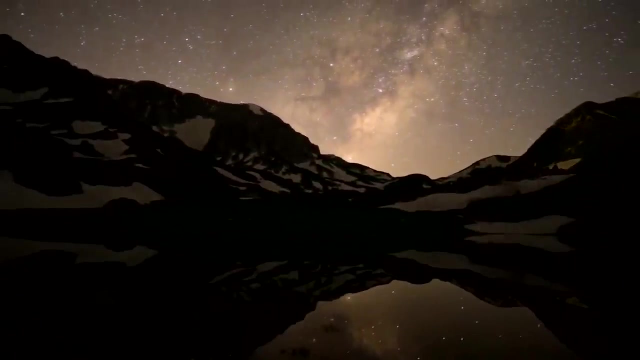 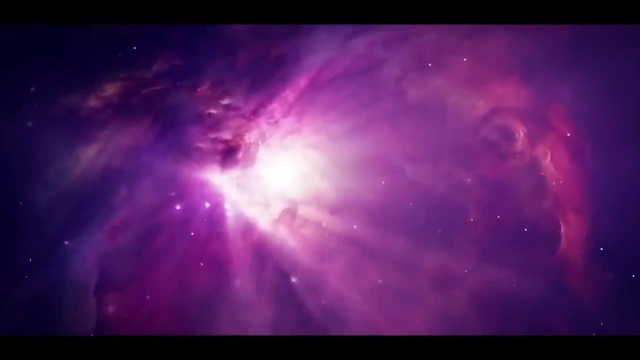 devices, we cannot see the area that is the last scattering of the universe, that is located beyond the surface of the last scattering, because it is opaque. after all, it is light that allows us to see distant objects and judge their properties by one means or another, regardless of the fact that it is 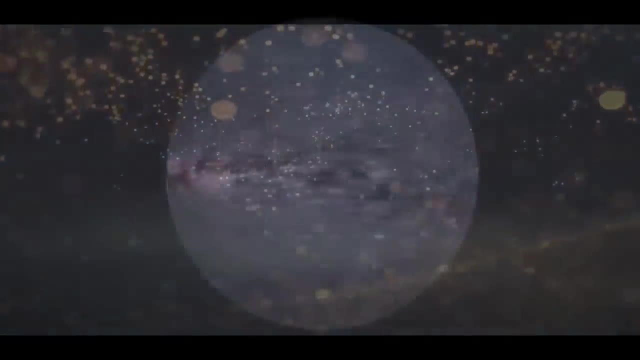 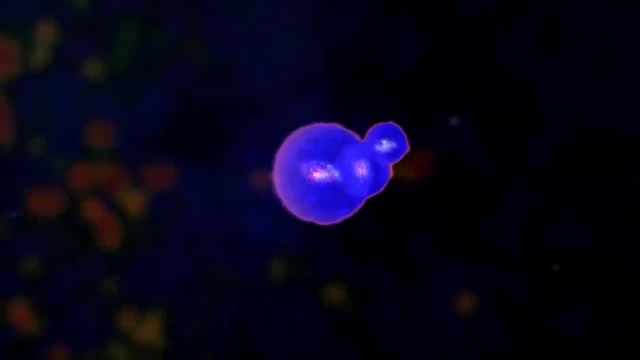 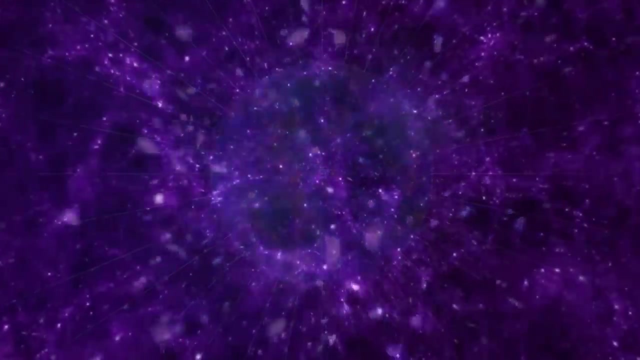 impossible to see what is happening beyond the last scattering surface. researchers are able to form an opinion about the expanse beyond it. to do this, they observe what effect it has an existing astrophysical objects. more than that, according to the latest data, galaxies are moving away from each other. 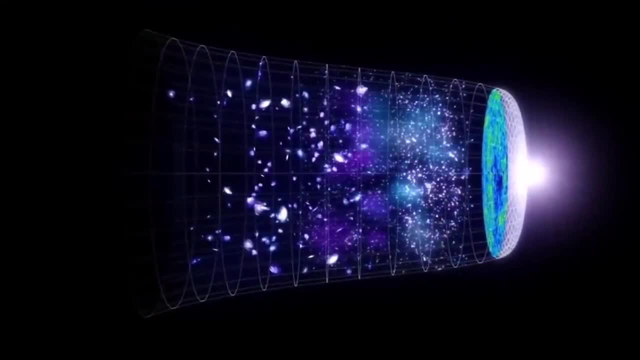 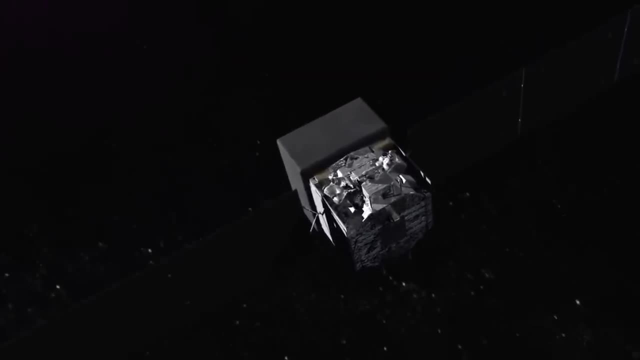 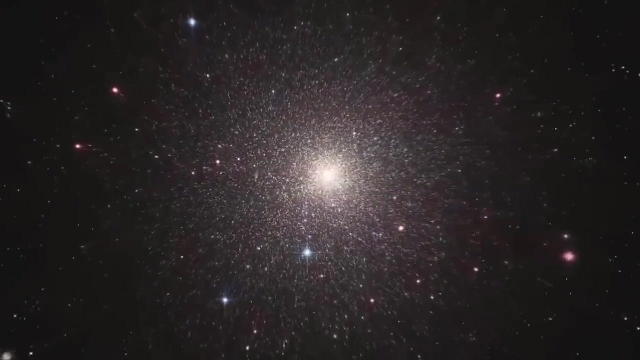 at an accelerated pace, and the further away the galaxy is, the faster it is moving away from us. this means that at some point, the speed of the separating galaxies will exceed the speed of light and we will no longer see them. these objects will go beyond the horizon, but will not disappear. this fact implies that 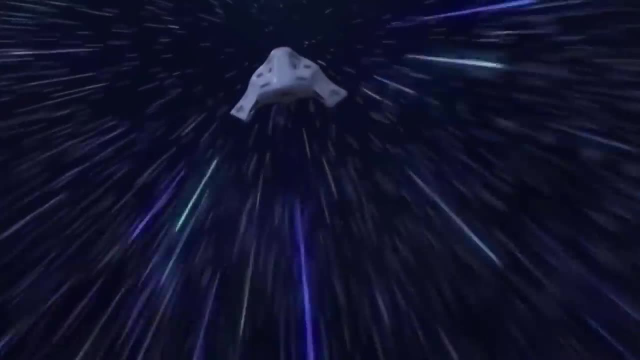 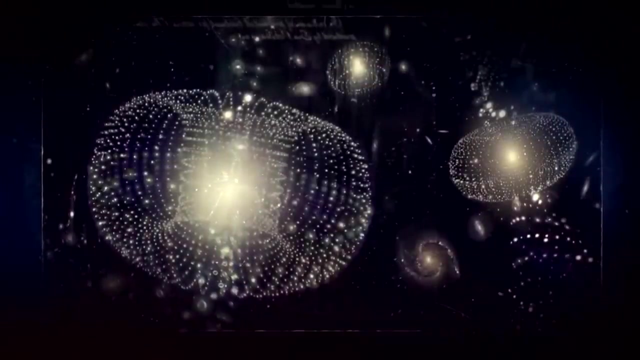 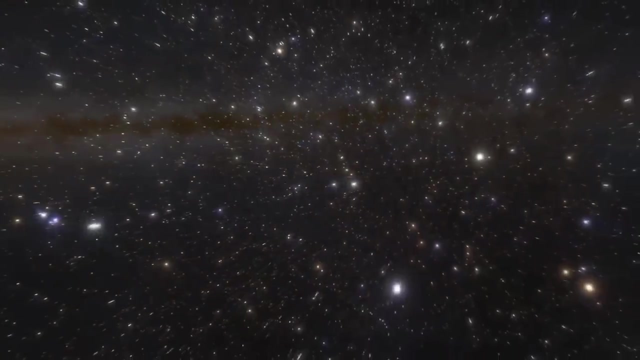 perhaps out there beyond the horizon, we will not be able to see these objects. beyond the observable universe lies an additional vast expanse that is hidden from us by the barrier of the speed of light, the point being that CMB maps made with telescopes, such as those of NASA's WMAP and the ESA's Planck, showed on a 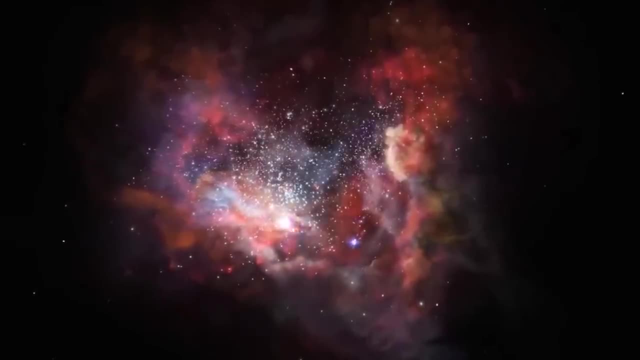 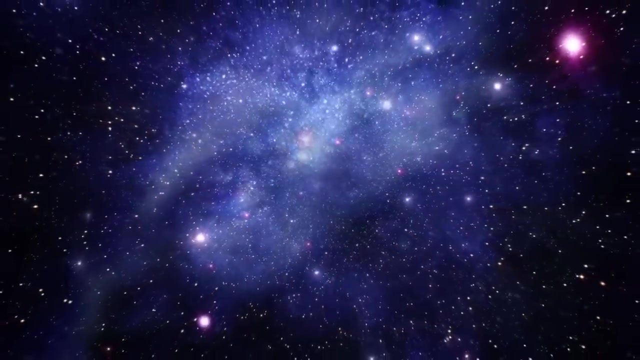 vast scale, a mystifying lack of perturbations. this jaunty little word means the departure of a celestial body from an orbit because of the influences of forces other than the gravitational attraction of the center of mass of the system, such as other celestial bodies or 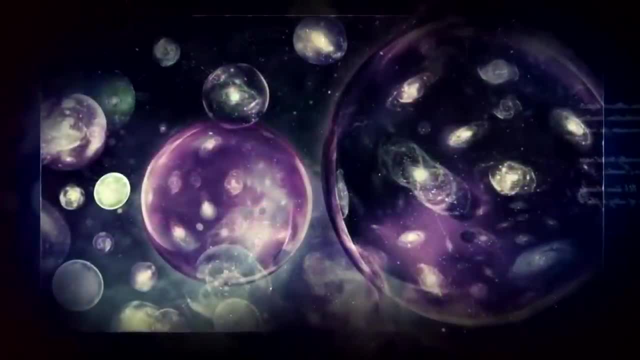 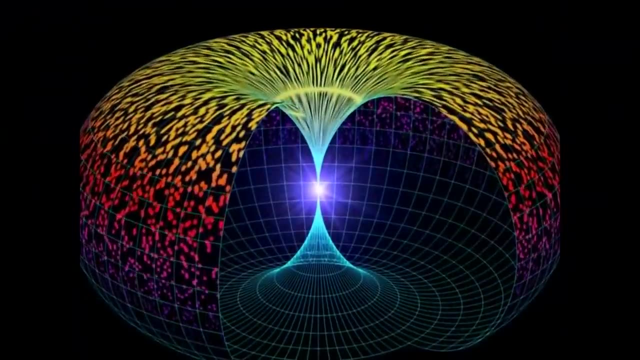 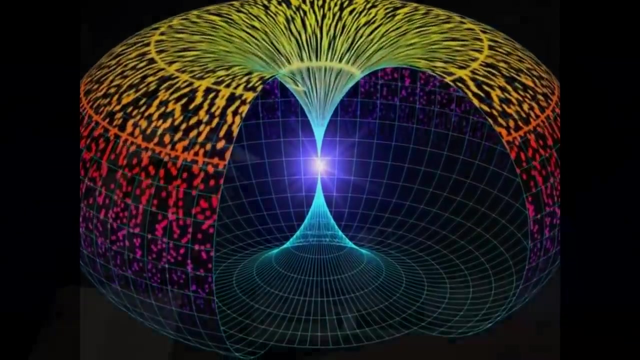 environmental resistance. in order to find out if these missing perturbations could be caused by a multiply connected universe, scientists made many computer simulations of what the cosmic microwave background radiation would look like if the universe had the form of a giant three-dimensional donut, where it is. 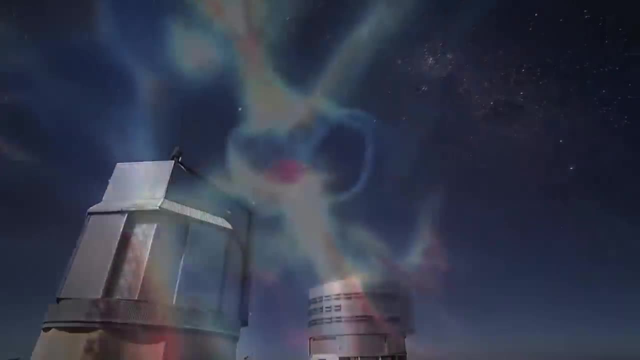 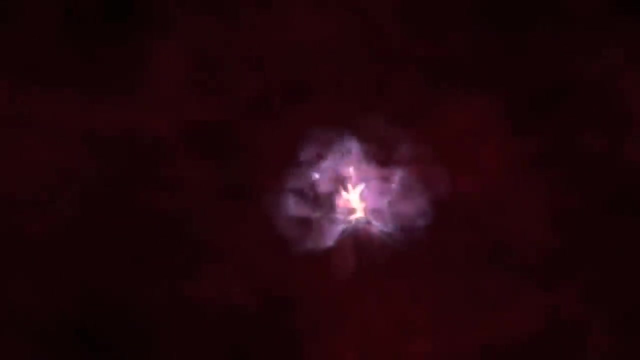 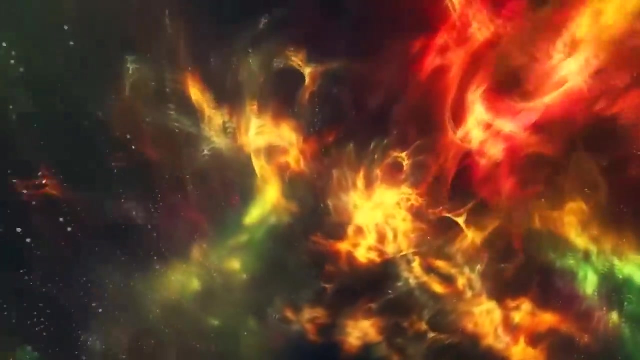 connected to itself in all three dimensions. the properties of the observed fluctuations, such as the deviation from the mean value of a random magnitude characterizing a system of a large number of chaotically interacting particles of the cosmic microwave background radiation, show insufficient power on a scale exceeding the size of the universe. this lack 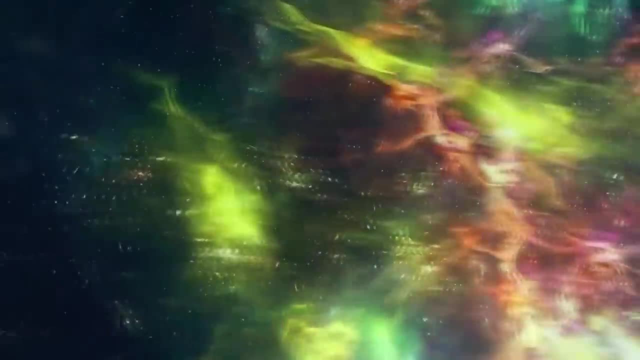 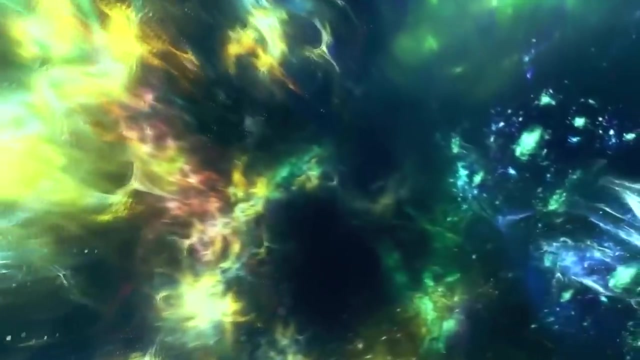 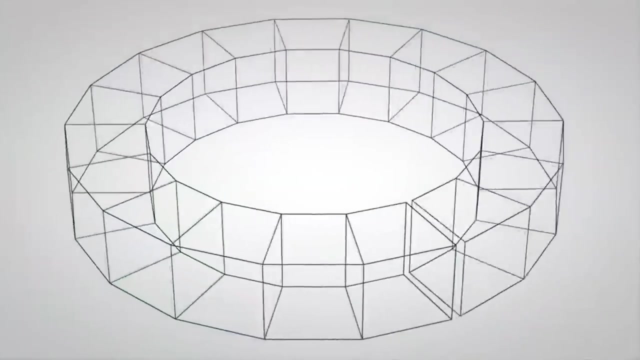 of power means that fluctuations in the cosmic microwave background radiation are not present on such scales and that our universe is multiply connected and finite. in other words, it looks like the cosmic microwave background is missing signals which must be present if the universe were truly infinite. one explanation for this suggests that the topology 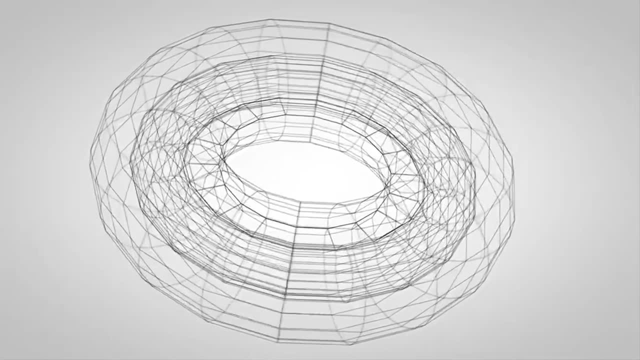 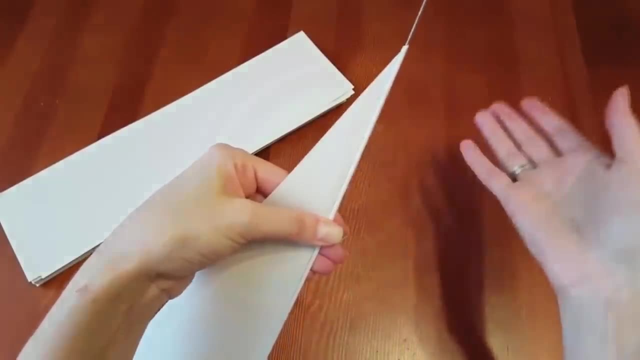 of the universe is curved in such a way that it connects back to itself like a donut or a bagel of intergalactic dimensions. just as you can roll a sheet of paper into a tube without changing its parallel properties, the universe can be donut shaped while remaining flat. 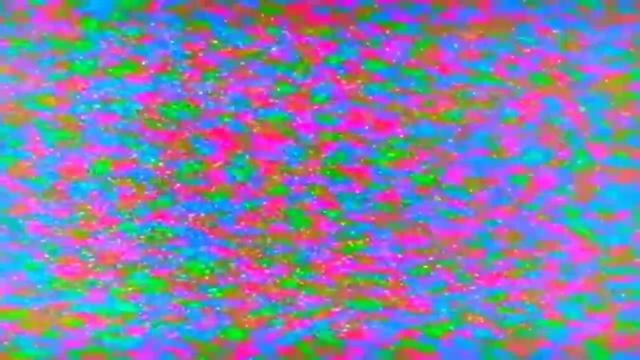 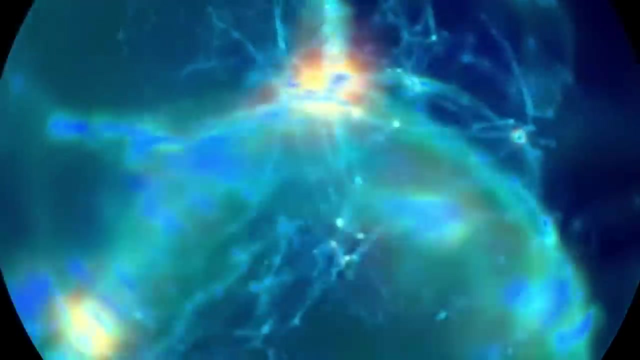 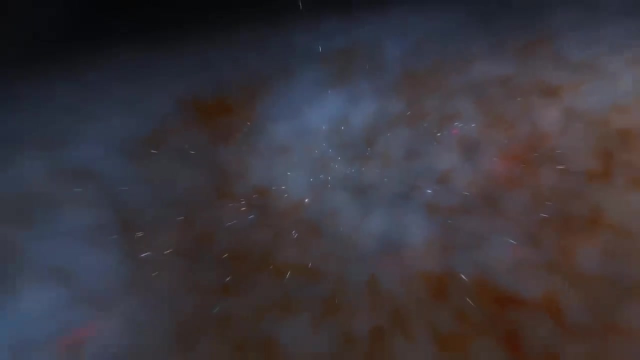 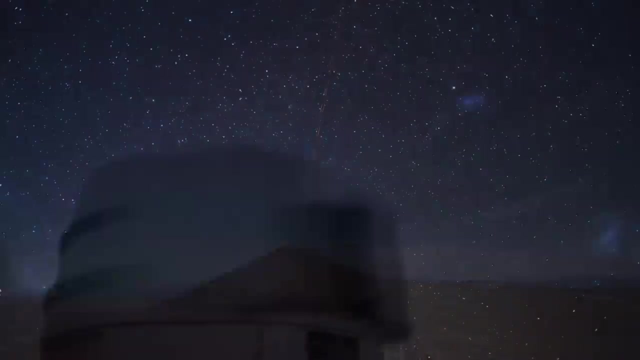 this is exactly what the researchers have found out with the aid of simulations of the cosmic microwave background. it turns out that, compared to the standard cosmological model, which is considered infinite, we found a much better matching observation of the fluctuations. such a universe must have an end, and the entirety of the vast expanse is possibly no more than four. 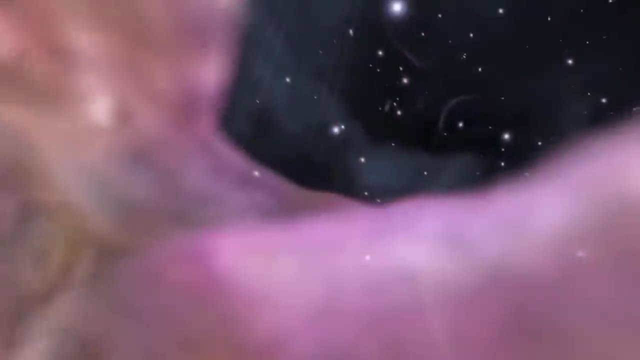 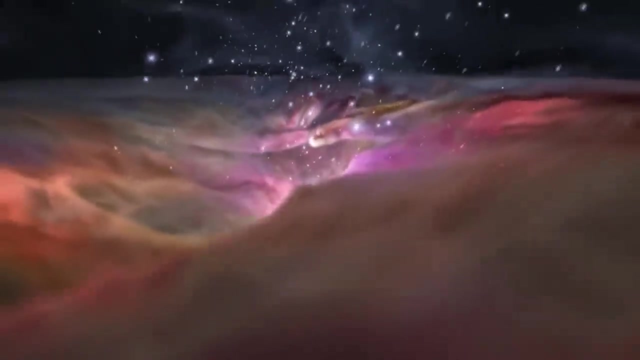 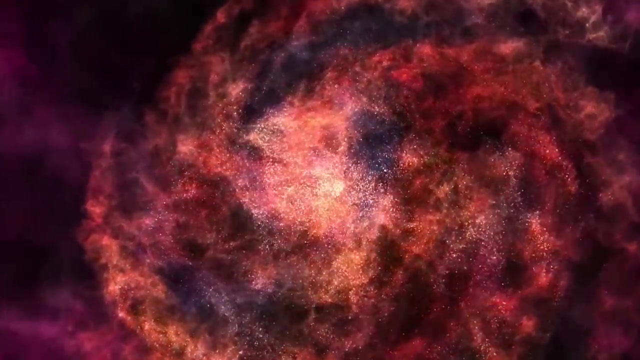 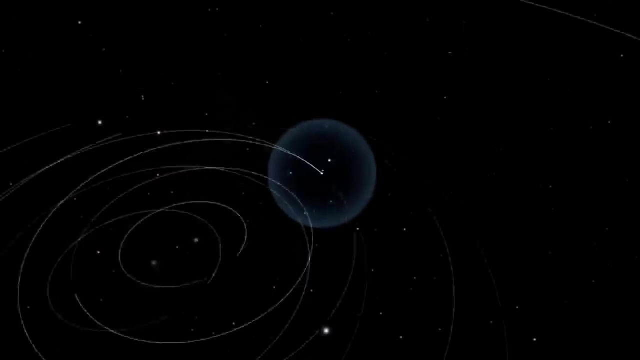 times larger than the boundaries of the universe that is observable by man. the size is 47 billion light years in diameter. the universe can be self-contained in three dimensions and have the shape of a three-dimensional donut. models of the finite universe may be intimidating to some people, but you will not perceive these boundaries for all practical. 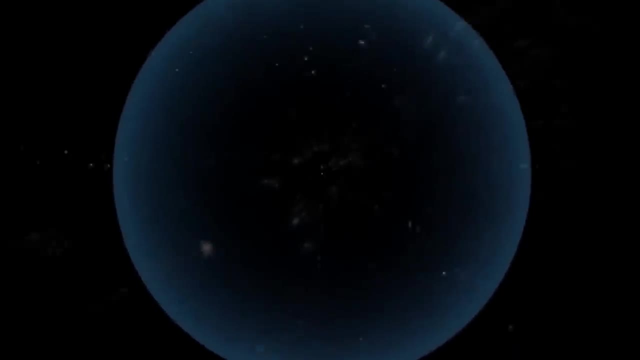 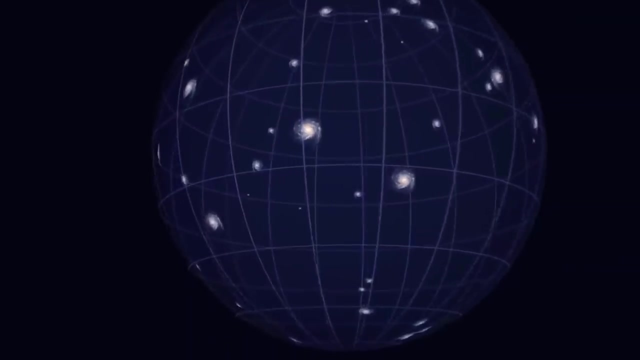 purposes. you simply live in an infinite universe, despite it having finite dimensions. but even if you don't necessarily end up finding yourself at the edge of the universe, you will not be able to get out of this finite universe. would you be able to circumnavigate it and return to where you? 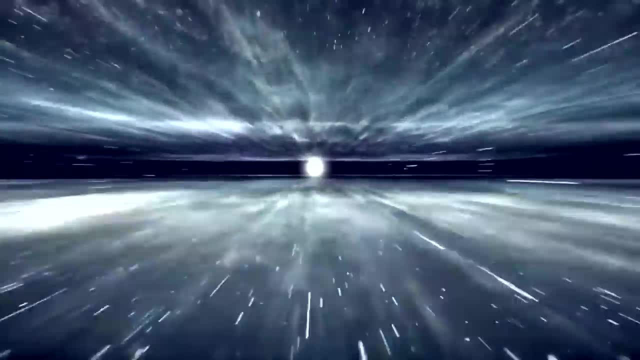 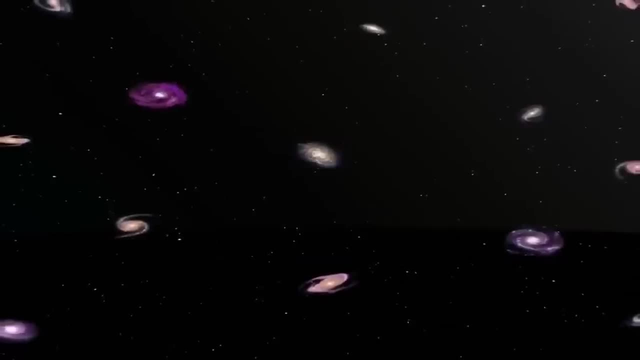 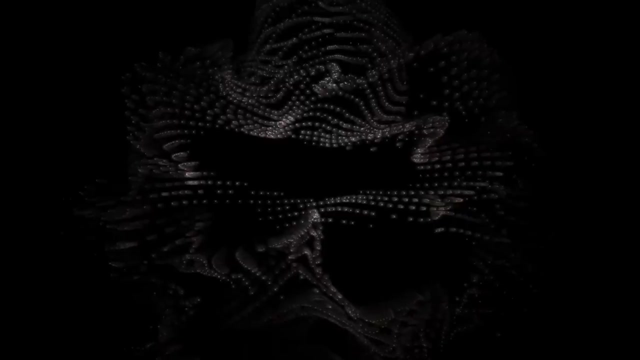 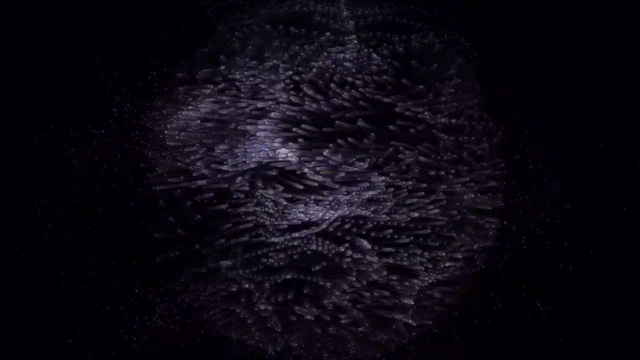 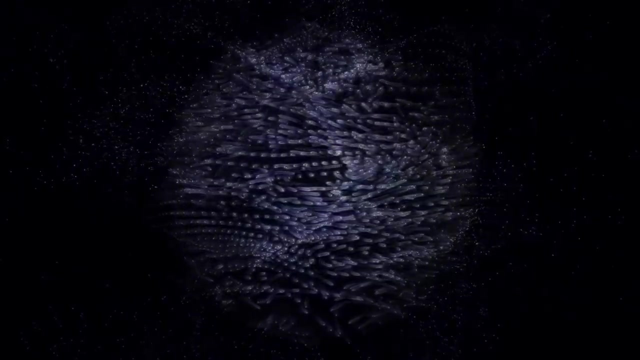 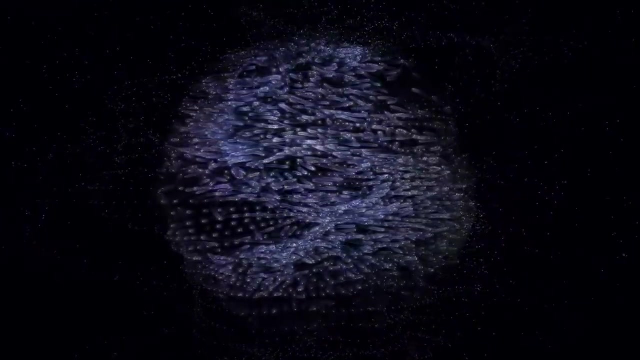 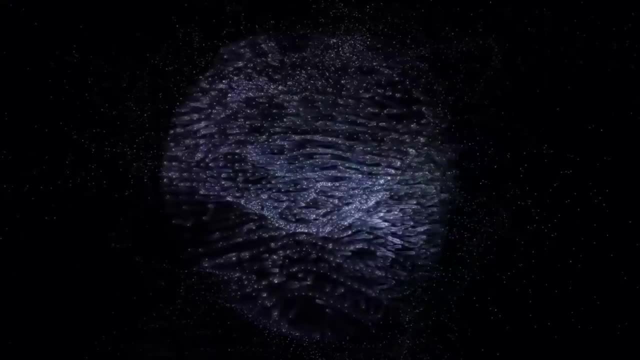 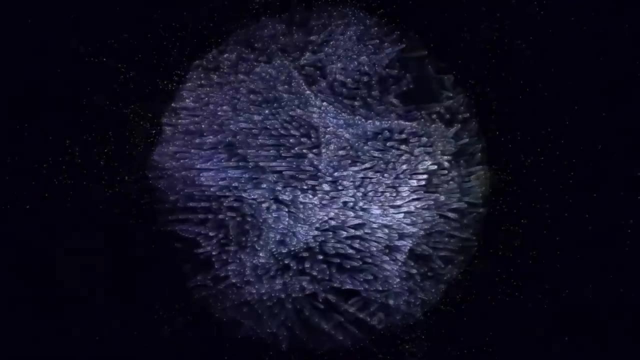 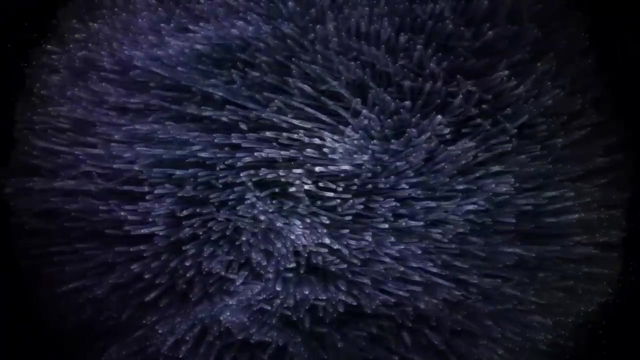 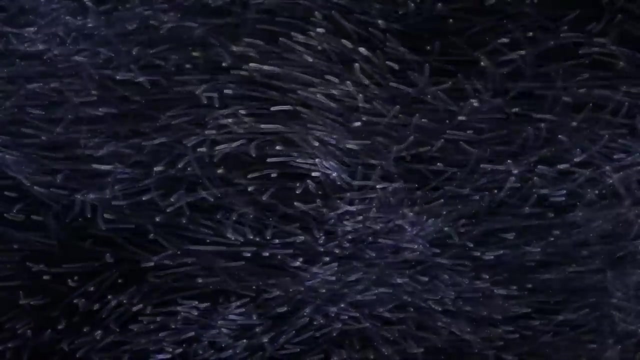 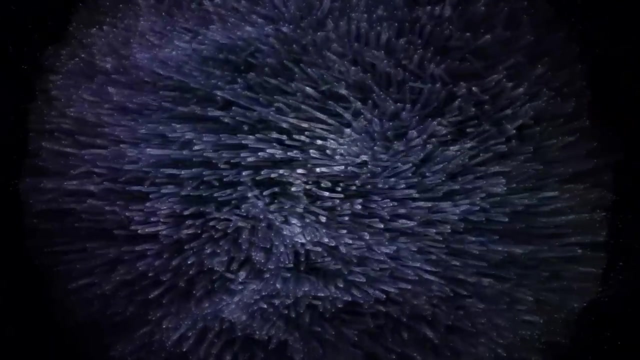 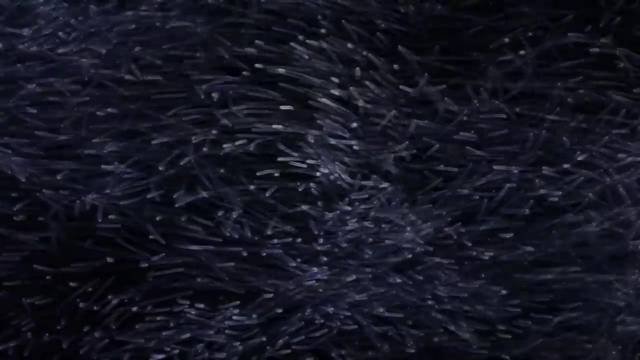 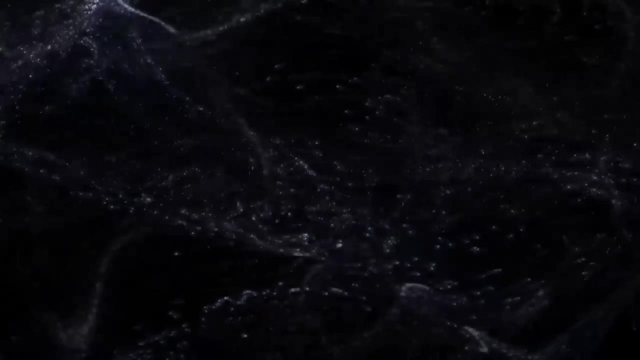 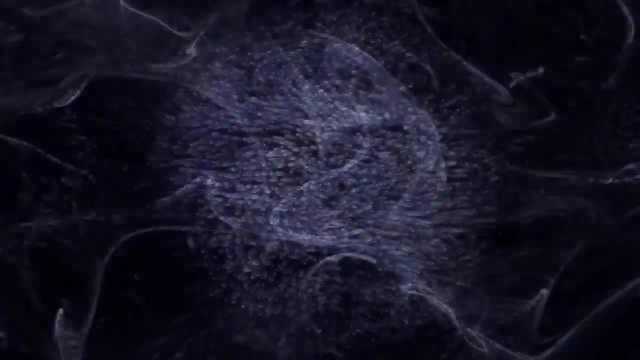 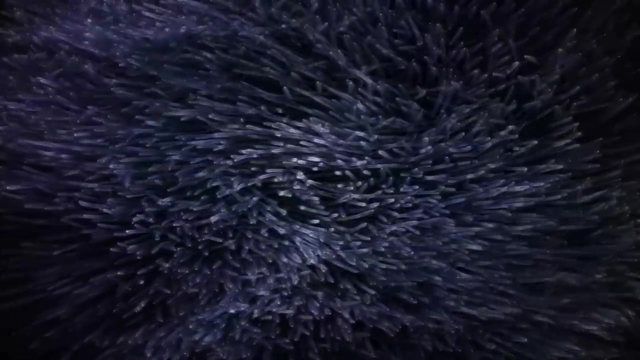 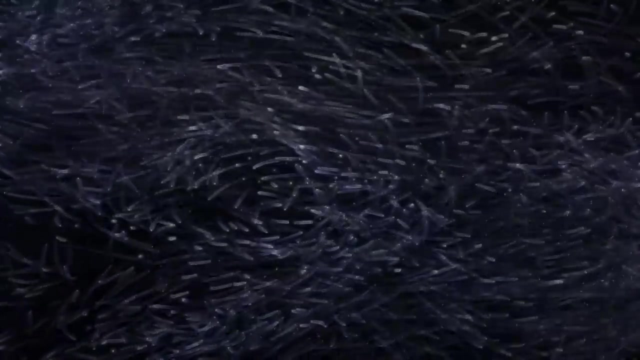 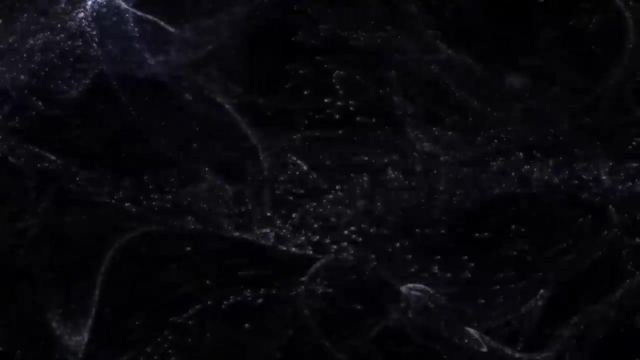 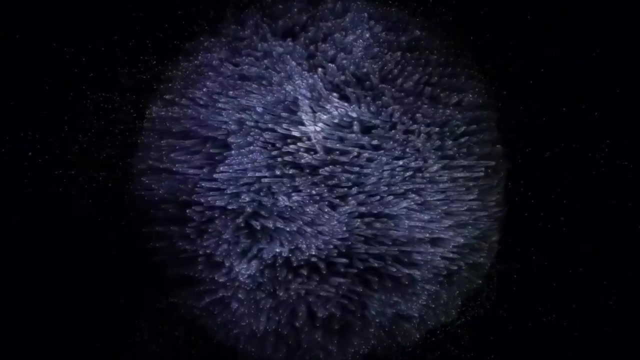 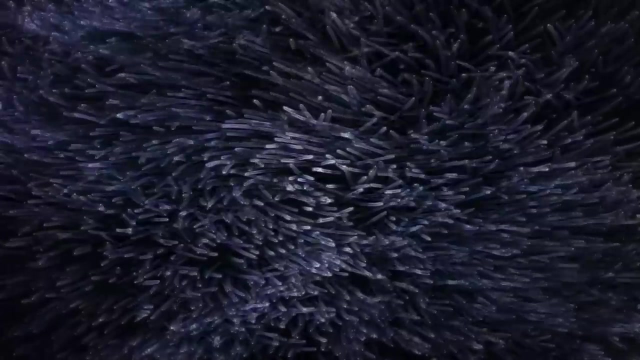 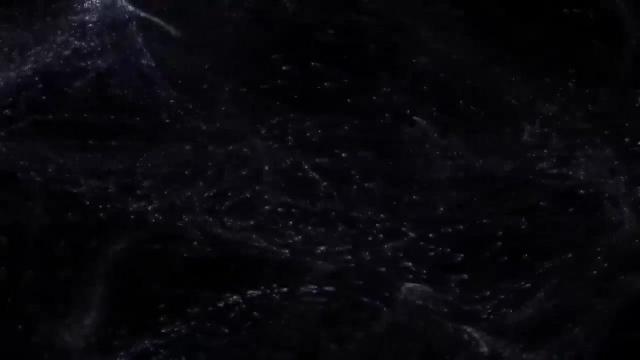 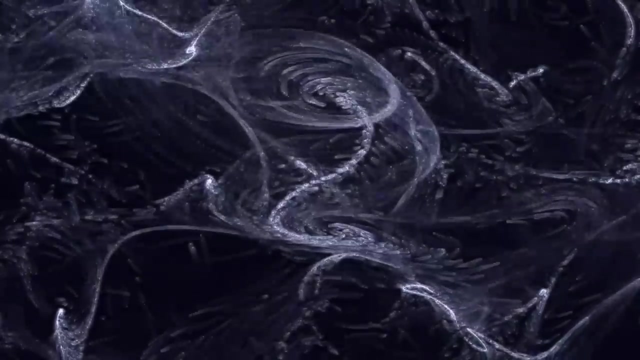 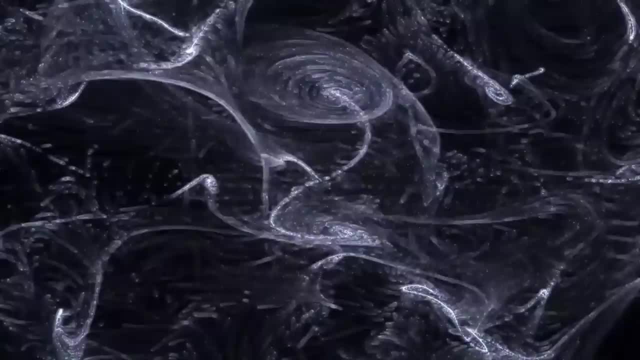 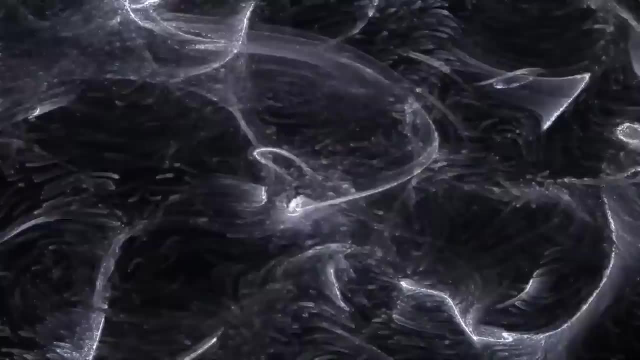 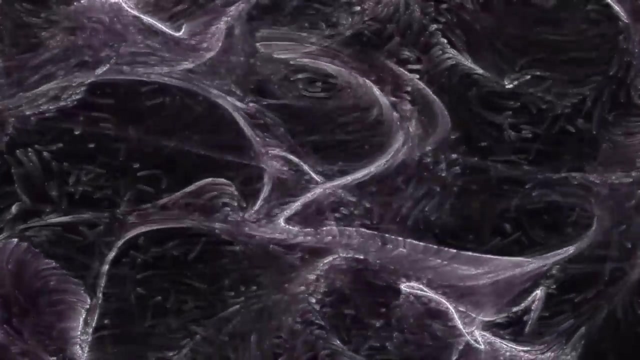 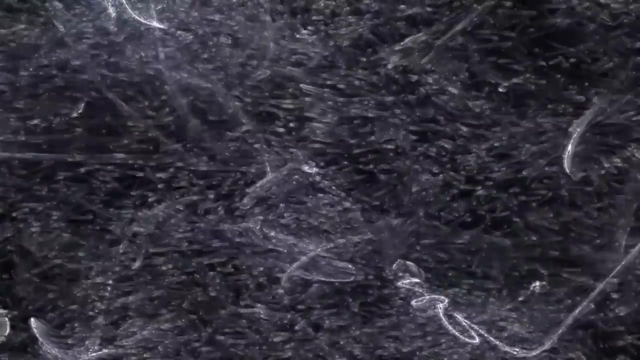 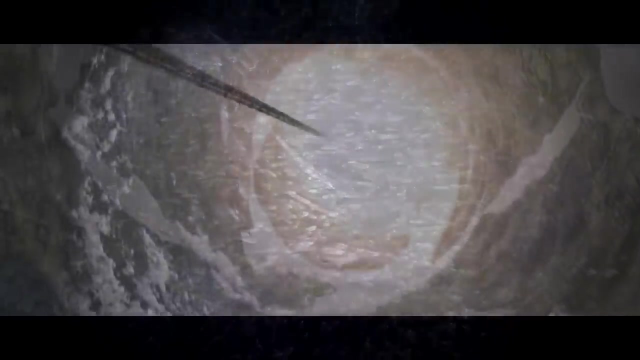 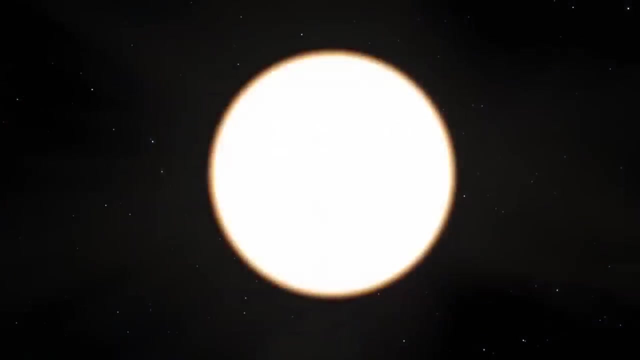 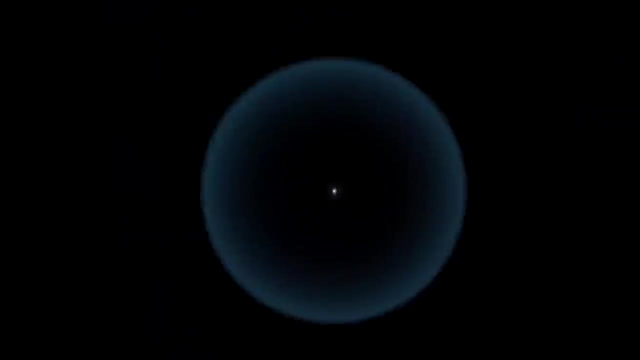 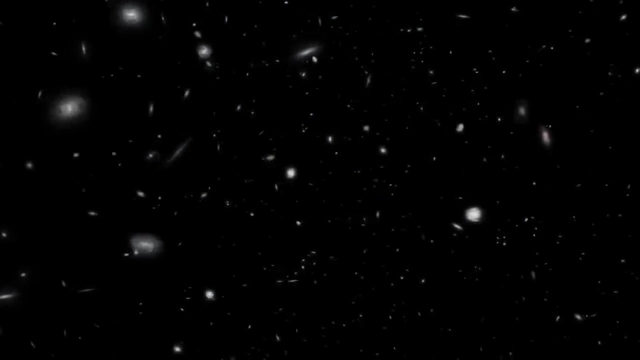 so so so so. lost somewhere in the universe is a small blue planet, the third in order, from a star called the sun, one of the billions of stars in the spiral galaxy, the milky way. but where is the milky way located in the universe? a team of scientists has collected data on more than 8 000 galaxies in the outer. 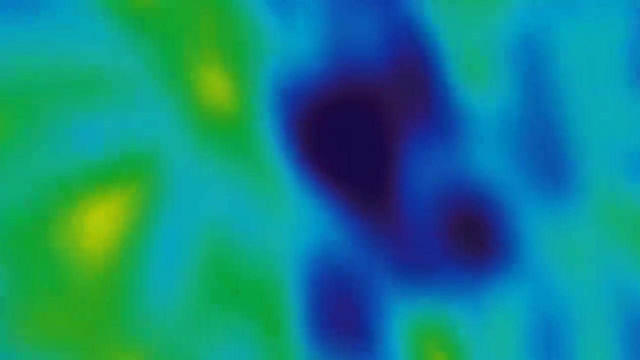 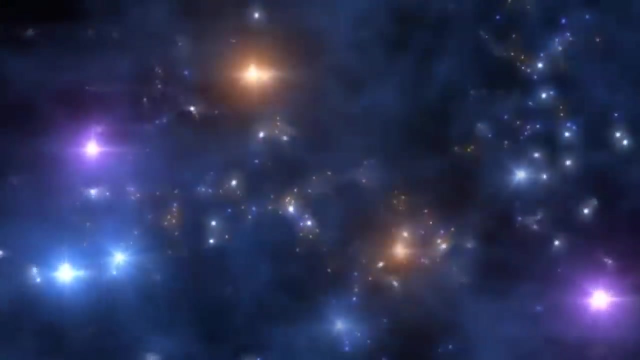 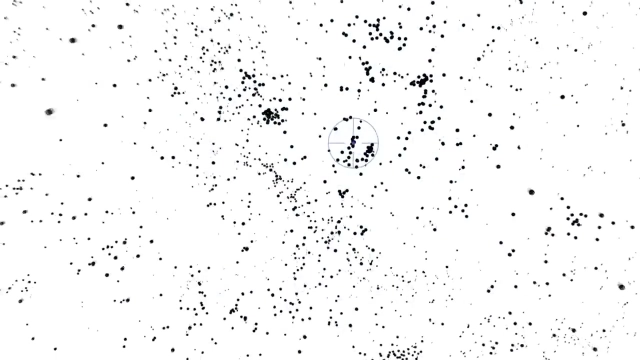 space that surrounds us. they have mapped the positions and speeds of the galaxies and, for the first time in history, we saw that the milky way is part of a much larger system of galaxies, a super cluster which they called laniakea. our galaxy is located in the outer reaches of this cluster. 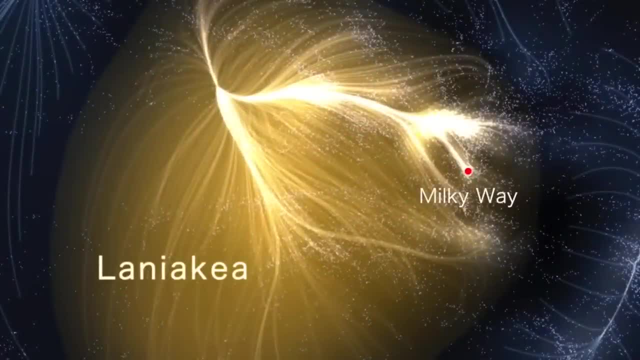 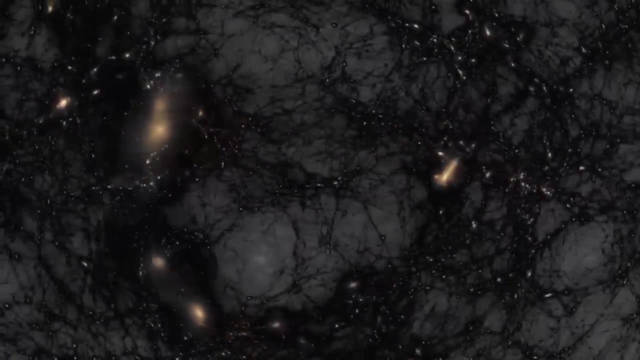 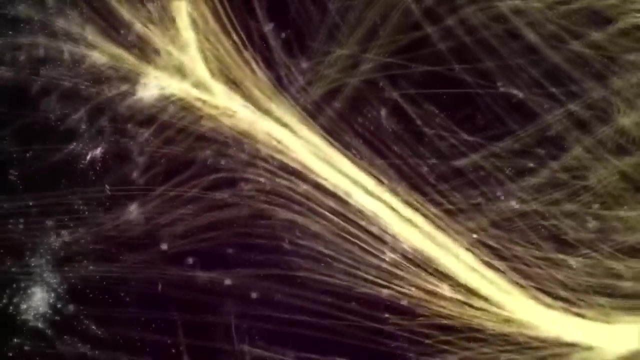 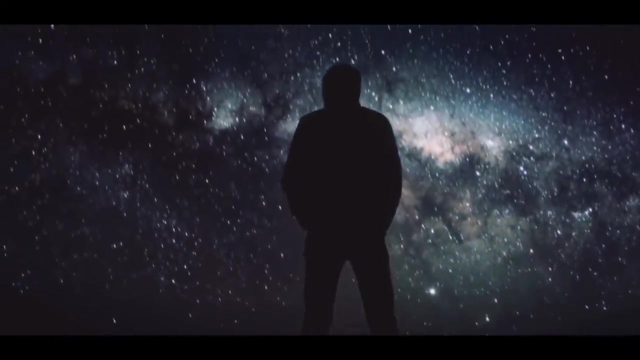 the entire universe is a sinuous network of galaxies, something like a cosmic spider web. some regions are almost empty and look like dark cosmic voids, while others, on the contrary, are densely populated by galaxies in areas that are called super clusters, and these are perhaps the largest structures in the universe that we know. but here's the question. think for a moment where. 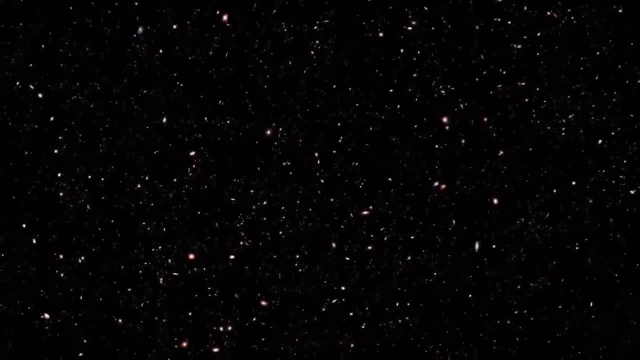 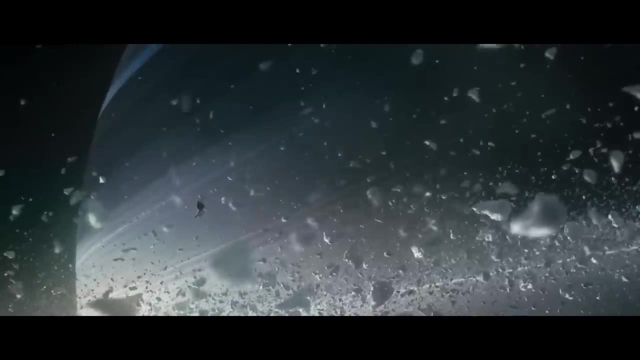 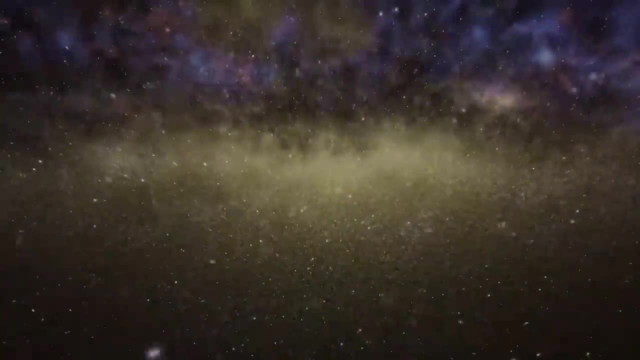 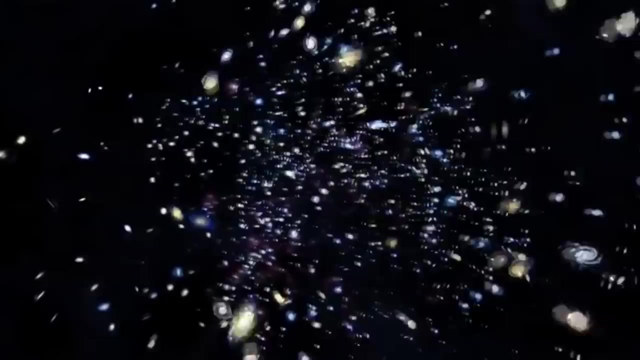 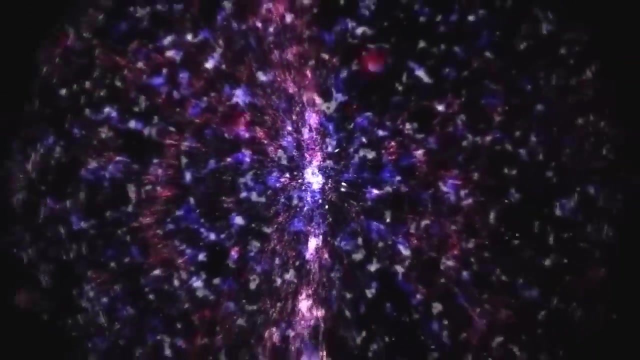 the name, the great attractor. our galaxy, just like neighboring ones, is attracted toward a specific region of space, and it's about 150 million light years away. and here's the surprise: we don't know exactly what's there. however, the name of this mysterious anomaly has already been thought up. 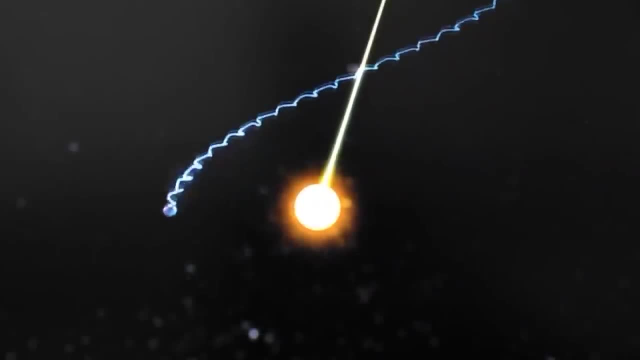 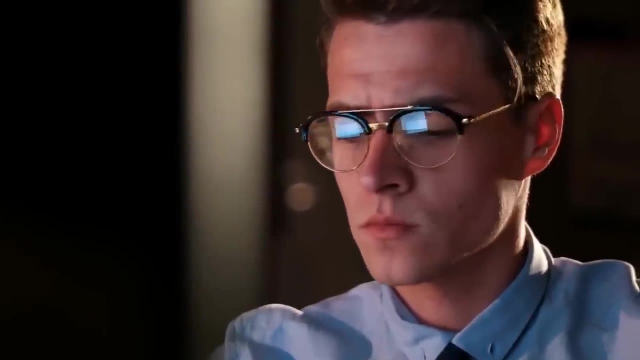 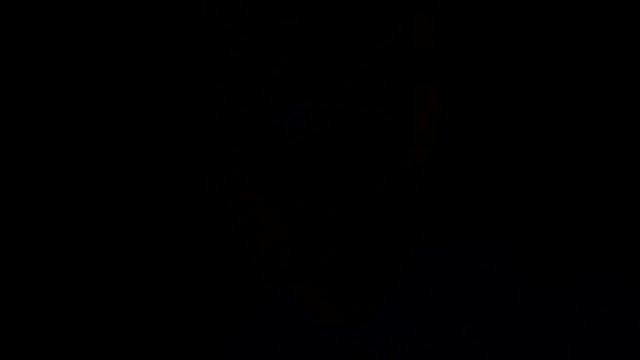 which is a great way off our shoulders. yes, we are talking about the great attractor. in part, it's so mysterious because it's located in a region of the heavens called the zone of avoidance, which is situated toward the center of our galaxy. there is so much gas and dust there. 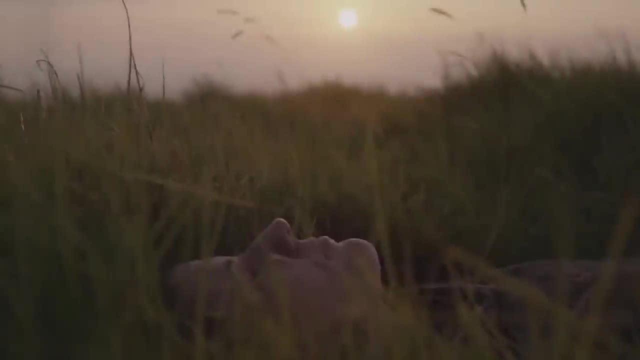 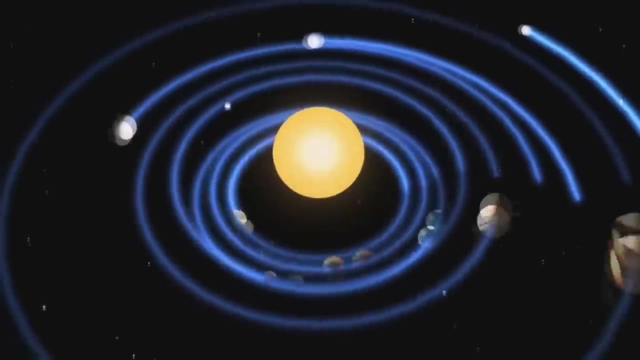 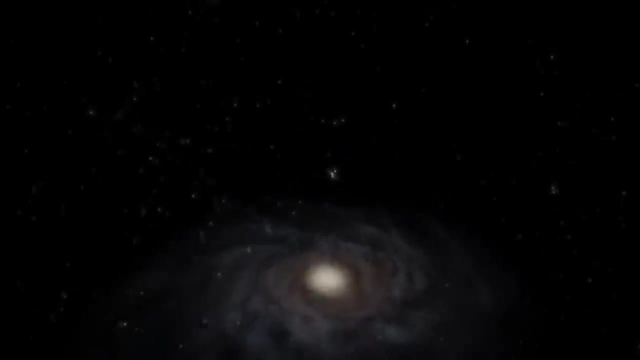 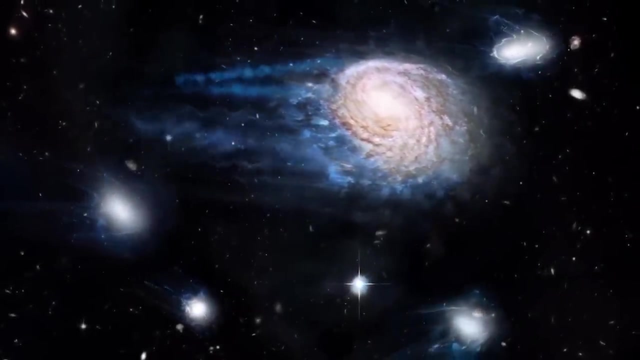 that you can't see very well or far in the visible light spectrum. the solution to the problem was the study of the clusters in the zone of avoidance. to study the hard to reach regions, x-ray radiation was used which easily penetrates clouds of gas and dust. clusters of galaxies are sources of x-rays, which makes observation and study easier. in fact. 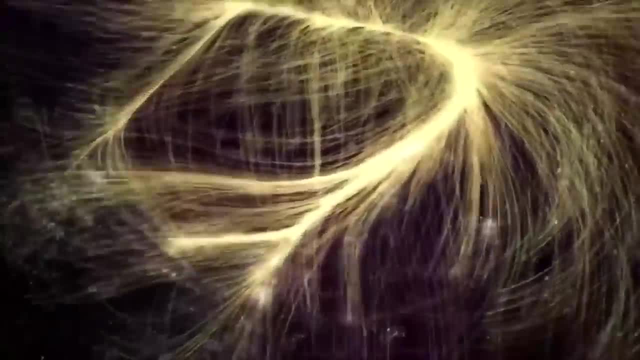 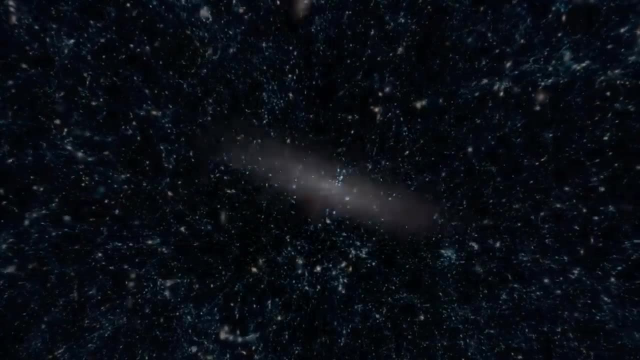 the zone of avoidance is currently quite well researched. galactic gas and dust are also penetrated well by radio waves, as well as light in the infrared range. according to the findings of the study, fewer massive galactic clusters are more likely to be found in the zone of avoidance. 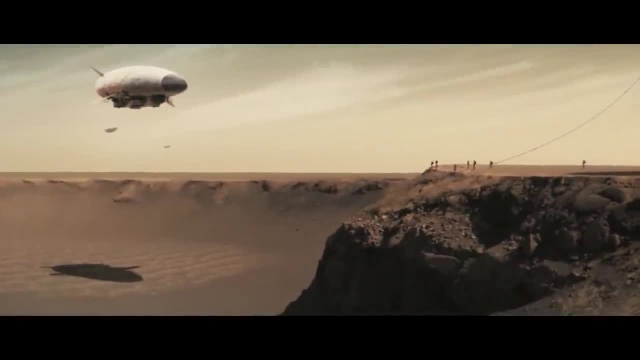 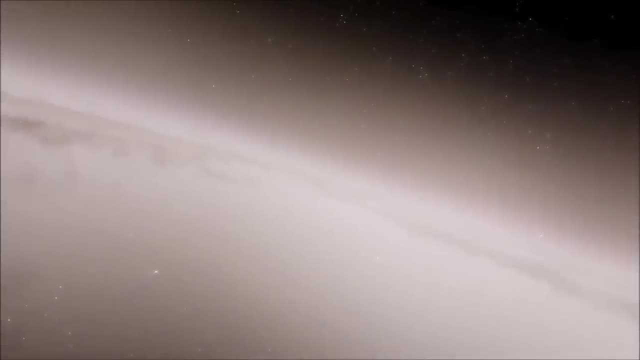 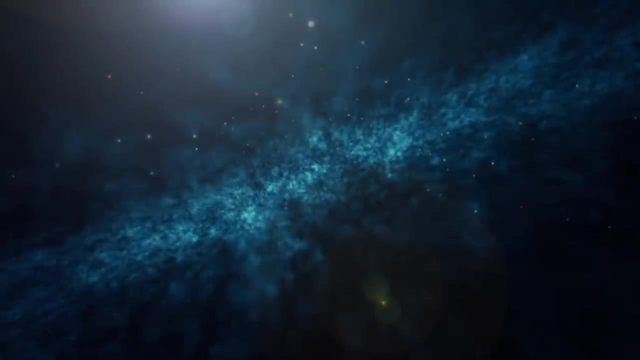 than in the zone of avoidance. in the zone of avoidance. in the zone of avoidance, however, a gravitational anomaly near the center of the great attractor, the abel 3627 cluster, was strong enough to tear apart the spiral galaxy es0137-001 or, as it is also known, the jellyfish. 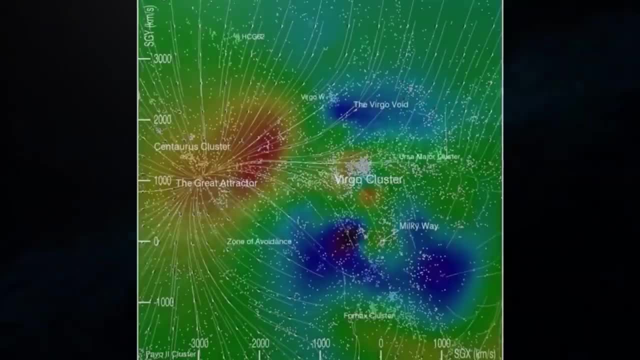 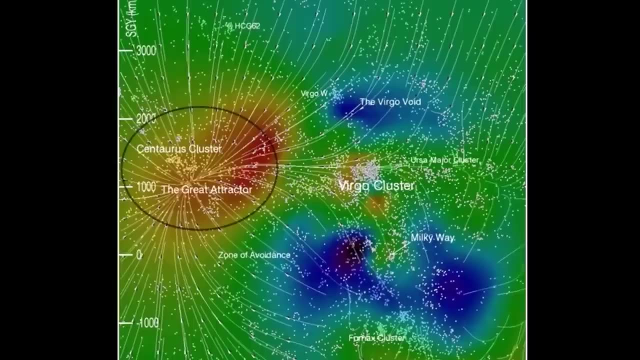 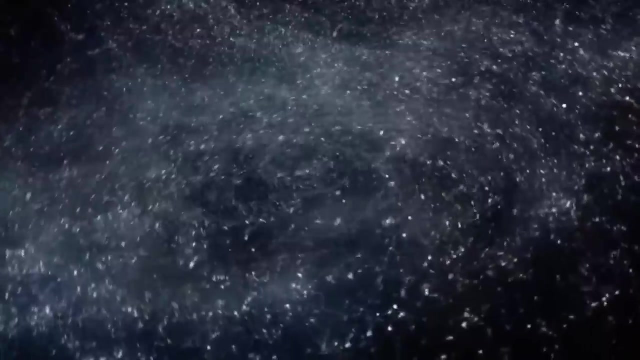 galaxy in the constellation of triangulum australi or the southern triangle as well as the southern triangle, so it is possible to make a study of the zone of avoidance in greater detail. it turned out that at the location of the great attractor there is a large super cluster of 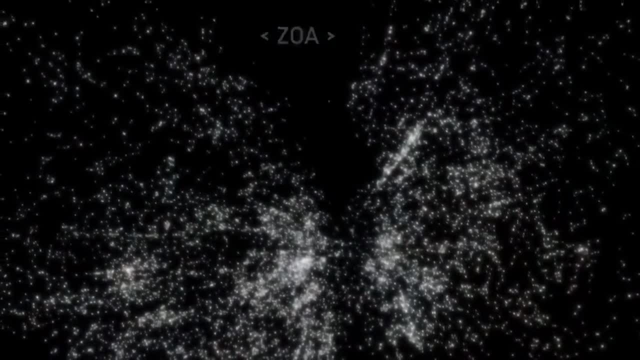 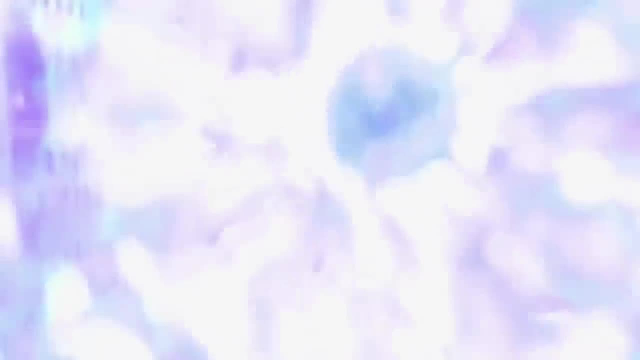 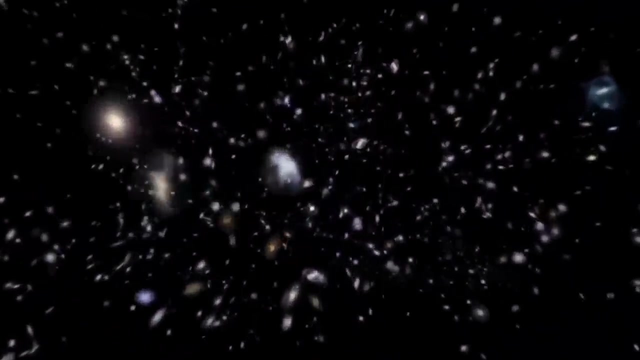 galaxies, called the norma cluster. its mass is about 1 000 trillion times the mass of the sun. it consists of thousands of galaxies and although the norma cluster is massive and the local groups galaxies are attracted to it, it is impossible for them to fully explain the movement of the. 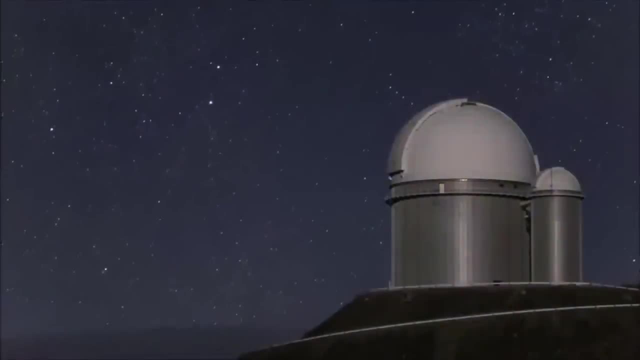 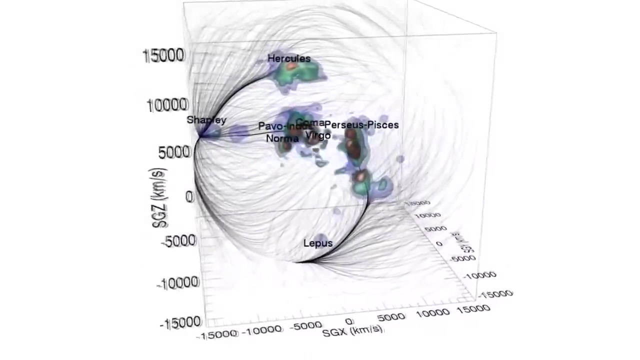 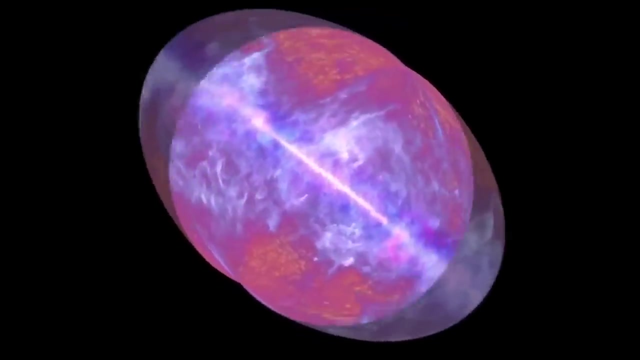 local groups, galaxies. mass of the great attractor is not enough to generate such attraction. a study was conducted which made it possible to calculate that the great attractor contributes only 44 percent of the speed of the movement of the local group, with the rest being associated. 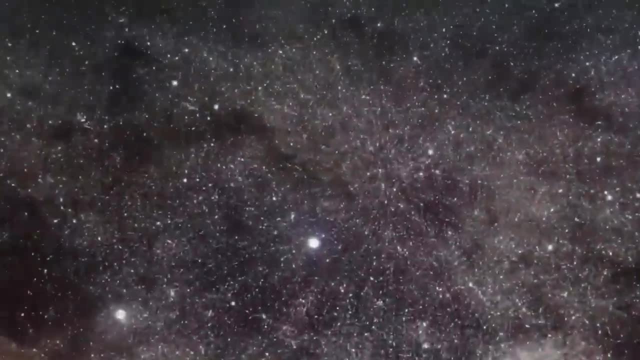 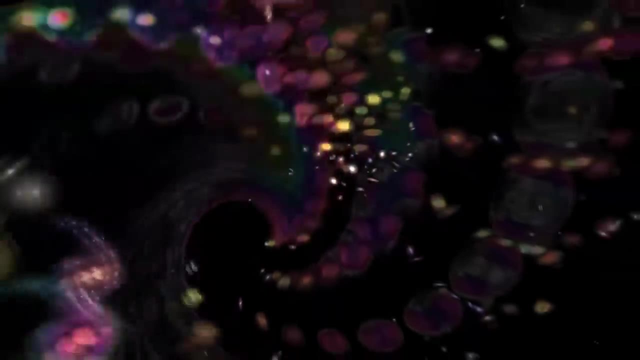 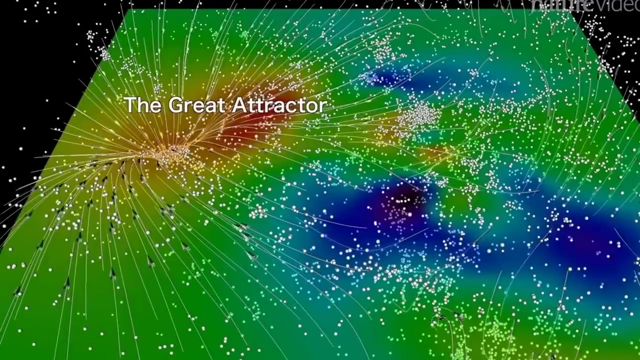 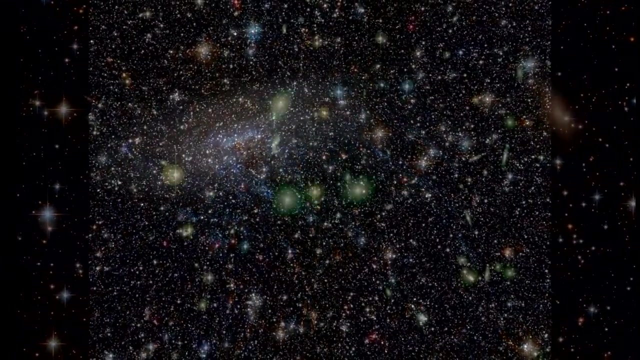 with the dark flow, where a significant region of the local universe, including even the great attractor itself, is moving in the direction of another object. continuing the research, astronomers at the university of hawaii have discovered an even more massive cluster of galaxies at a distance of more than 600 million light years from the milky way, far beyond the great attractor. this 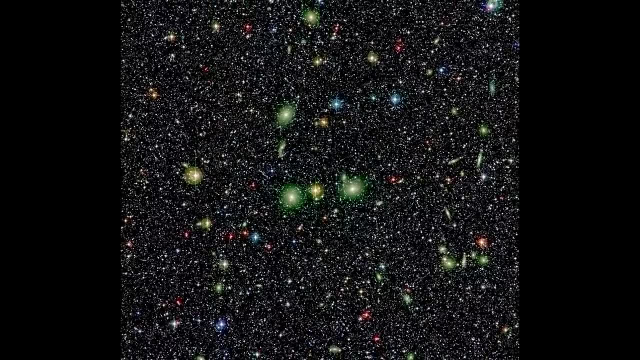 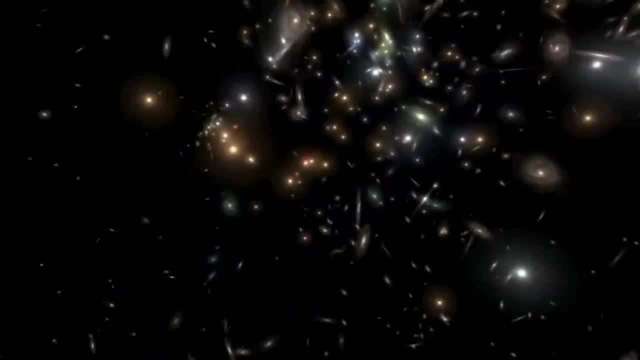 refers to the shapely supercluster in which there are more than 8 000 galaxies and it has a mass of more than 10 million billion suns, which is 10 times greater than the normal cluster in the region of the great attractor. out of the 220 million suns in the region of the great attractor. 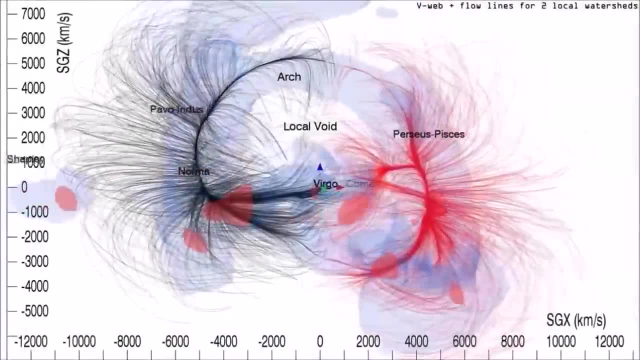 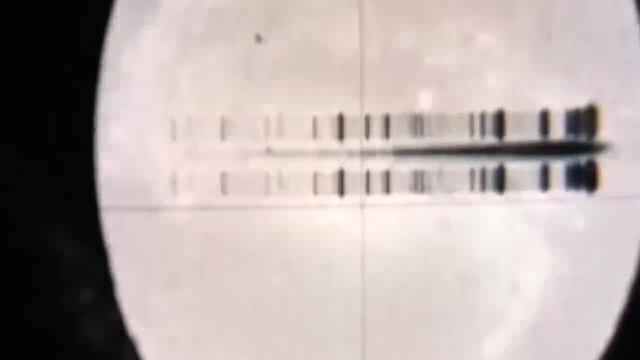 out of the 220 million suns, there is a one of two completely known super clusters of galaxies in the observable universe. the shapely super cluster is the most massive and most likely having reached the region of the great attractor, the milky way, as a part of the complete local group. 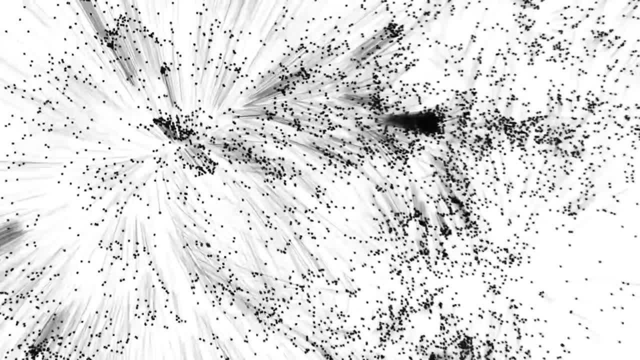 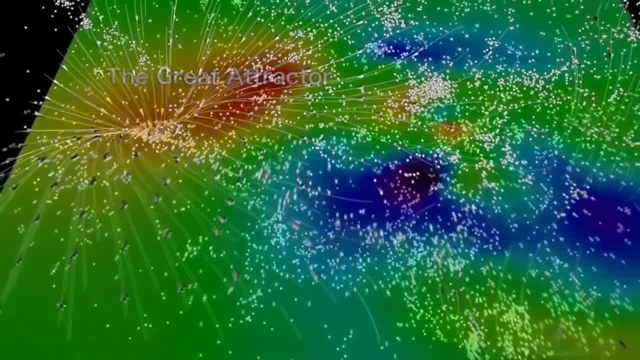 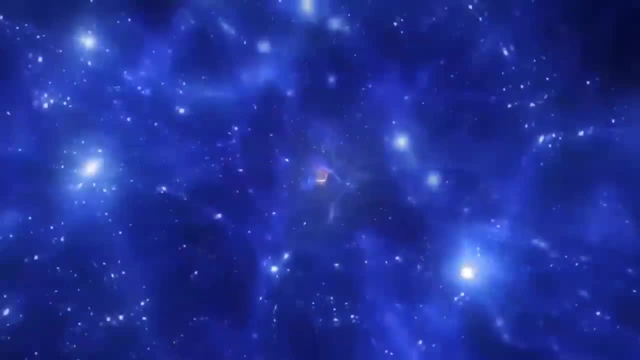 will continue moving on further to the larger object, namely the shapely super cluster. as usual, the logical questions then arise. what will happen to the earth? what awaits humanity, humanity? no one really knows what this could mean, or even if our planet is in danger. astronomers say they will need a few additional years to learn more about this anomaly. 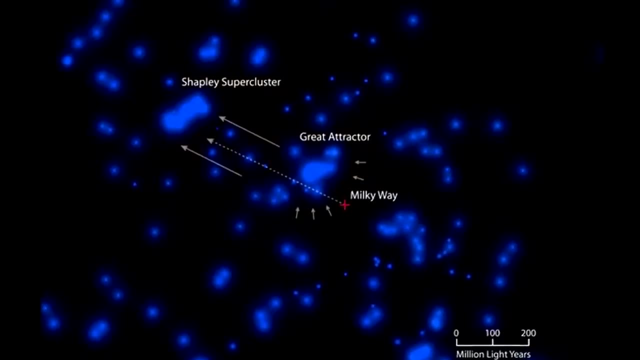 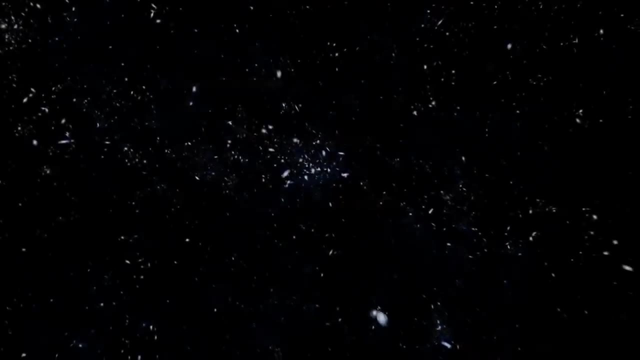 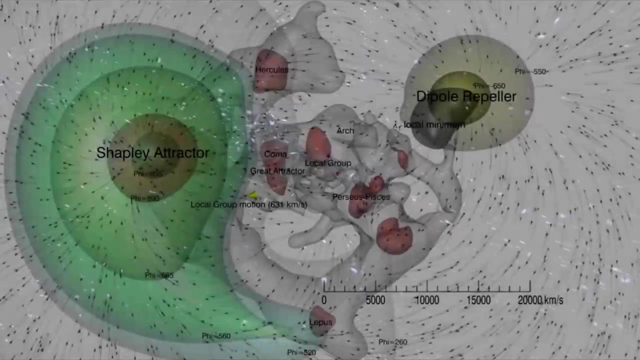 some specialists do not consider it a threat, while others insist that all galaxies and clusters will merge into larger and even larger super clusters. and that's how the universe will come to its logical end, the big crunch which theoretically may well result following the expansion after the big 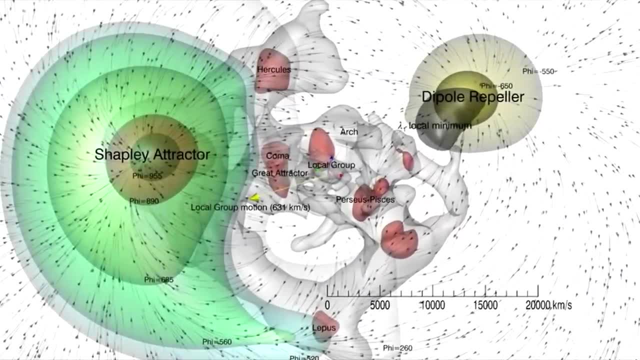 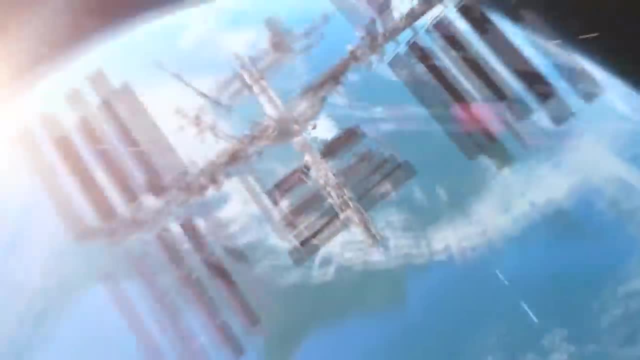 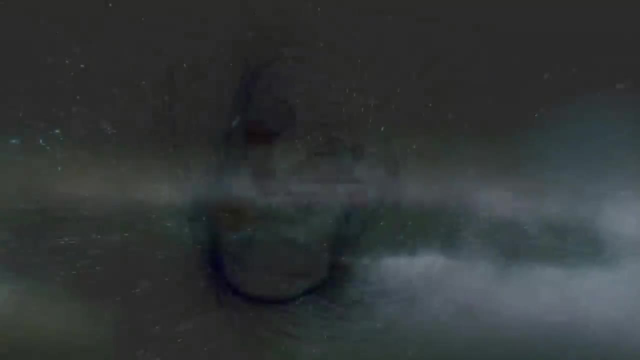 bang. by and large, we have been able to distinguish that the great attractor is a gravitational anomaly located in intergalactic space. in fact, it is a collection of many galaxies formed and hidden away far off in the distance, and a large mass consequently causes the stronger attraction. 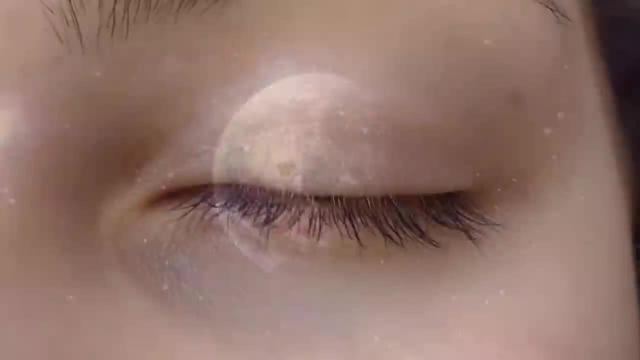 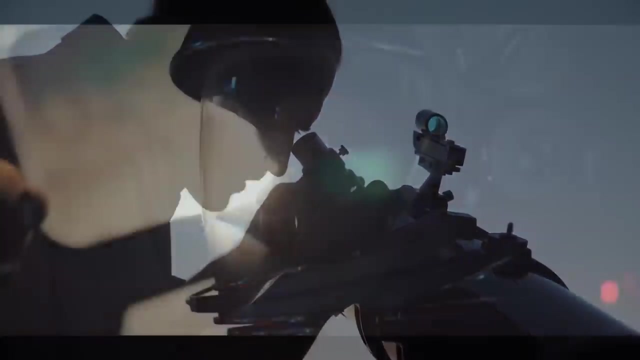 of other objects to include you and i. what do you think of the great attractor and what sort of hopes do you have that we will discuss in the next episode. we will discover something new in this region of space into which our little blue planet is moving so swiftly. 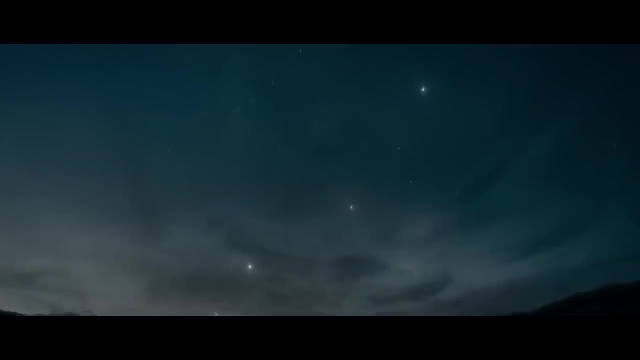 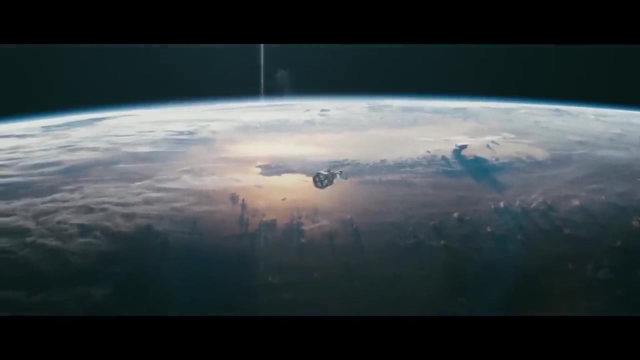 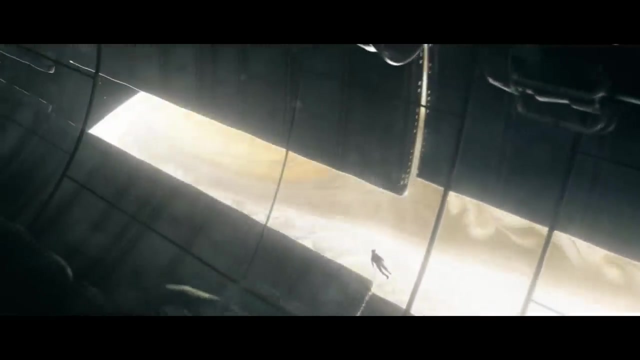 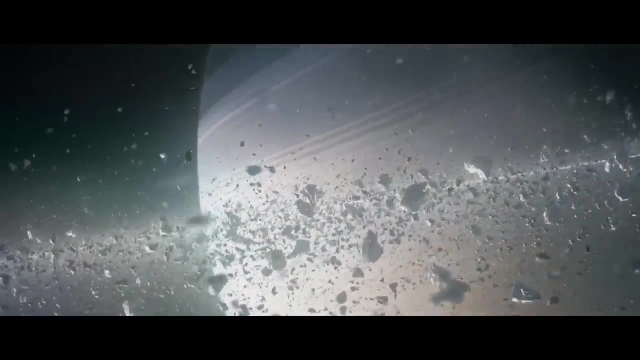 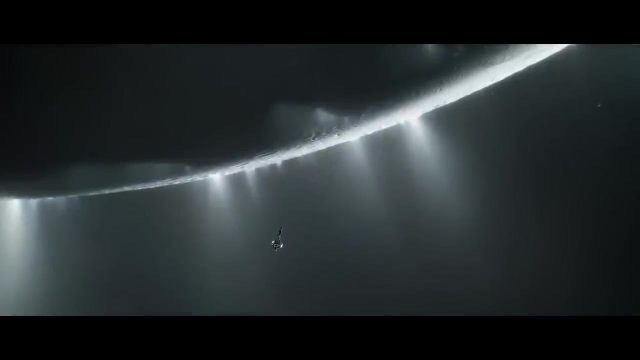 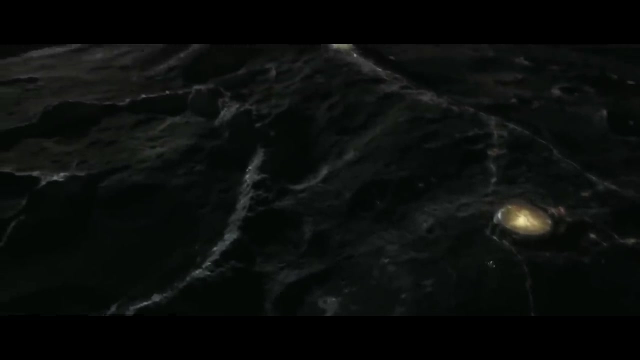 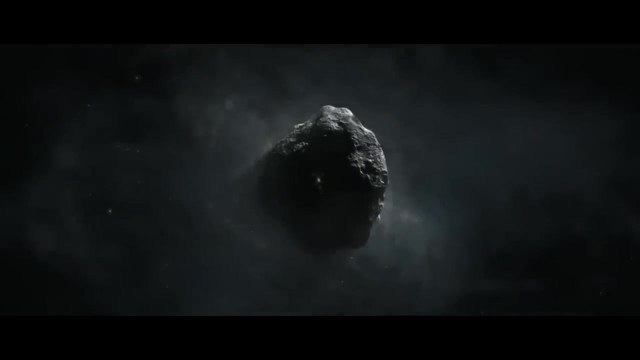 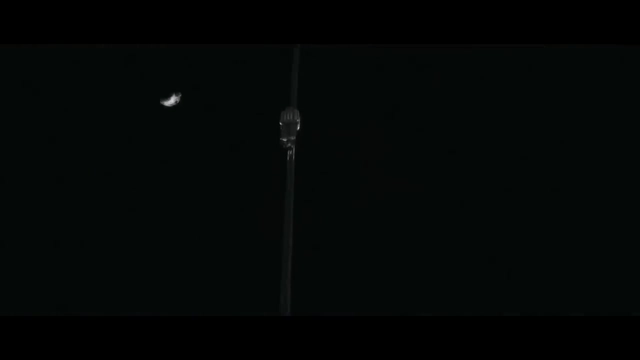 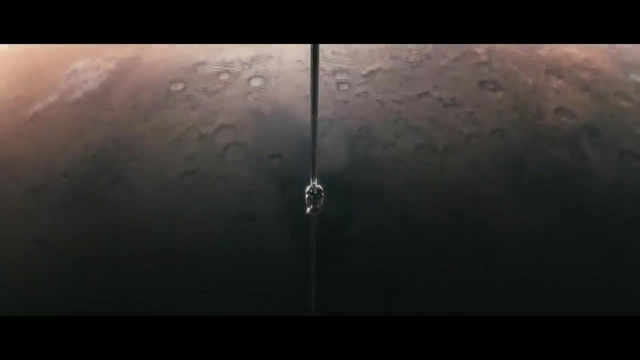 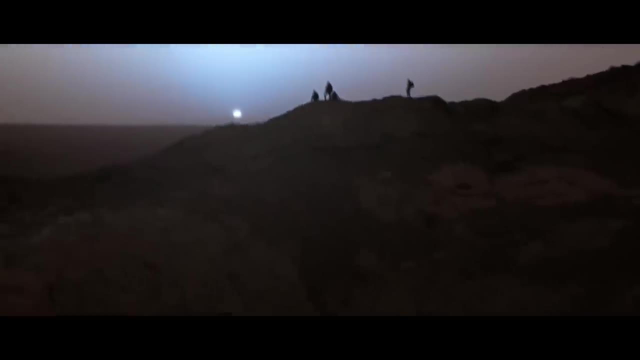 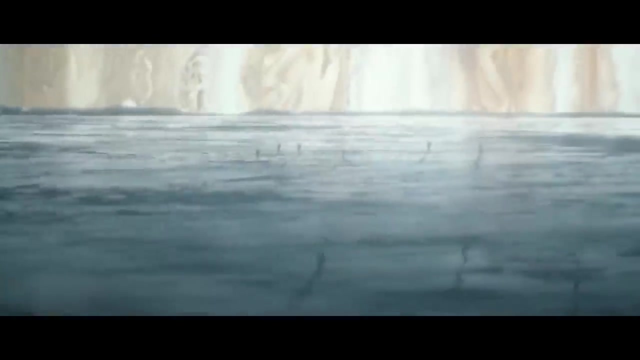 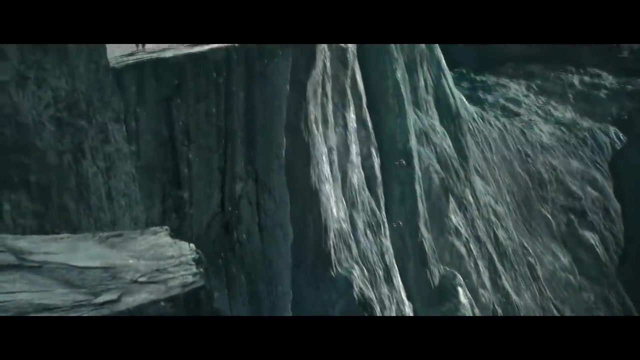 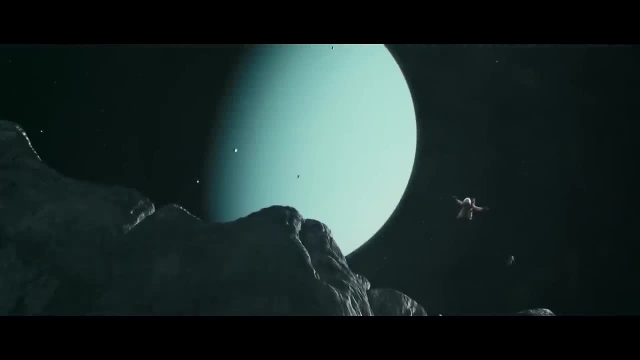 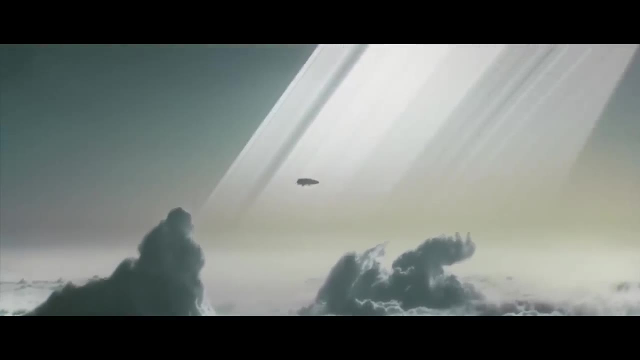 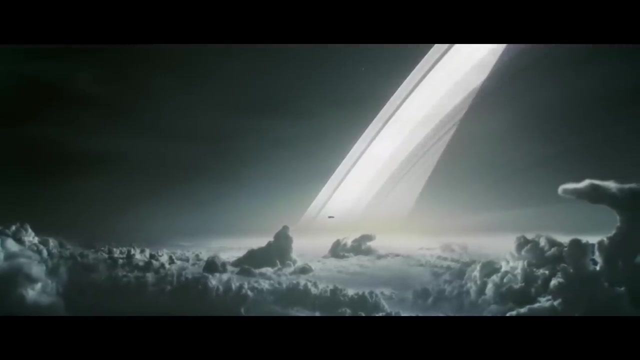 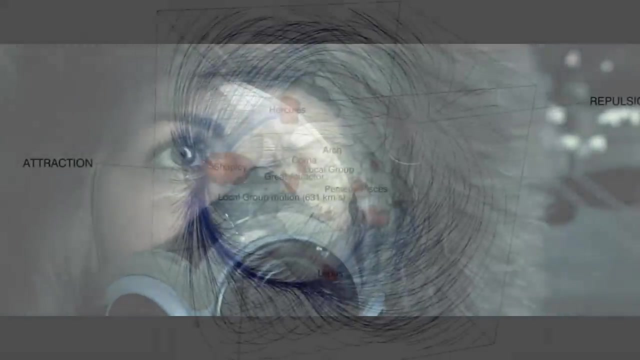 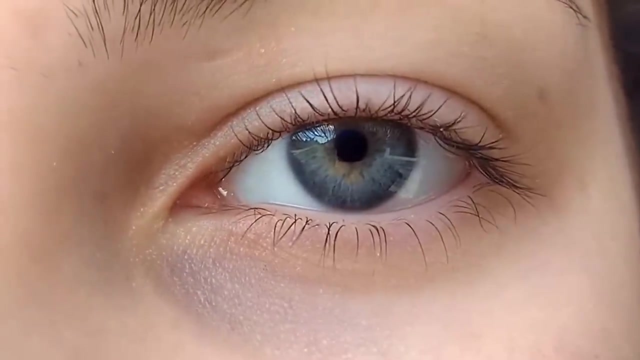 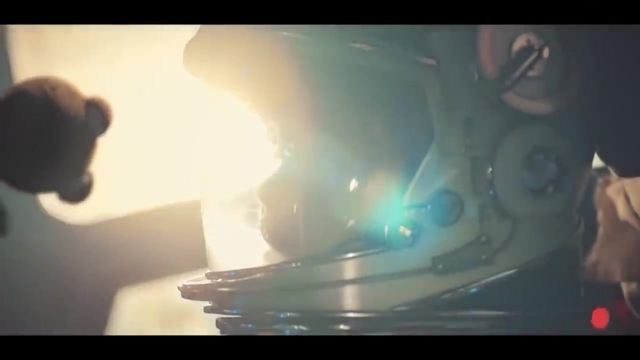 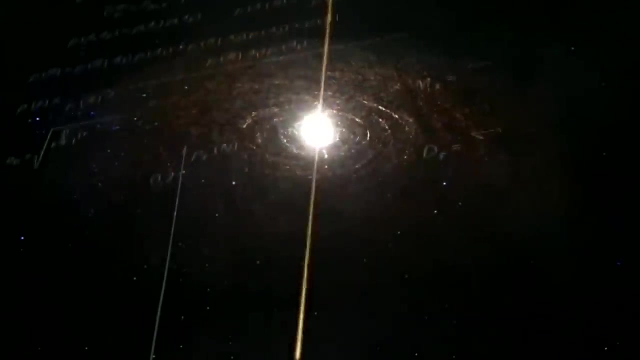 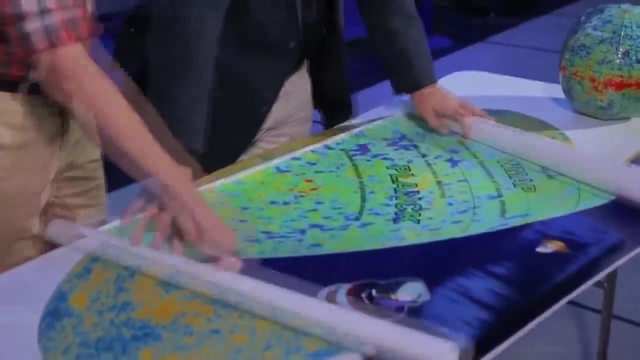 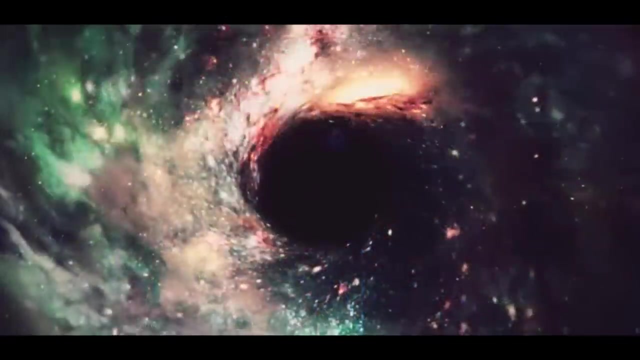 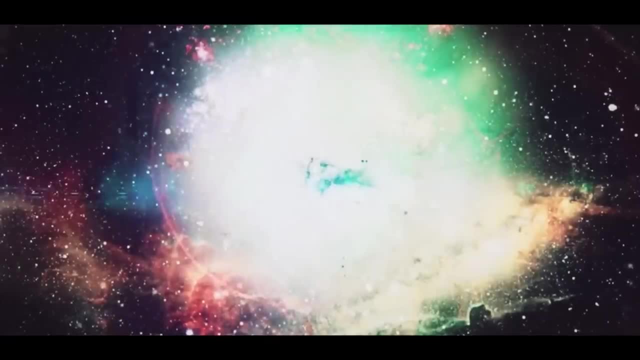 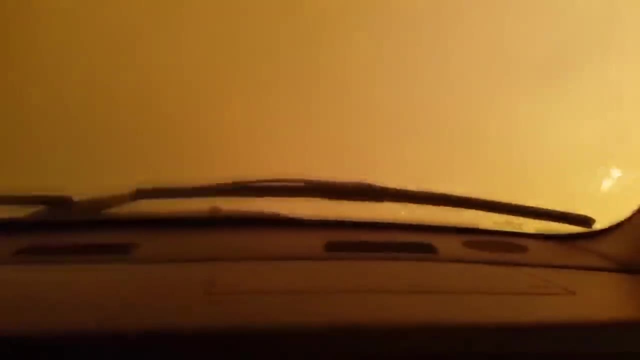 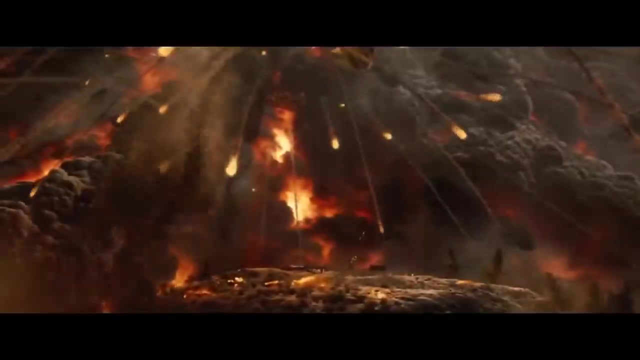 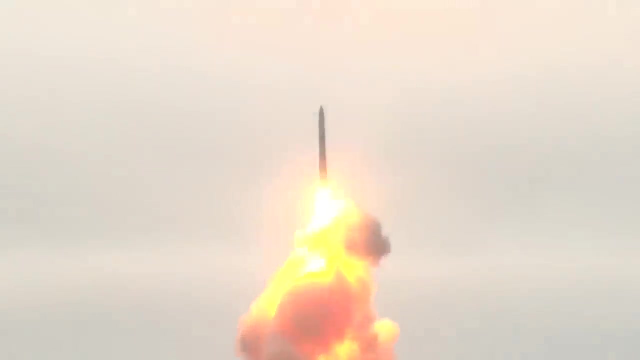 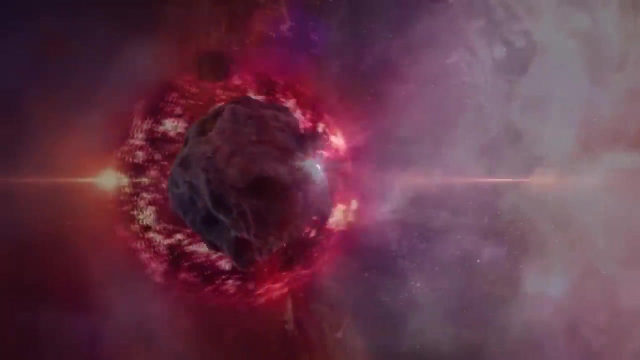 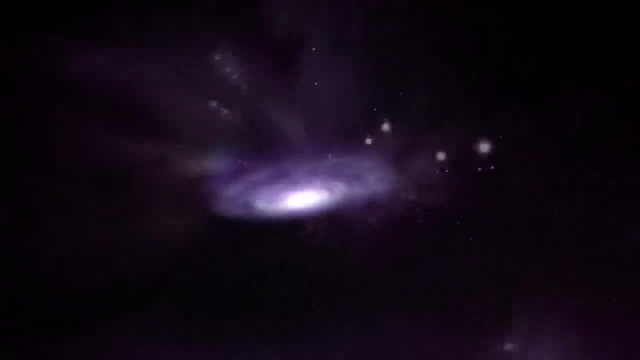 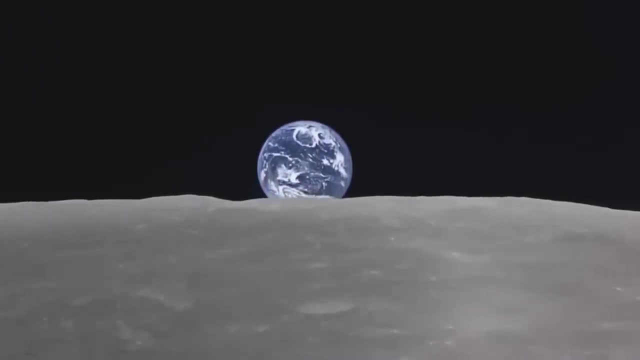 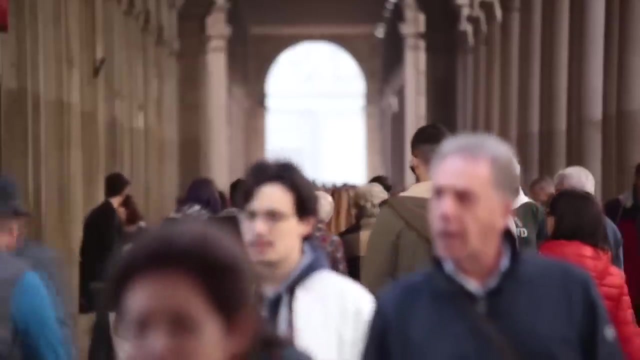 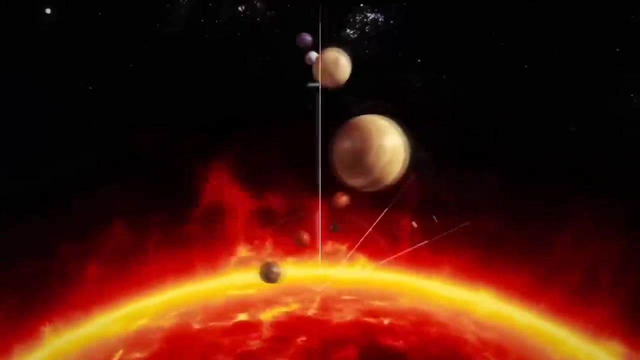 so, so, so. so it is well known that our universe has dimensions, or a number of position coordinates by which it can be measured: length, height and width. in other words, these are measurements that put bounds on the universe that is known to us. multi-dimensional space turns out to be more concentrated, in terms of informational and energy capacities, at one point of space. 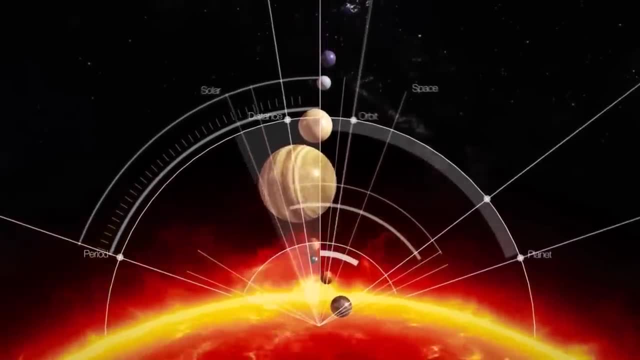 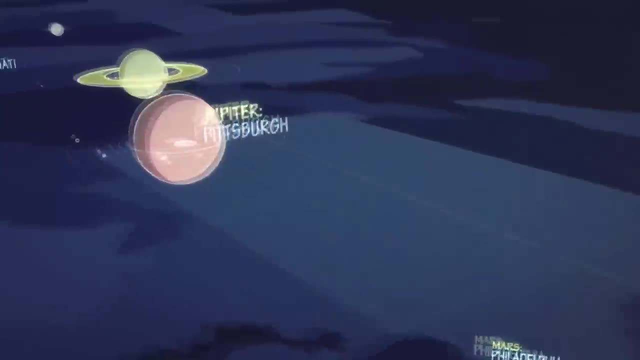 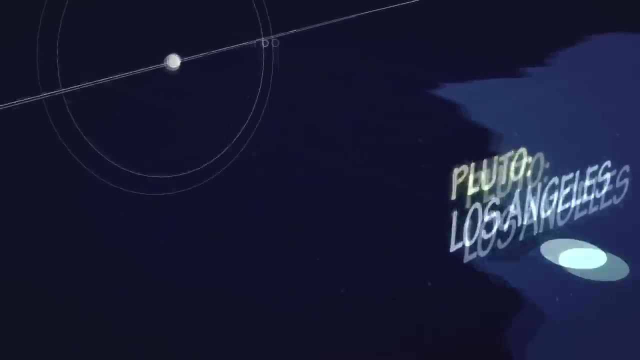 a higher dimension may be the concentrated information of all the other layers of reality of the lower dimensions. is it possible to discover that most inaccessible fourth dimension, and what does contact with it change in our world? if we ponder it for a while, we may possibly succeed in finding the answers. 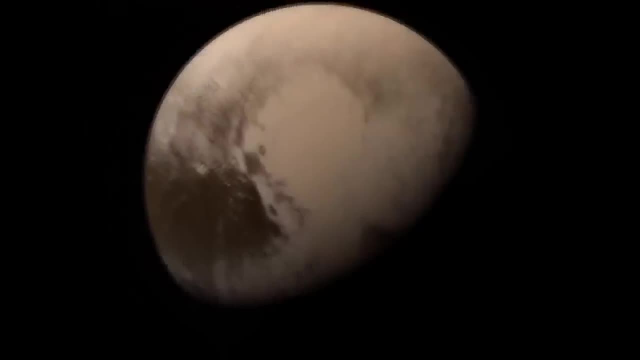 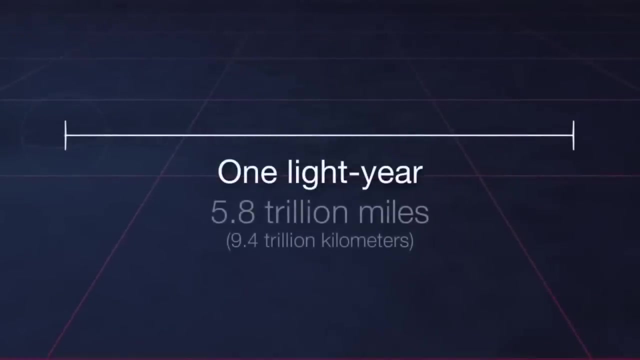 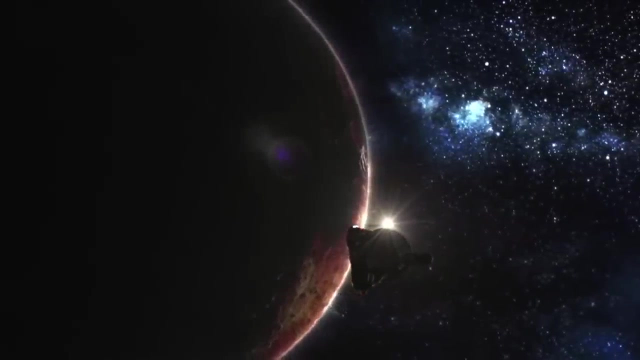 simply stated: if you place a cube in front of you, then you won't see its backside, since vision is two-dimensional. if the cube begins to rotate, then the brain analyzing it will understand that it is a cube and that there is a backside. but what our brain knows is one thing, and how it is seen by. 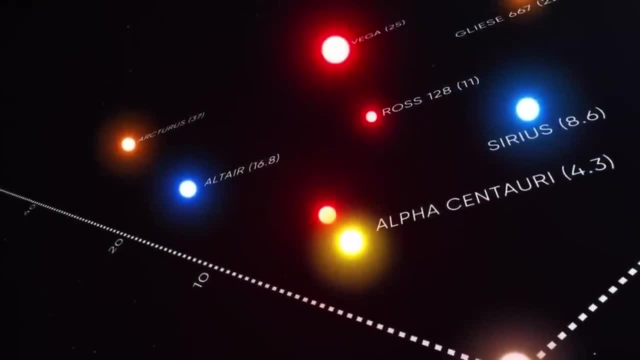 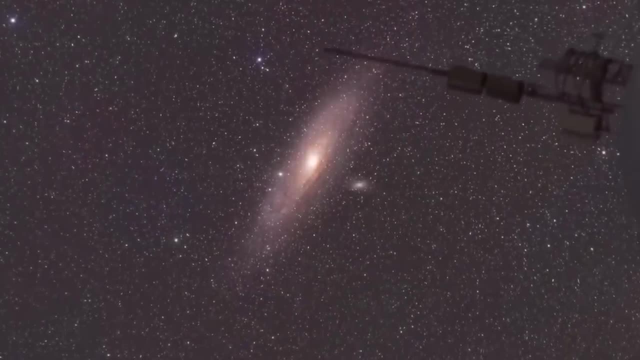 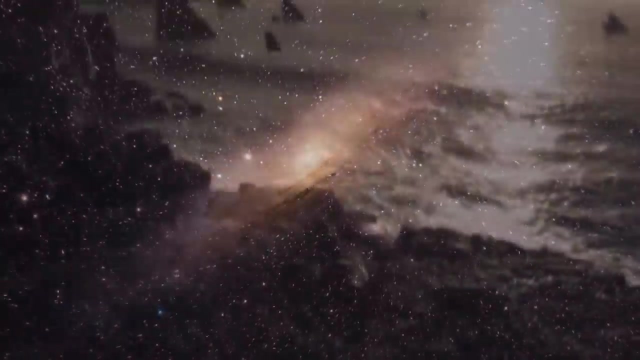 the eyes is another. if our vision were three-dimensional, then we would see the cube simultaneously from all sides, like a scanner at an airport. we would see all of space in its entirety and nothing could be hidden from us. that is to say, we must observe from without, as if we are watching a movie or even our own dream, in which we can sometimes. 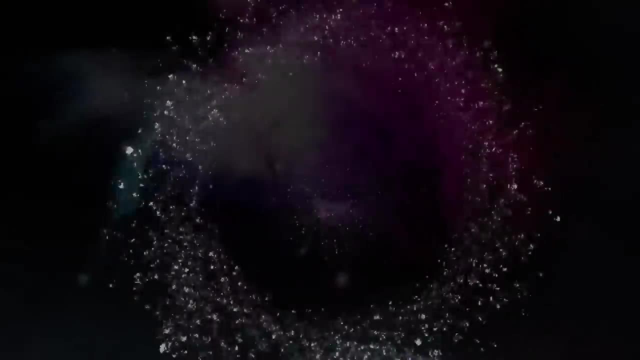 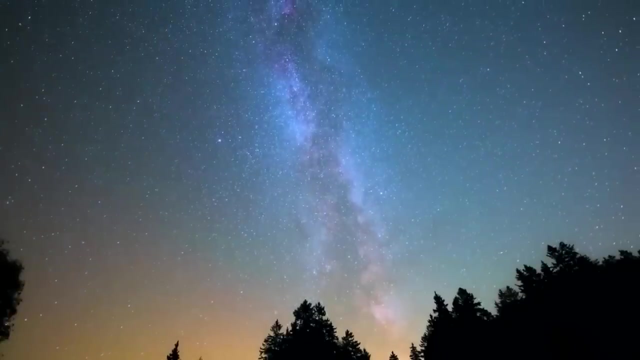 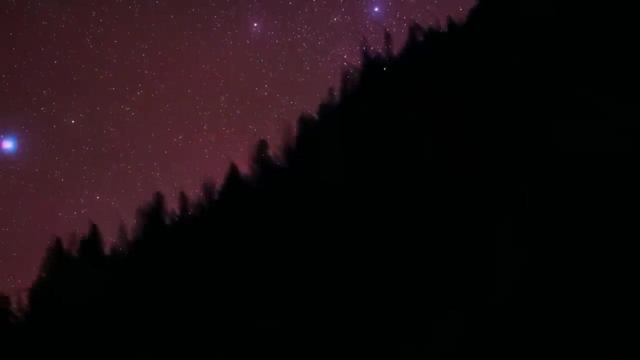 evaluate ourselves from the sidelines. indeed, if we were to live in a two-dimensional space on a flat plane, we would have to stretch our imagination considerably in order to think of how to move a rectangle off of the flat plane on which we live. well, conceptualizing a four. 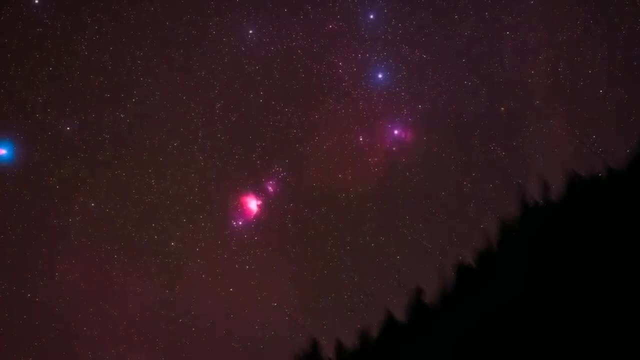 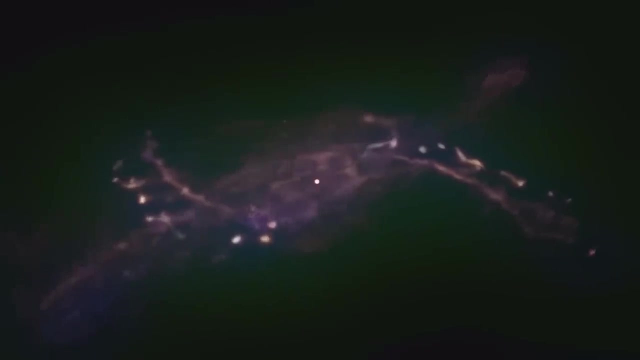 dimensional space is also quite difficult for us. a three-dimensional space is a space in which the position of a point is different from the position of a point is different from the position of a point is designated, as we have already said, by three numbers. for example, the position of an aircraft. 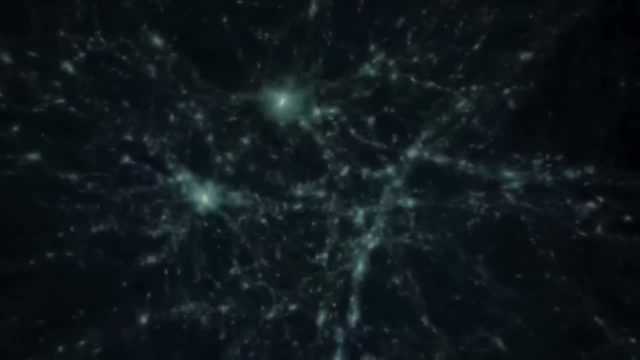 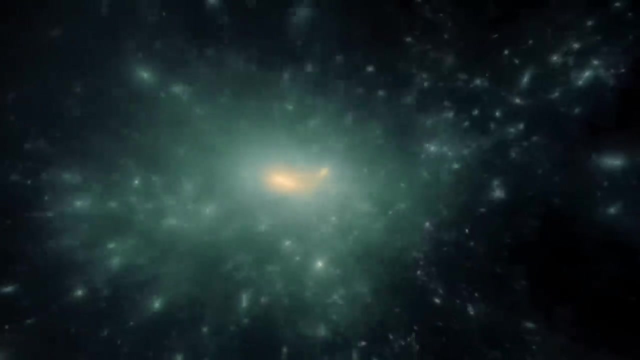 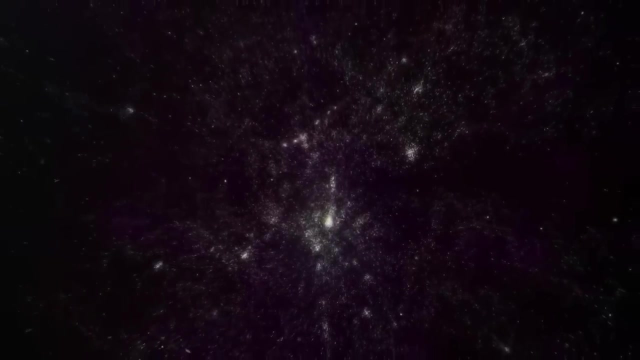 is indicated by longitude, latitude and altitude above sea level. in a four-dimensional space, an object corresponds to a four number coordinate. a four-dimensional cube is obtained by sliding an ordinary cube along in a particular direction that doesn't lie within our three-dimensional space. where this direction is, or how to transcend our limits. 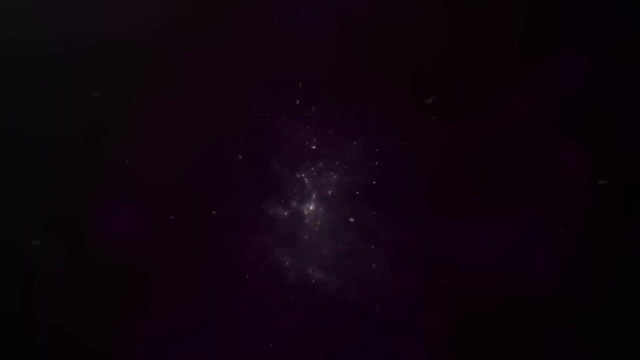 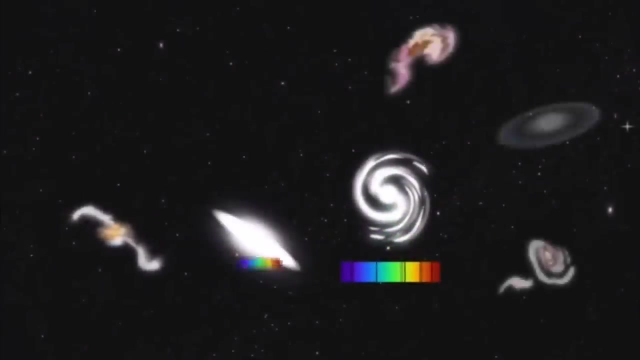 is a three-dimensional space. where this direction is or how to transcend our limits is a three-dimensional space is difficult to say as well as to perceive, but use your imagination and indulge in fantasy. and why not? often this type of four-dimensional cube is called a tesseract, the equivalent of a 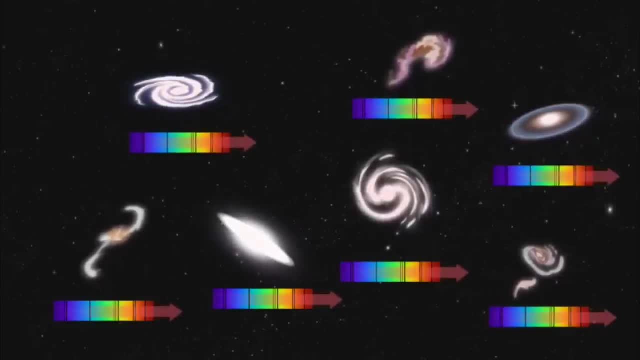 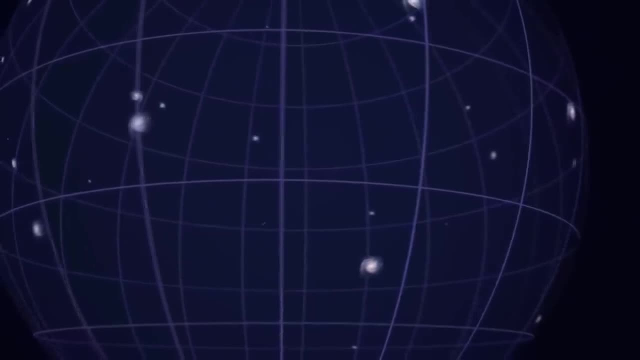 usual three-dimensional cube generalized in a four-dimensional space. try to picture the properties of a hypothetical 4d space. to begin with, we need to understand if a fourth orthogonal axis is feasible in the of a hypothetical 4d space. to begin with, we need to understand if a fourth orthogonal axis is feasible in the 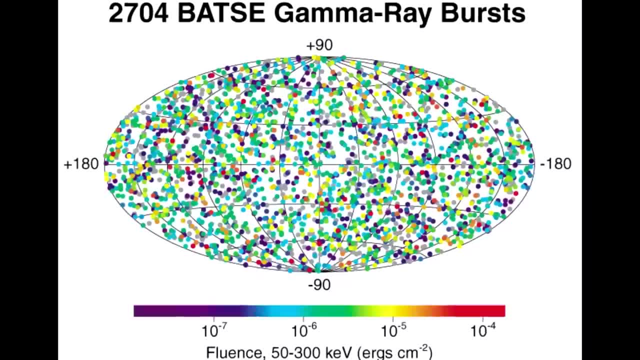 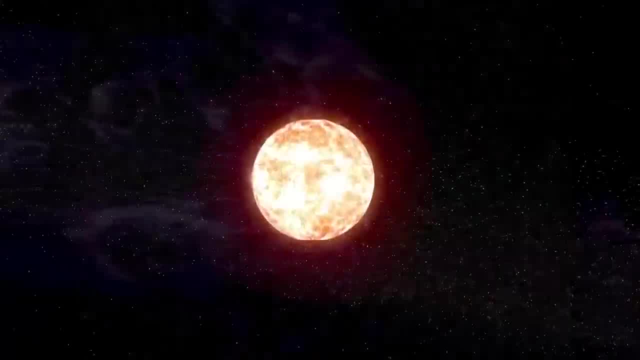 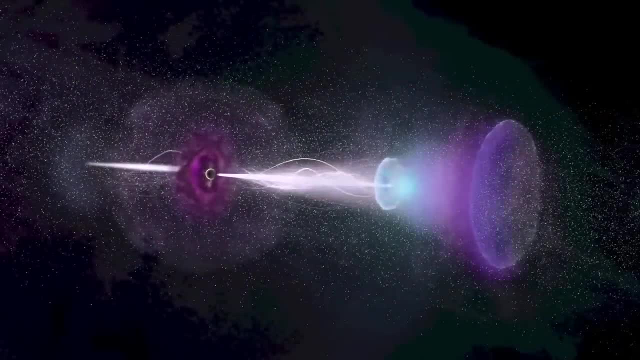 coordinate system and if so, where is it located? indeed, for us, our familiar three-dimensional space is associated with three axes of the coordinate system, and if we can't even imagine something that is mentally create its corresponding image, does that then mean this? something does not exist it. 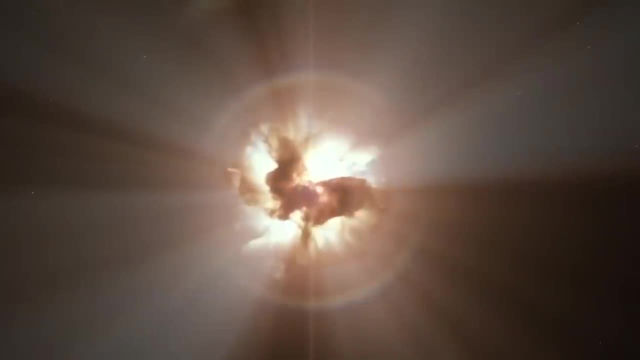 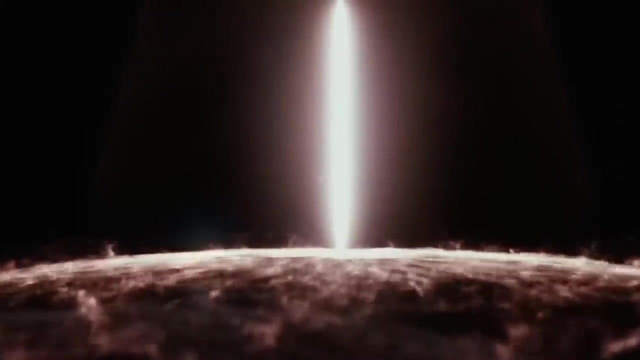 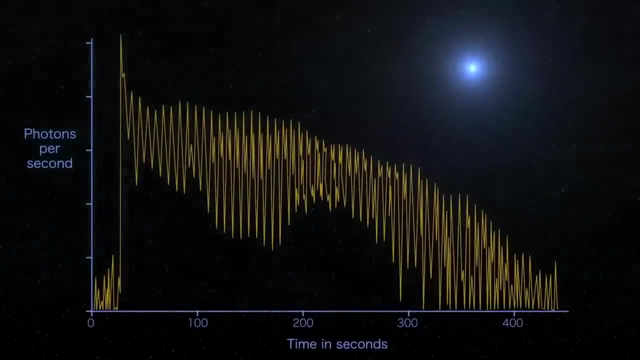 appears. so this poses the question: why exactly are there three spatial dimensions? no more and no less? it is a apparent, because the atom, and along with it all the rest of matter, has precisely three spatial characteristics: length, width and height. what characterizes these three attributes of space? 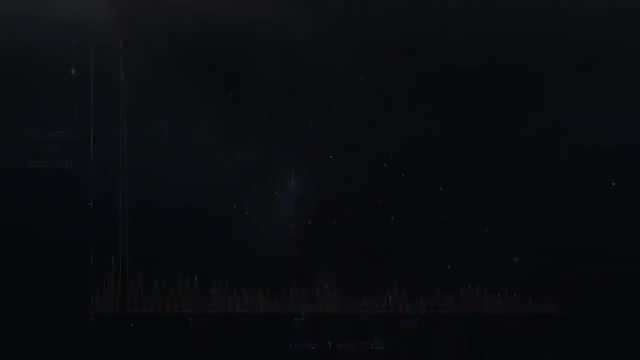 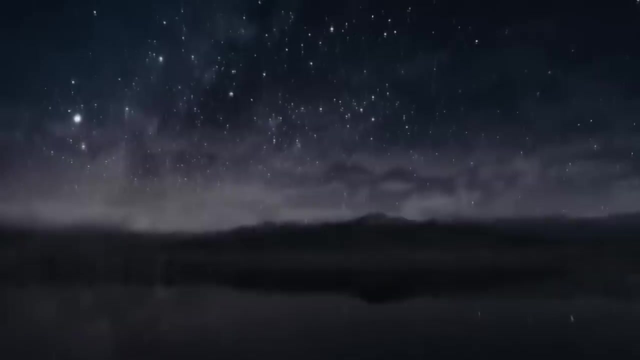 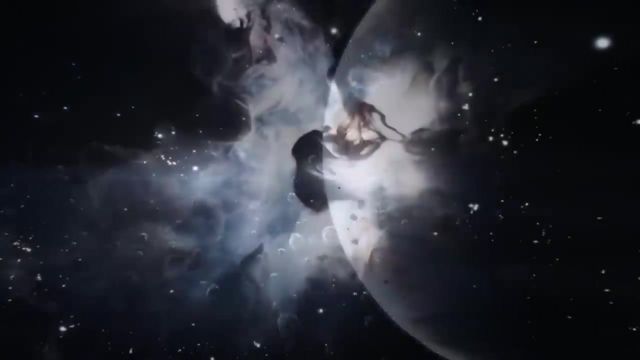 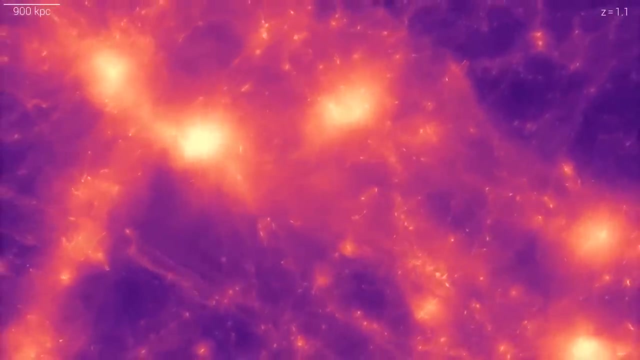 naturally the spread of tangible objects in three possible directions: forward, back, left, right, up down, the usual pattern for a kangaroo. is it possible to see something from the fourth dimension? most likely, yes, but it will only be a projection, a part of what it really is. that is for inhabitants in a 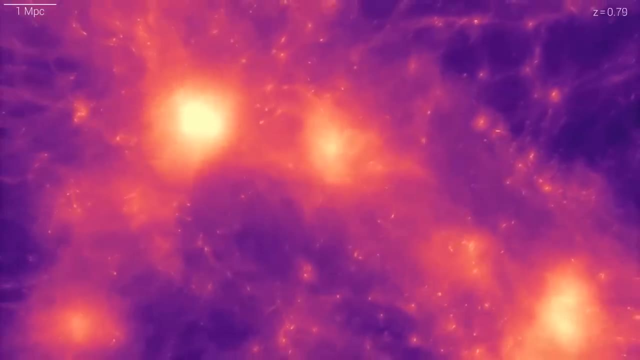 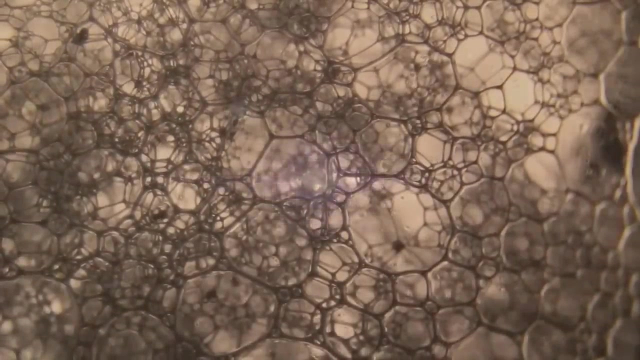 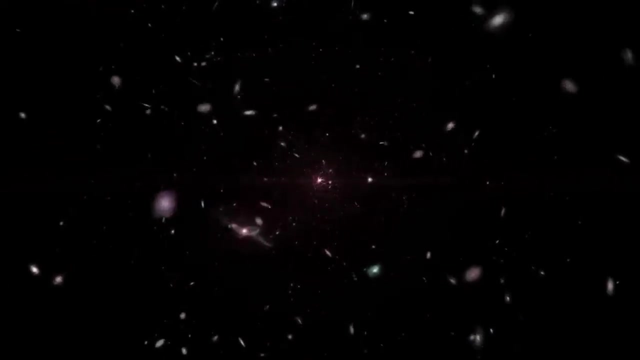 one-dimensional existence, a line- any two-dimensional beings would be perceived merely as component parts of one dimension whatsoever- transcends the bounds of this dimension, won't be noticed, as the eyes are already out of the picture. in the same way, the inhabitants of a two-dimensional space, a flat plane, 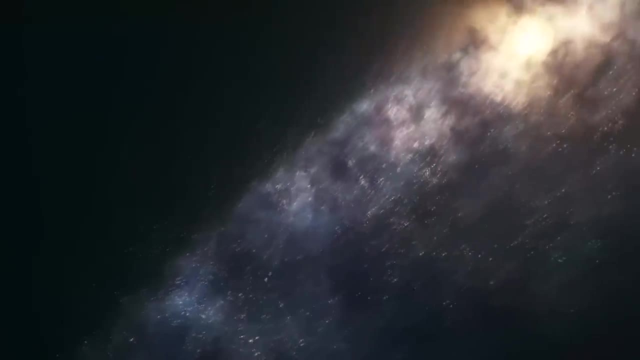 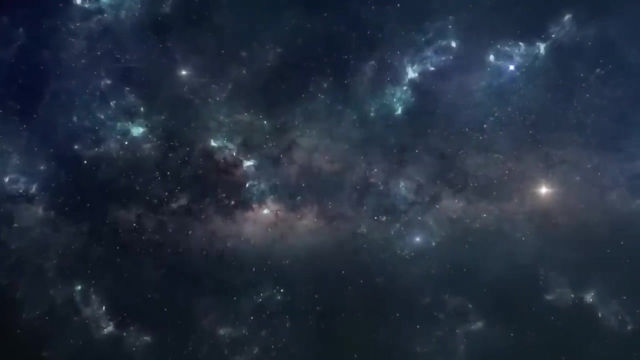 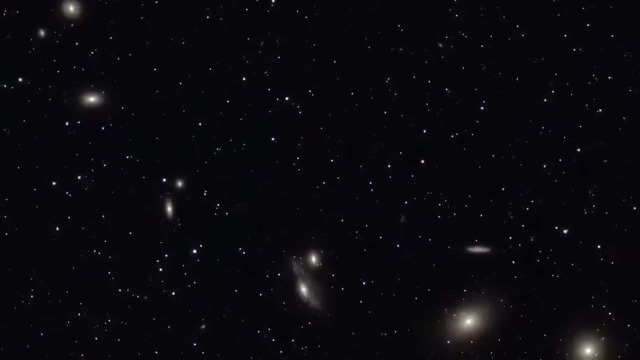 can see the inhabitants of a three-dimensional space only in the form of their two-dimensional imprints or projections. they also simply don't see anything in the third dimension. this means if a person were to end up in this two-dimensional space, then in the best-case scenario, the local 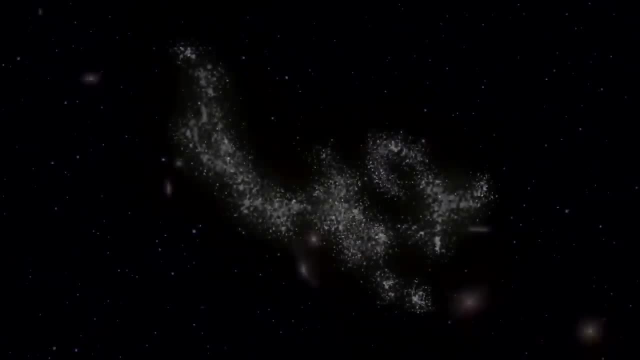 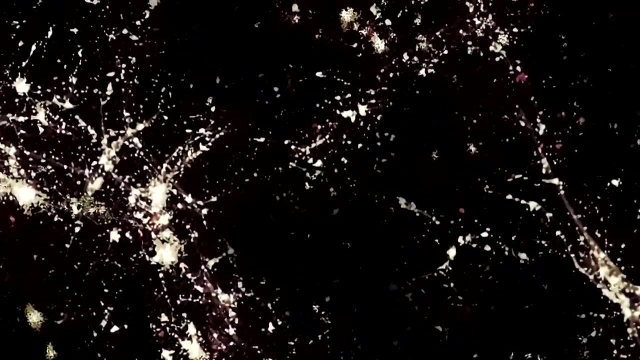 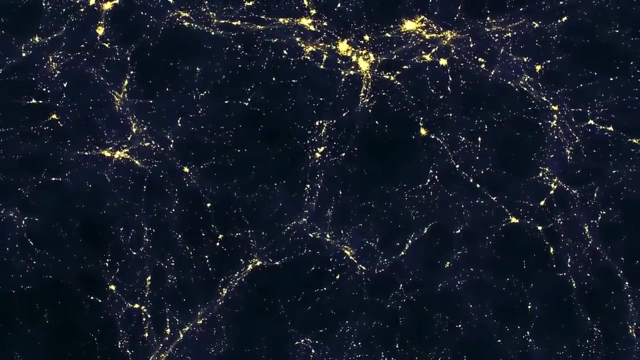 inhabitants of the flat plane would become acquainted with his footprints and, in the worst case, his cross-section. but if a fourth dimension does exist, then what would creatures or life look like on another world? in order to answer this question, we need to imagine: how would the space 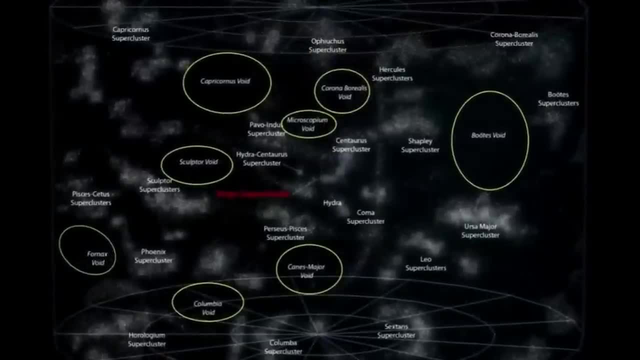 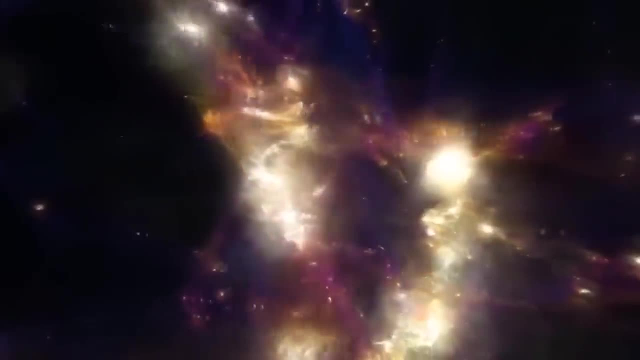 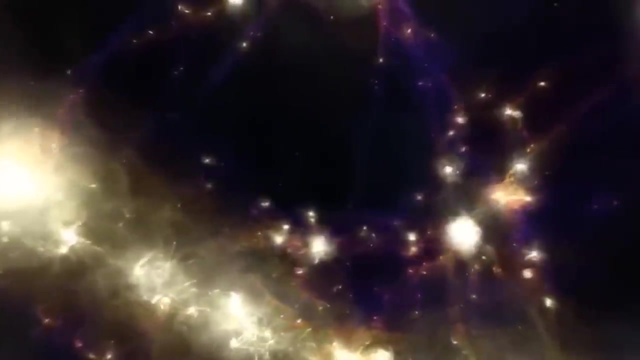 of our world change. if it became four-dimensional, it's logical to assume that an additional side would appear in which movement is possible and a restructuring of configuration at an atomic level would begin. the electrons around the nuclei of atoms, having received an unrestricted new side, will begin to rotate in the fourth direction. the nucleus of the atom will begin to rotate in the 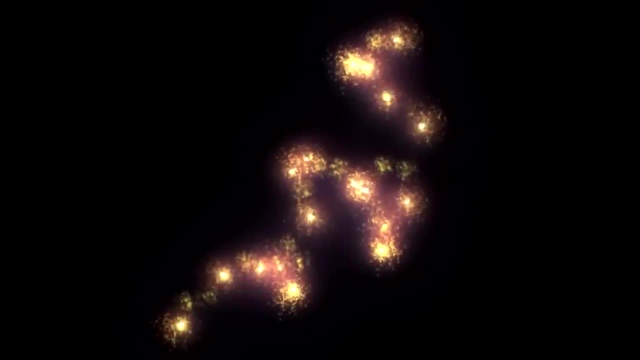 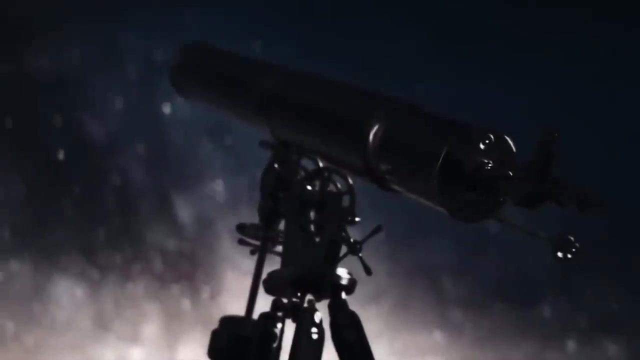 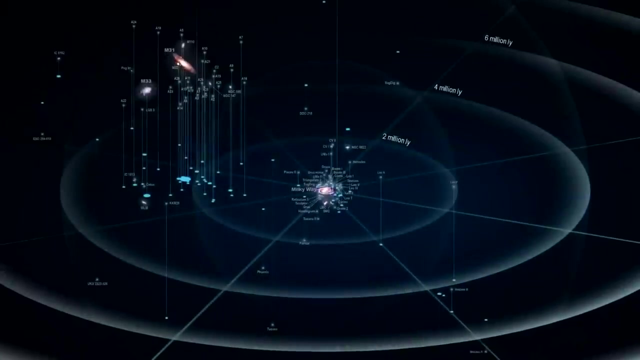 atom will also be restructured and the chemical properties of the elements will change, which of course will fatally split all forms of 3d life. meanwhile, after the restructuring of atoms in the fourth dimension, our planet earth will be only one atom in thickness, but the earth's mass will 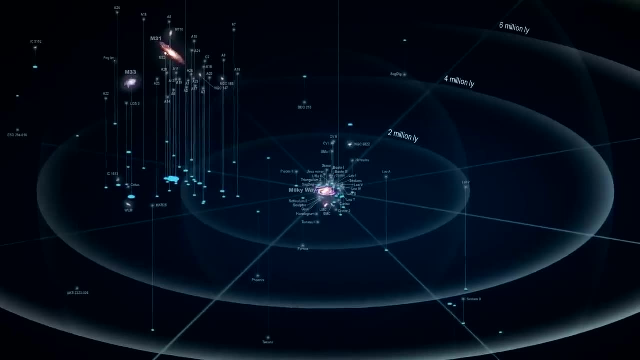 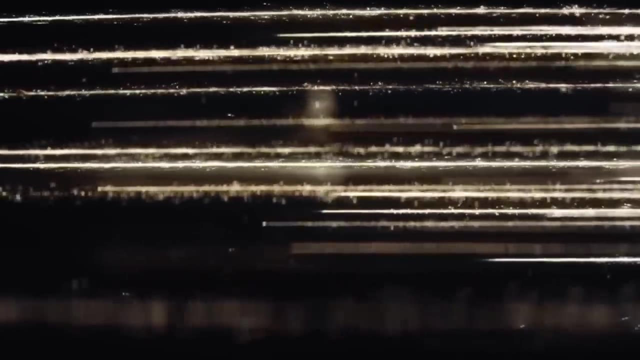 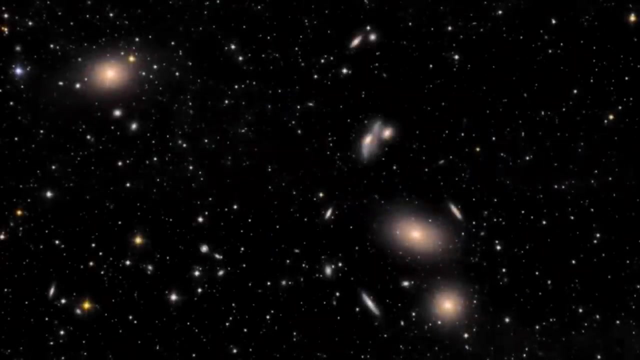 remain the same as it was in the three-dimensional space, due to which it will collapse in the fourth dimension under the weight of its own mass and, in the end, form a four-dimensional hypersphere. The same will happen to the Sun and the other planets and stars. Gravity will 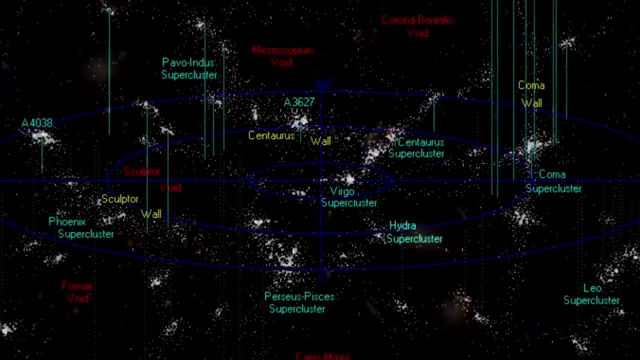 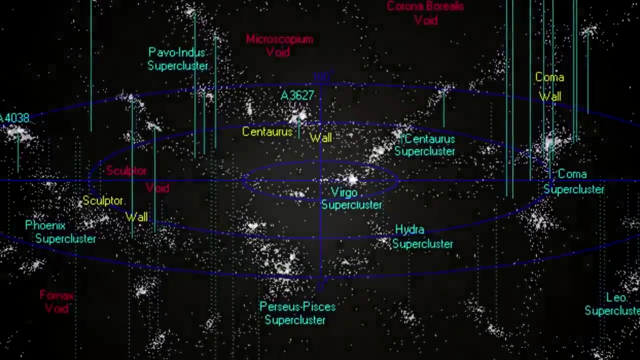 begin to spread out into the new direction, due to which there will be a chaotic change in the orbits of all of the celestial bodies in the entire universe. Ultimately, after a catastrophic restructuring, everything will stabilize and there will be a new universe. 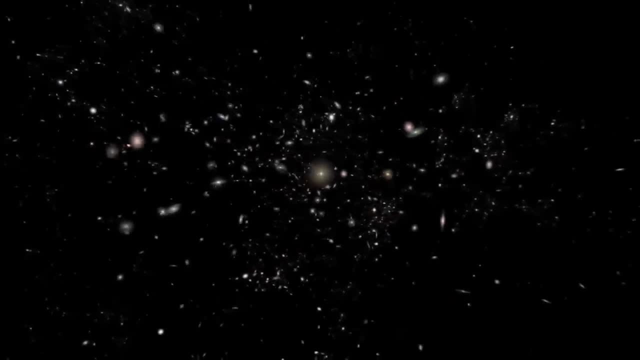 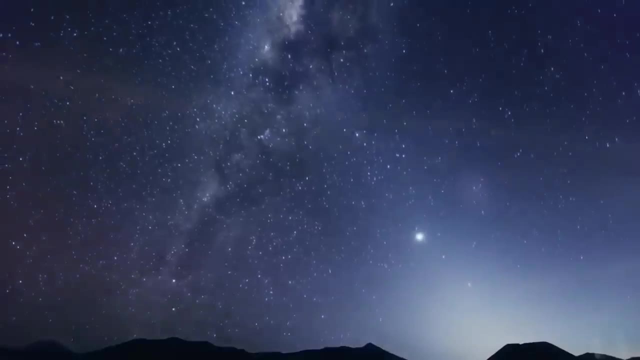 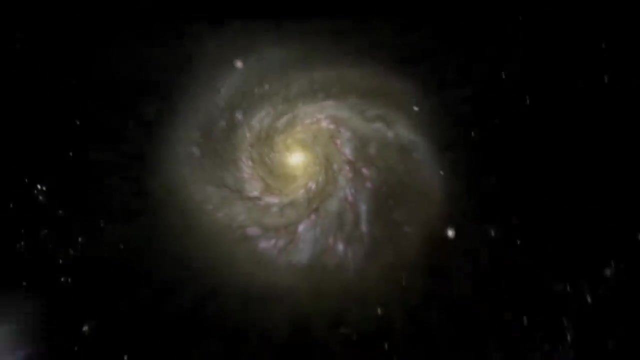 True. nothing living on it up to that moment will remain. How many dimensions are there beyond our perception? For now, it remains a mystery. In the meantime, the world truly is multidimensional, Based upon a mathematical hypothesis: an infinite number of spatial 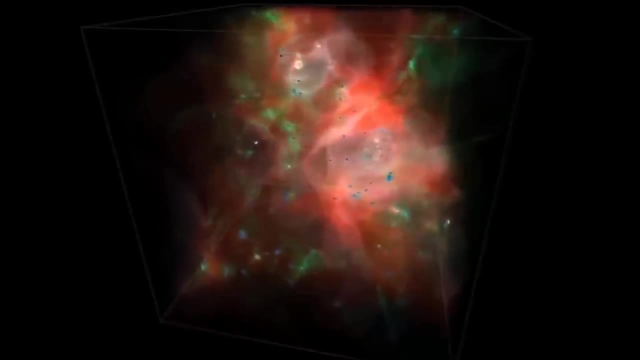 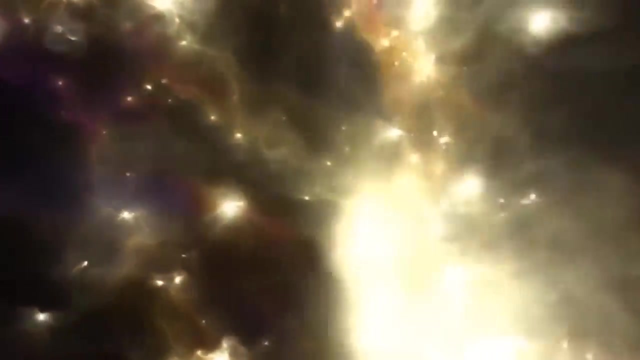 dimensions can exist. Modern physics also adheres to this logic. only, it is impossible to count the number of these types of dimensions, But owning to the understanding of at least a few of the additional dimensions, we would obtain a good tool for managing the world. 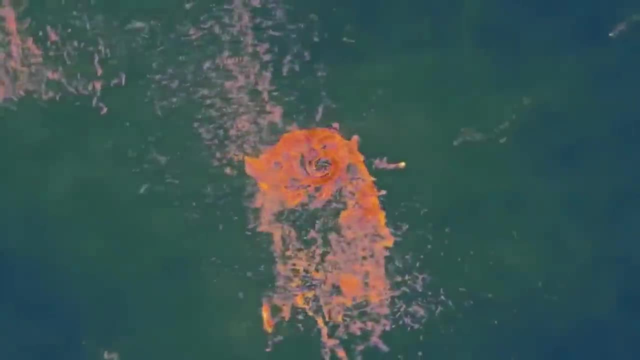 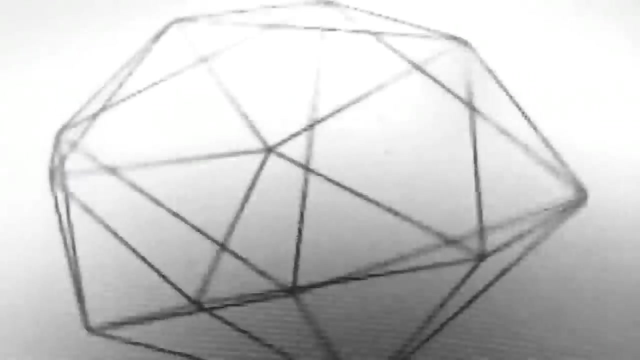 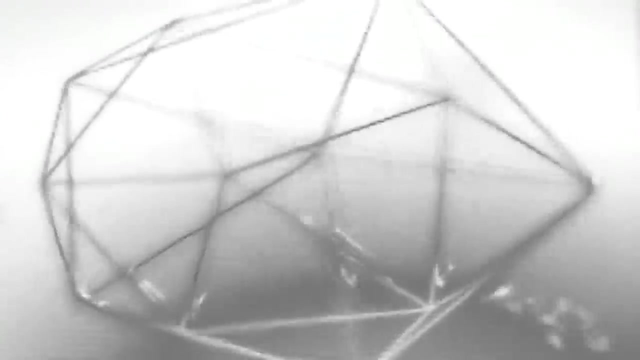 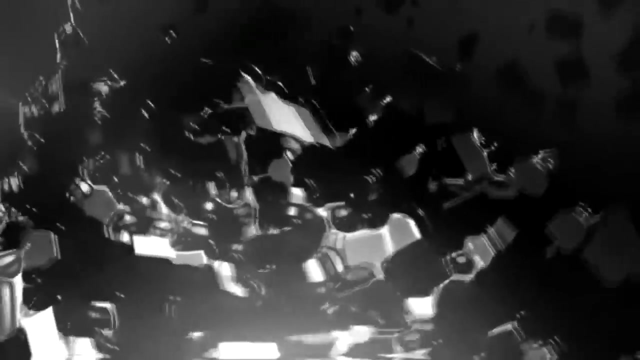 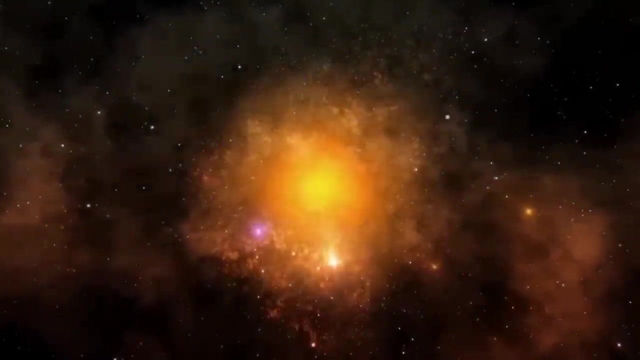 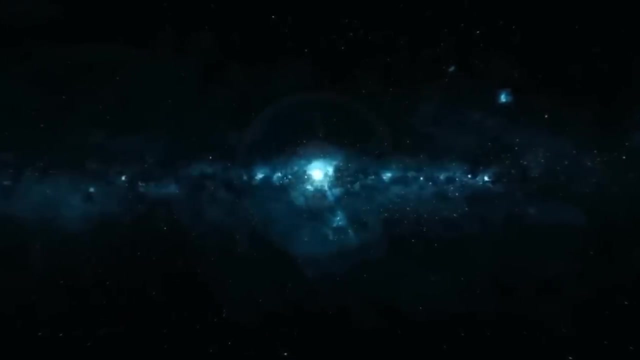 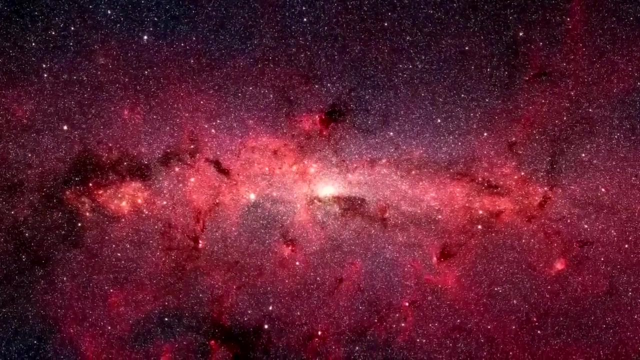 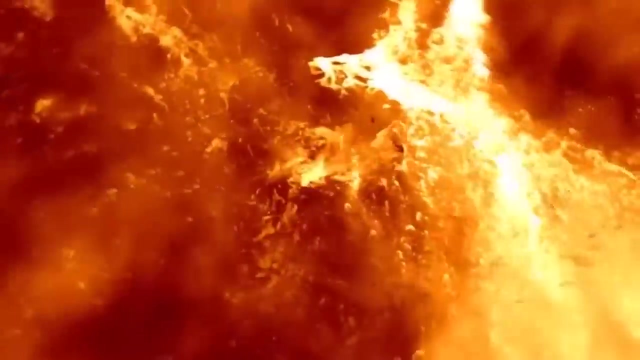 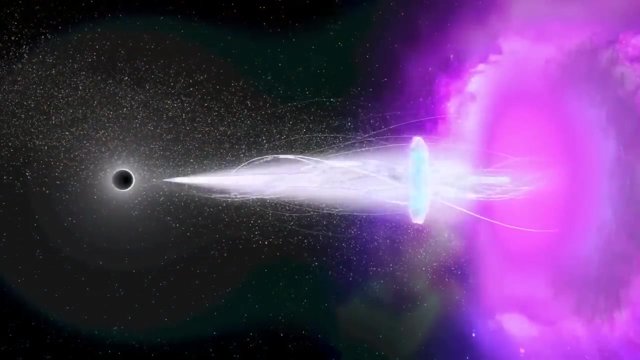 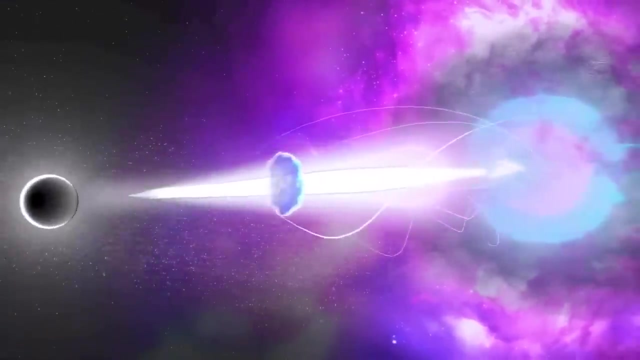 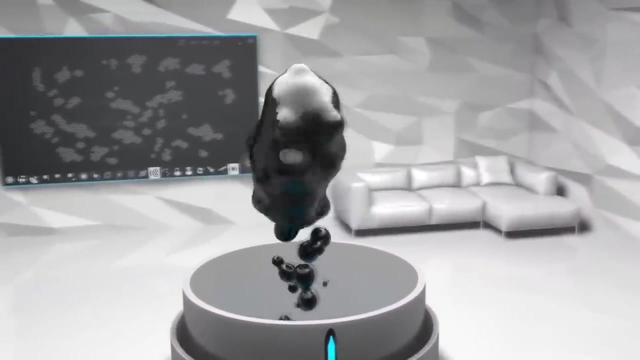 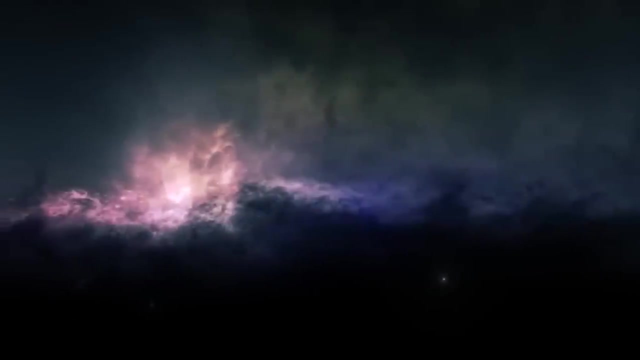 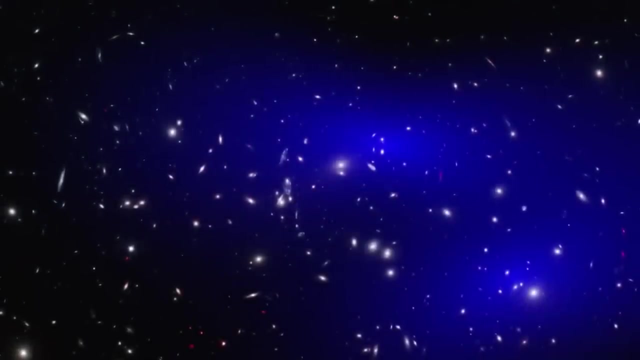 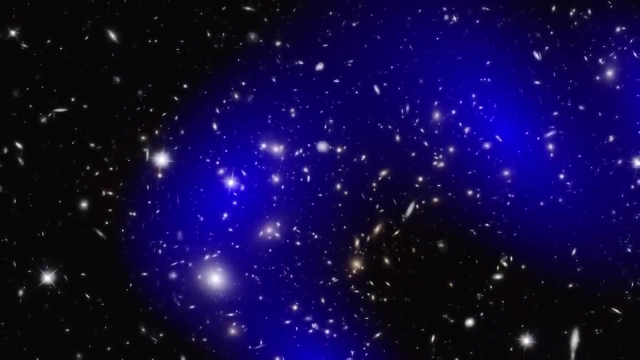 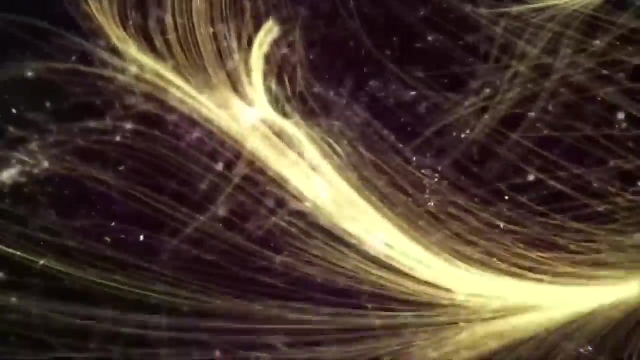 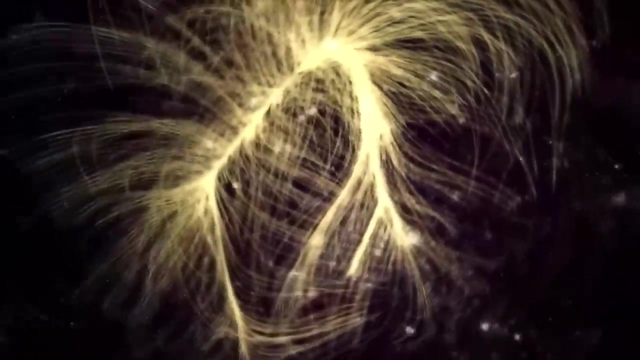 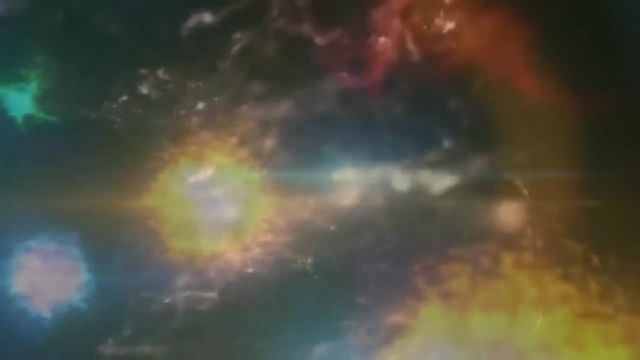 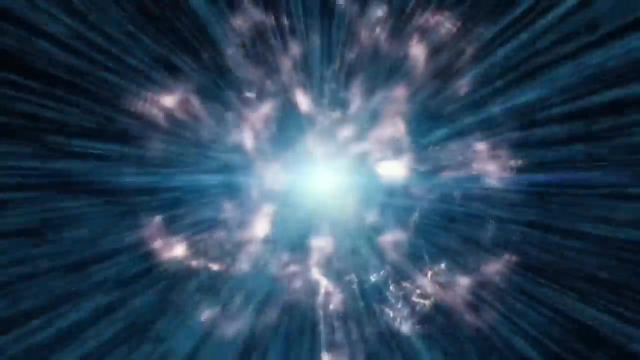 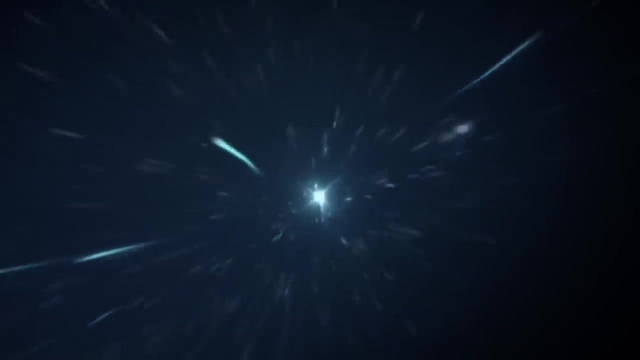 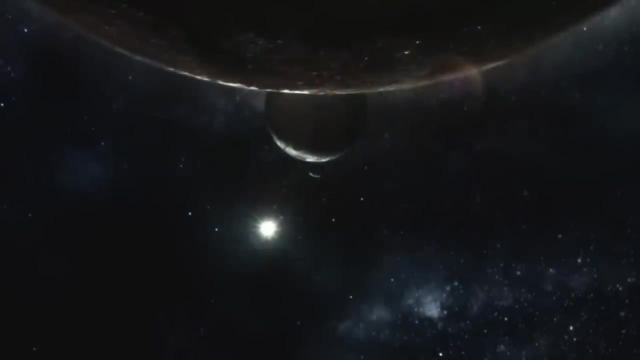 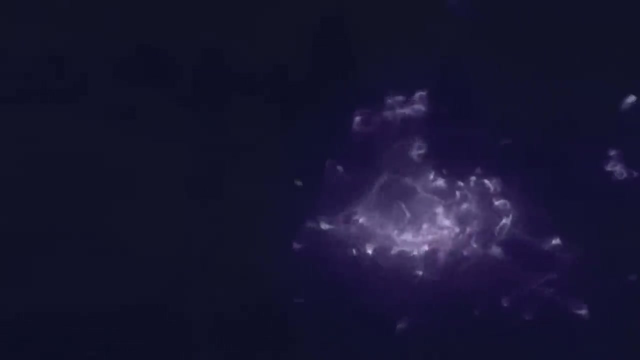 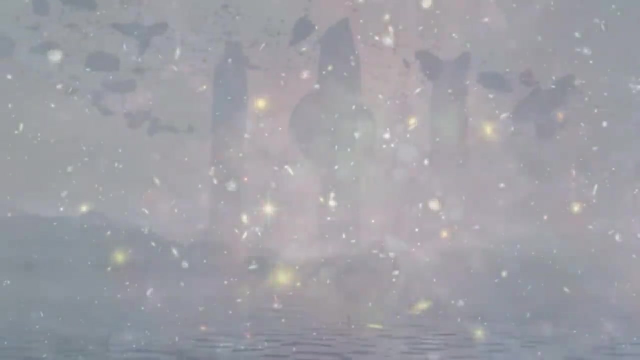 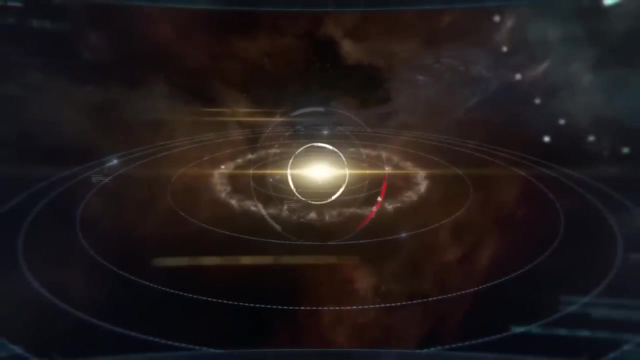 around us. Transcription by ESO. Translation by —. Transcription by ESO. Translation by —. Transcription by —. Transcription by —. Transcription by —. In the distant and mysterious valleys of space, where the stars twinkle against the dark mantle of night, a huge galaxy is hiding which attracts the eyes of astronomy lovers, dreamers and writers. 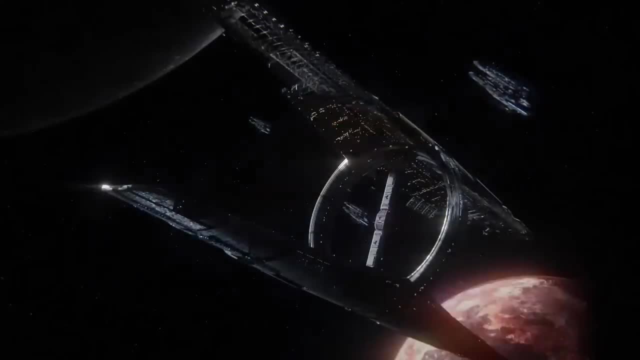 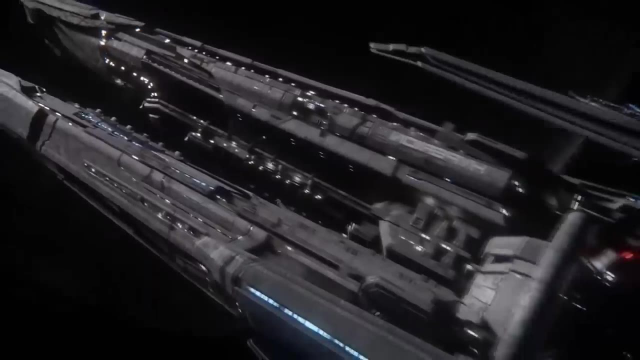 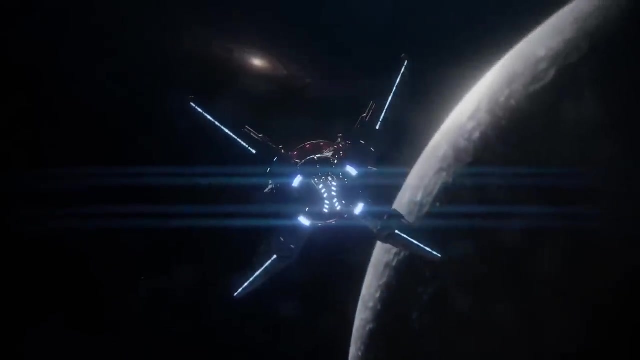 This galaxy is named Andromeda And today we will make a grand journey to her heart, to the very center of the galaxy. An alluring adventure, mesmerizing with bright colors and the promise of new discoveries, begins right here: Andromeda Galaxy or M31.. Our nearest stellar neighbor. 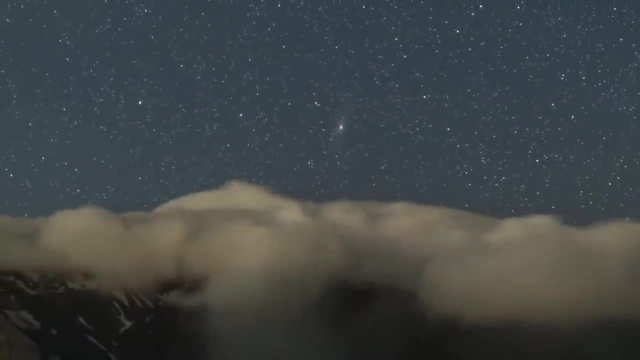 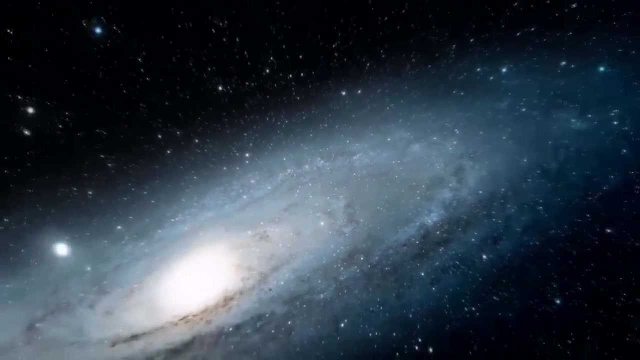 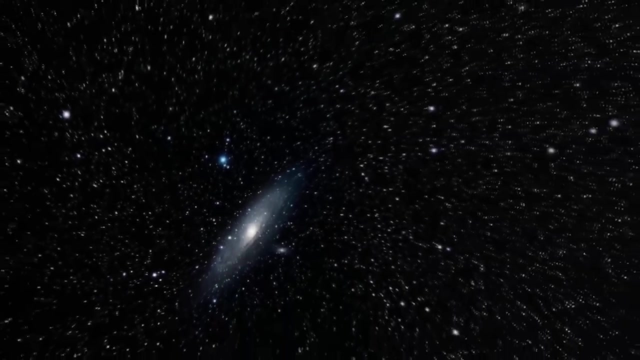 On a clear night, it can be seen in the sky with the naked eye. It is located at a distance of about 2.5 million light-years from Earth and its diameter is approximately 200,000 light-years. And although it seems incredibly far away, but in fact it is not so at all. 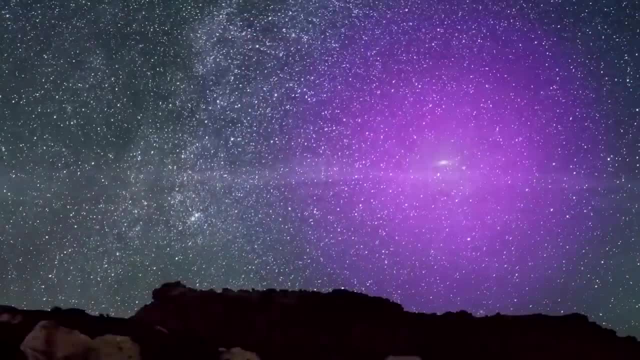 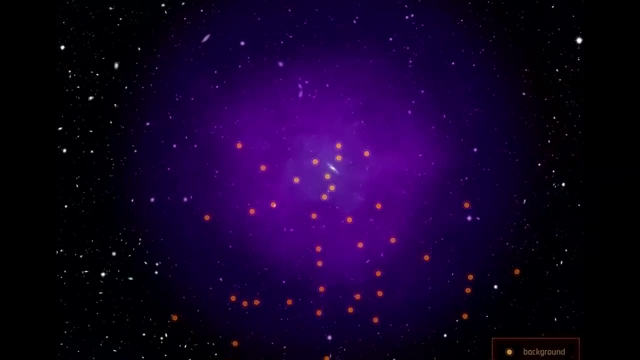 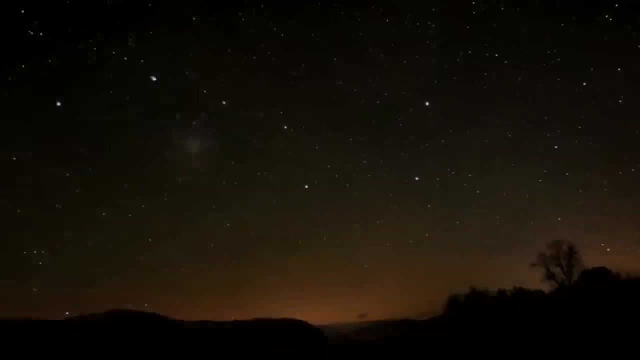 Unlike the others, the galaxy has a bright future. It has a bright, gallow, or giant luminous cloud consisting of stars as well as very discharged ionized gas. If this halo could be seen without magnifying glasses, in the visible spectrum it would be three times larger than the constellation Ursa Major. The area of the huge head around the Andromeda Galaxy is huge and is located about halfway to the disk of the Milky Way and in some places even bumps into our galaxy's own halo. Of course, the galaxy is 믿습니다. Yes, in fact, the galaxies are incredibly close to each other. 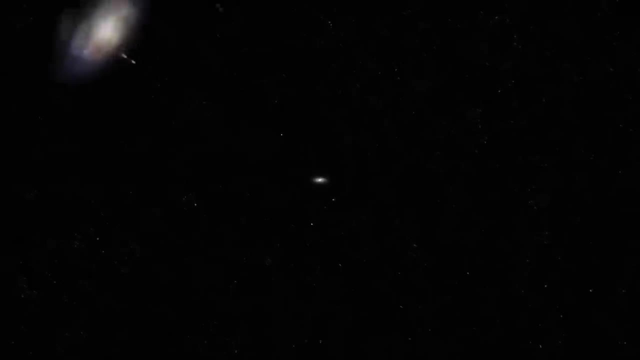 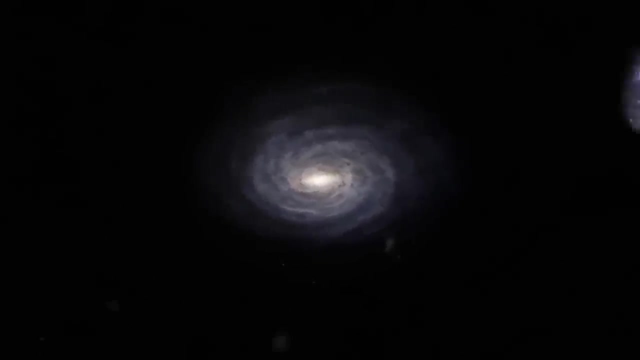 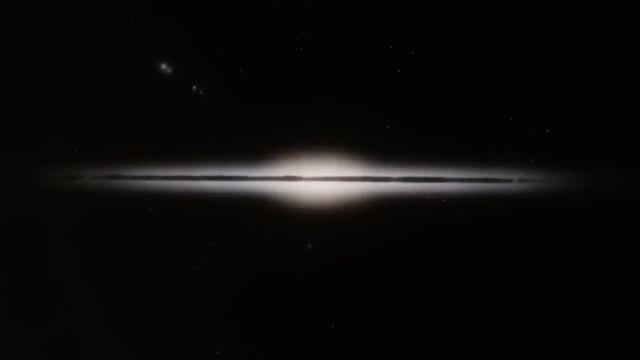 We are starting our journey Flying through the spherical component of M31,. we are getting closer and closer directly to the disk of the galaxy with noticeable spiral arms. However, the Andromeda Galaxy, unlike the Milky Way, has a significantly thickened disk. 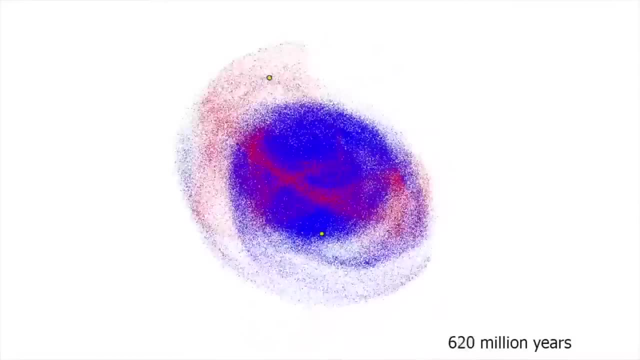 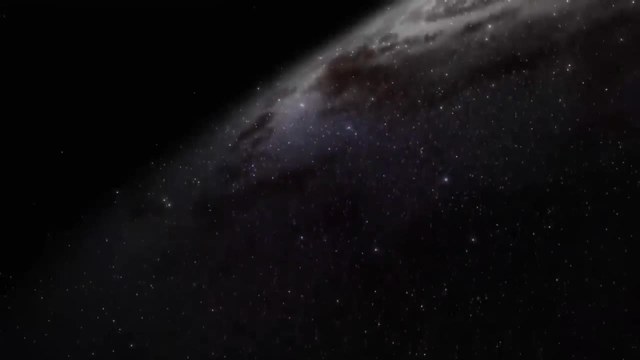 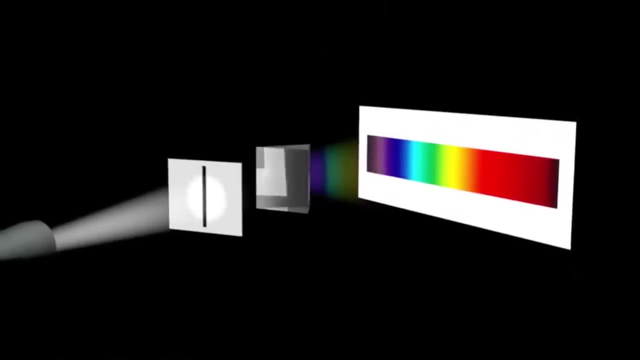 According to the standard cosmological model, most galaxies were formed as a result of, or acquisitions of, small satellite galaxies, And the presence of a blurred, thickened disk in the Andromeda galaxy is a sign of just such mergers And using spectra of different ages and 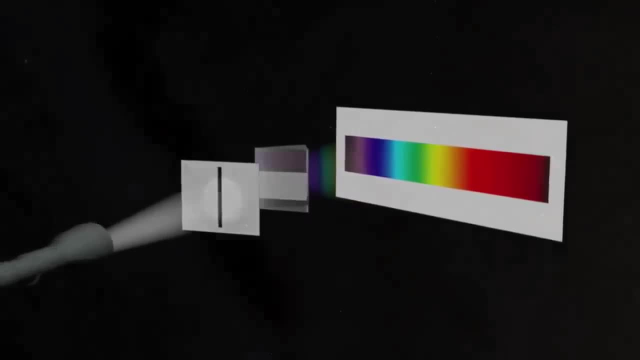 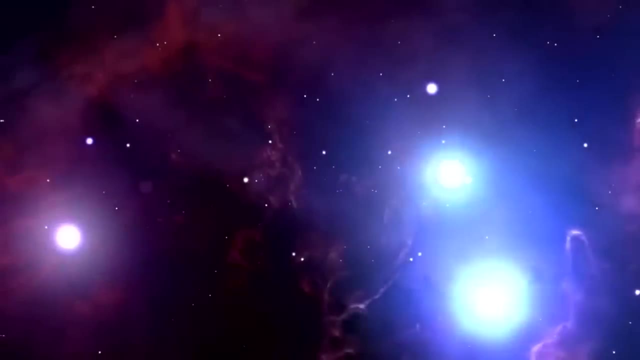 types of stars, it is possible to calculate the variance, that is, to determine how much the speed of a given star differs from the average speed of its nearest neighbors. The results were very interesting. The older the stars, the higher the dispersion and velocities. That is, it is much. 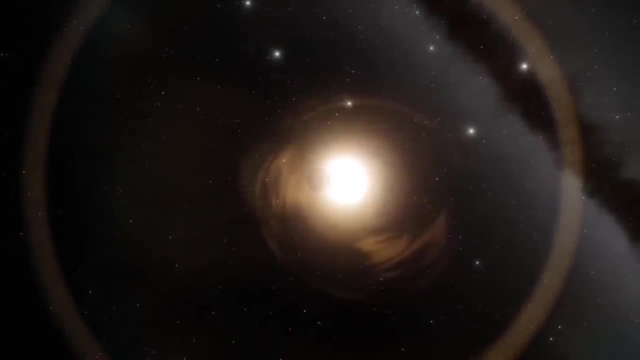 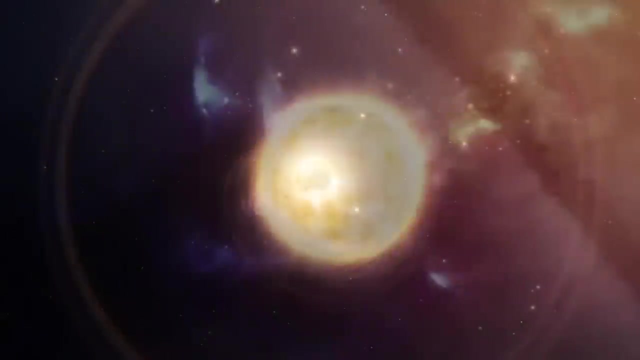 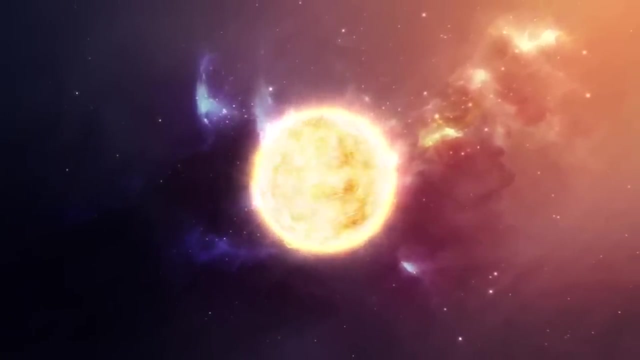 more likely that young stars are quietly rotating around the center of Andromeda, while stars in which the nuclear reaction is at an end are moving at enormous speeds. Moreover, even for the calmest stars in Andromeda, the dispersion is three times higher than that of the stars of the Milky Way. 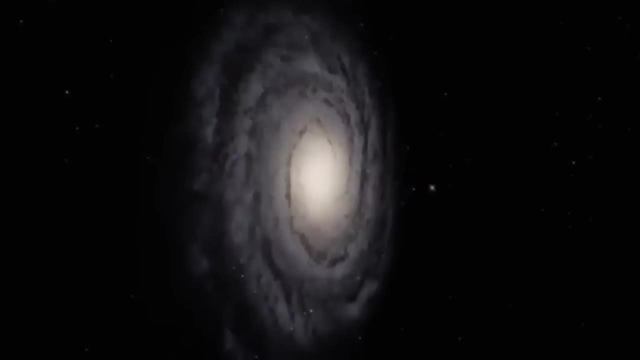 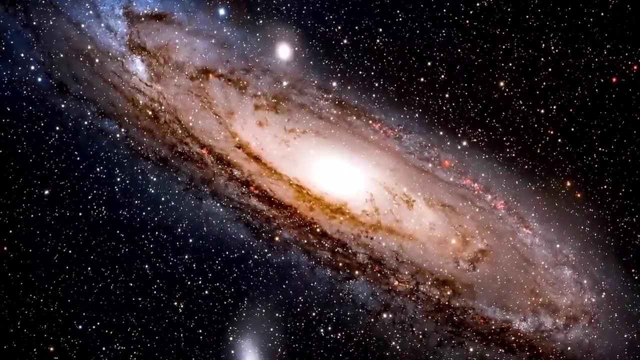 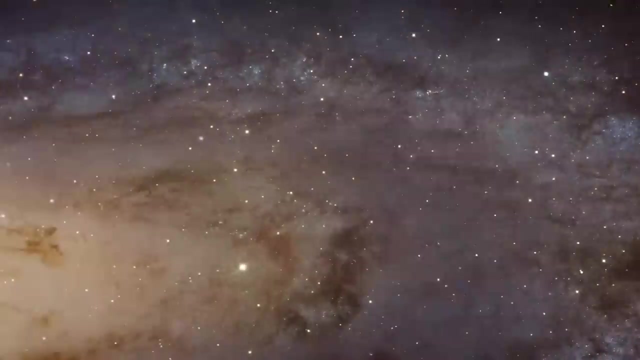 This clearly indicates that the history of the galaxy M31 is much more complex and full of events. There are many segments of spiral arms in the disk of the galaxy. In the inner regions of the galaxy, they stand out mainly due to dust, and in the outer ones due to supergiants and regions of ionized hydrogen. 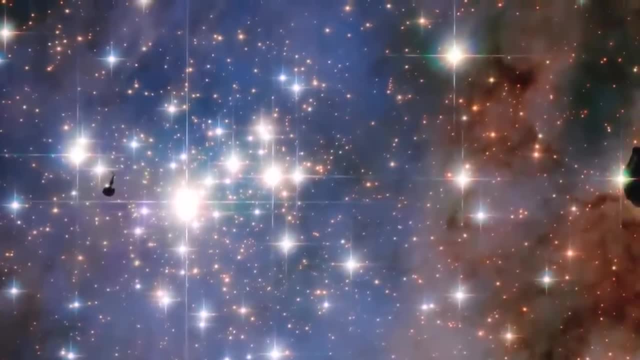 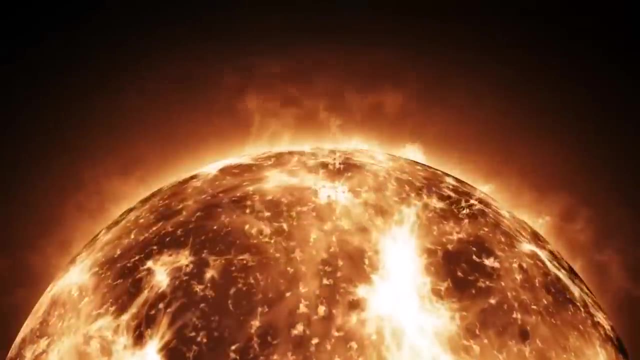 M31 contains more than 400 globular clusters. among them, the Mile 2 cluster is the brightest cluster in the local group, which has a mass of 7 to 15 million solar masses and is possibly the core of a dwarf galaxy destroyed in the past. 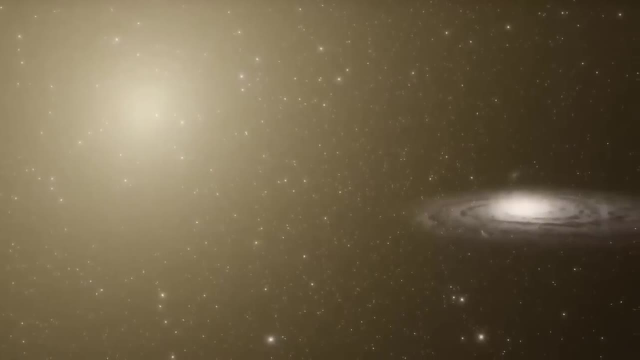 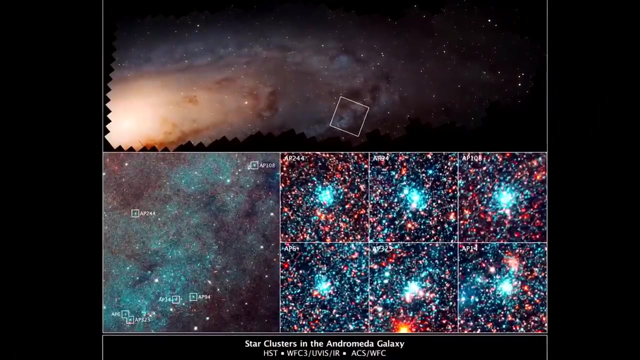 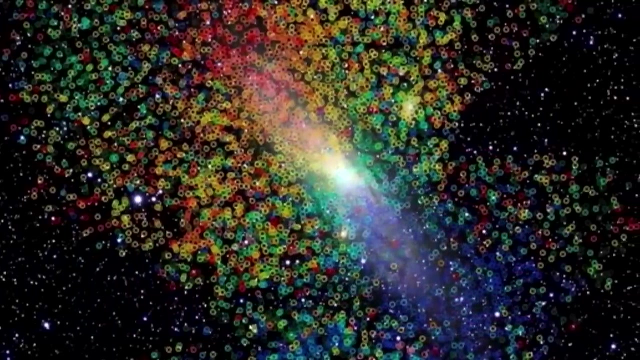 On average, globular star clusters in the Andromeda galaxy have a greater metallicity than in the Milky Way. It is also interesting that in Andromeda there are clusters with a large number of stars occupying three ranges from 100 to 500 million years, about 5 billion years. 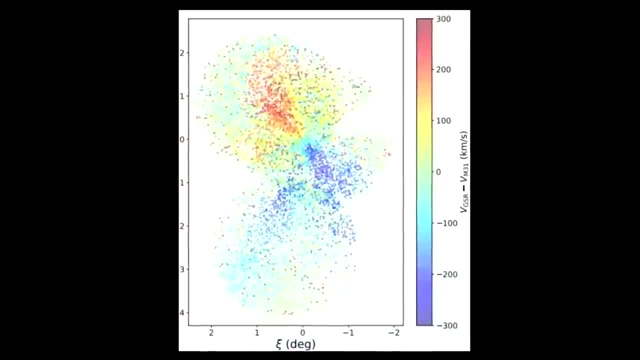 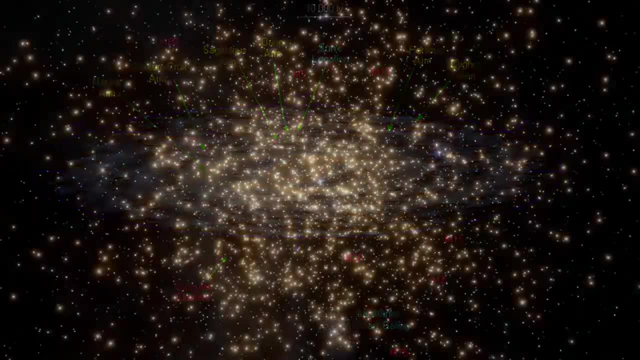 and the third from 10 to 12 billion years. In the Milky Way, for comparison, globular clusters are almost equally old, with an age of 10 to 12 billion years. In the Milky Way, for comparison, globular clusters are almost equally old, with an age of 10 to 12 billion years. 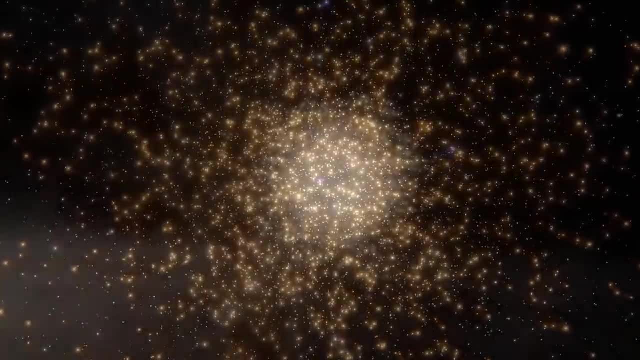 In the Milky Way, for comparison, globular clusters are almost equally old, with an age of 10 to 12 billion years, and there are no young ones at all. The presence of young clusters in Andromeda is probably explained by its voracious appetite. 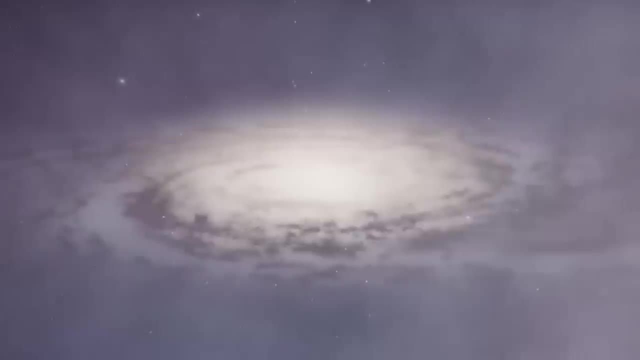 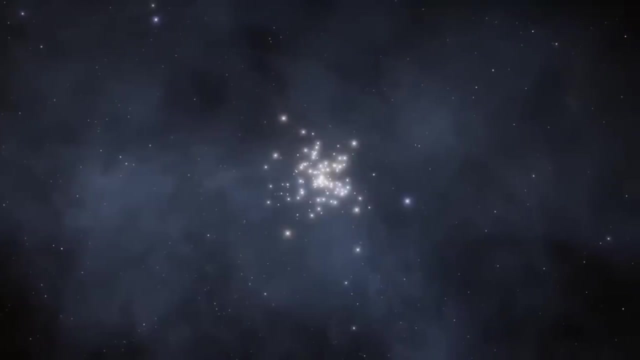 that is, the absorption of irregular galaxies in the past. In addition, there are star clusters in M31 that are intermediate in characteristics between globular star clusters and dwarf spheroidal galaxies, whose analogs have not been found in the Milky Way. 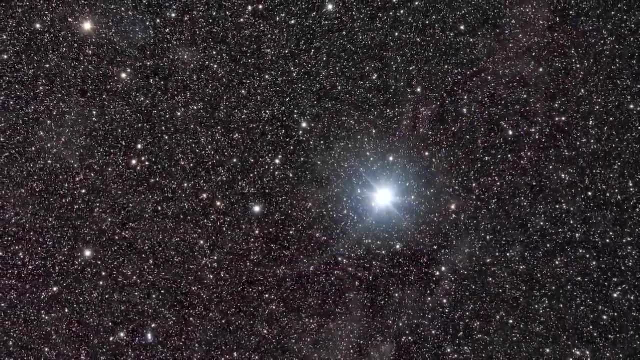 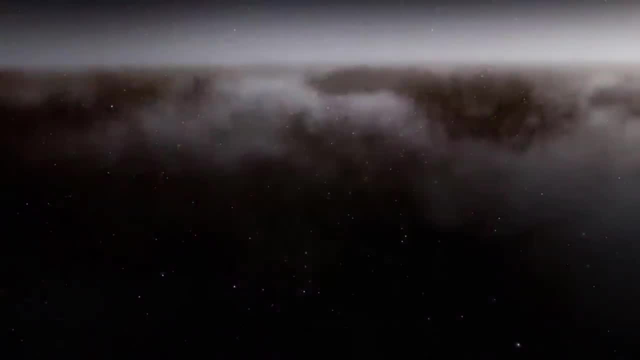 Although their luminosity and colors are the same, they are not the same. Although their luminosity and colors are the same, they are not the same. They differ only in very large radii, about 30 parsecs. They differ only in very large radii, about 30 parsecs. 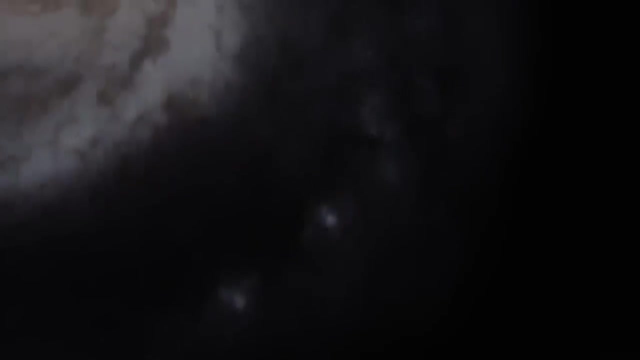 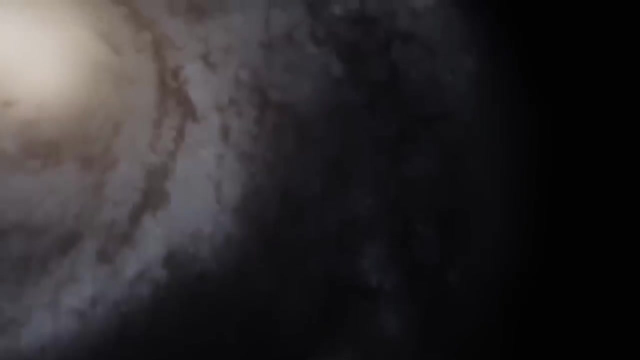 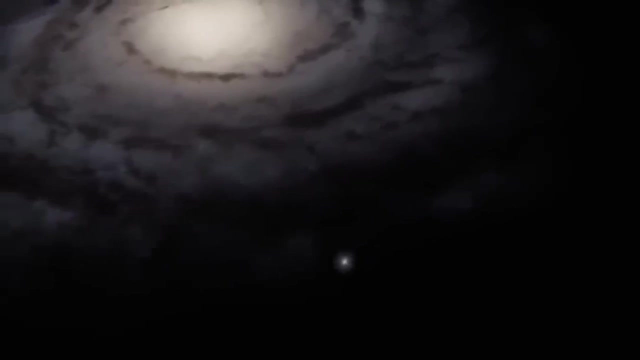 Andromeda's interstellar medium consists of gas with different temperatures and dust, which are enough here for it to be observed in the form of dust bands partially obscuring the light from the northwest side of the bulge. Dust bands- and there are more than 700 of them- are clearly visible due to the large angle of inclination of the galactic plane. 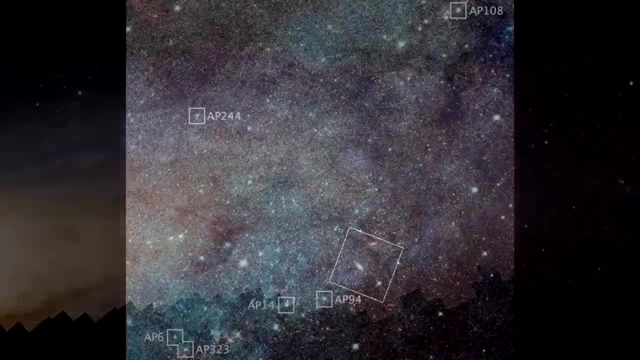 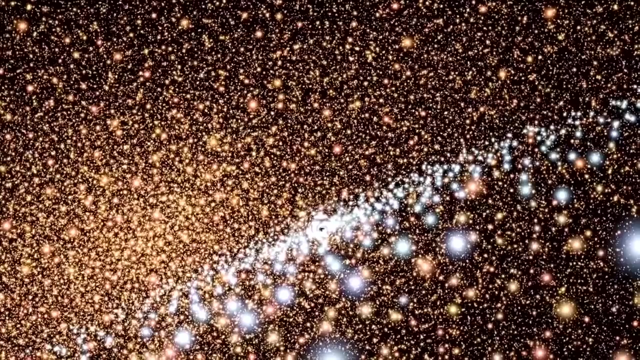 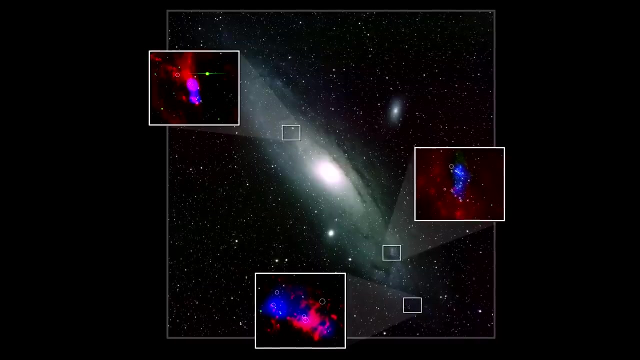 About 4,000 regions of active star formation from ionized hydrogen are known in Andromeda, as well as 26 supernova remnants and 20 more candidates for such objects. In addition to them, more than 4,000 planetary nebulae are known, and there are estimated to be about 8,000 of them in the galaxy. 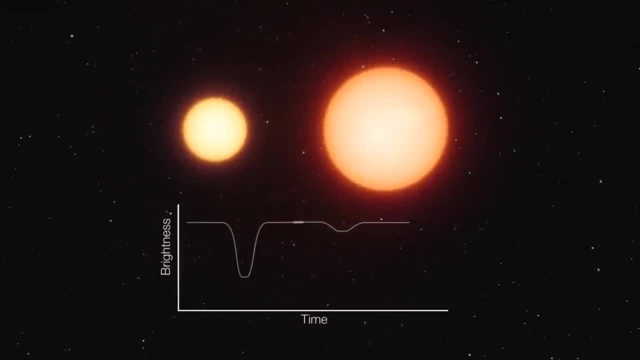 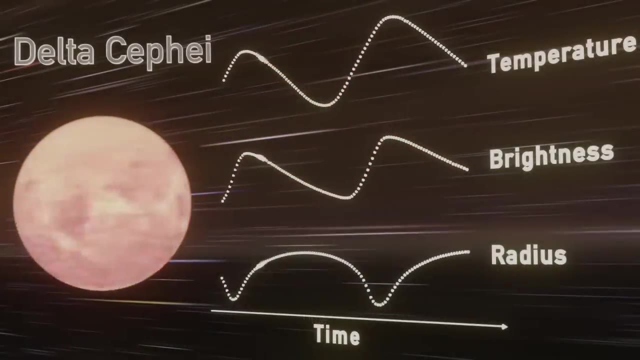 At least 35,000 variable stars of various types have been discovered in M31.. First of all, these are Cepheids, bright stars with a certain dependence between the period and luminosity by which you can determine the distance to them. 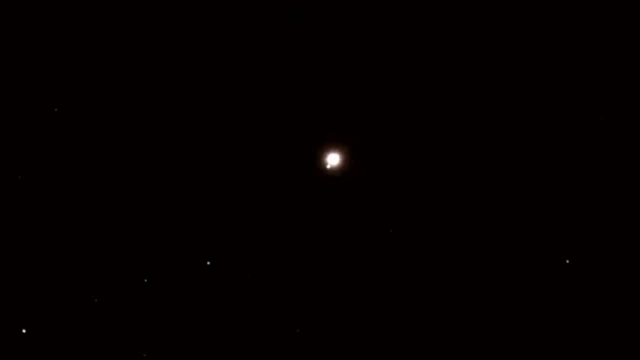 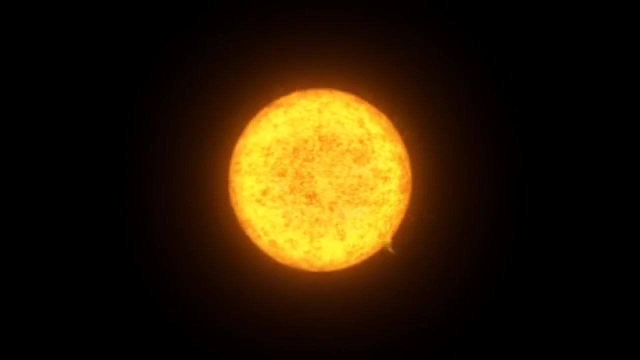 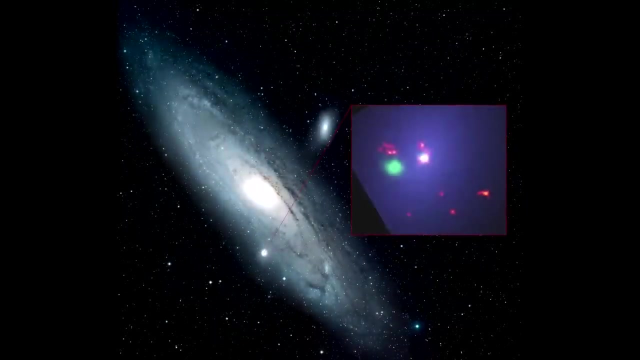 Most Cepheids have a period of 5 to 125 days. Other well-known types of variables include bright blue variables, Lyre-type variables, long-period variables and Ar-type variables of the Northern Crown. On average, about 1,000 stars are known in M31.. 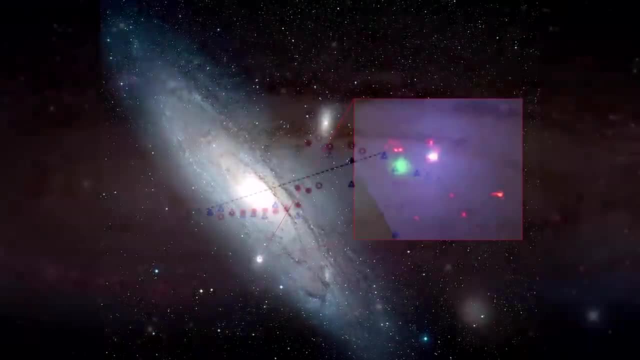 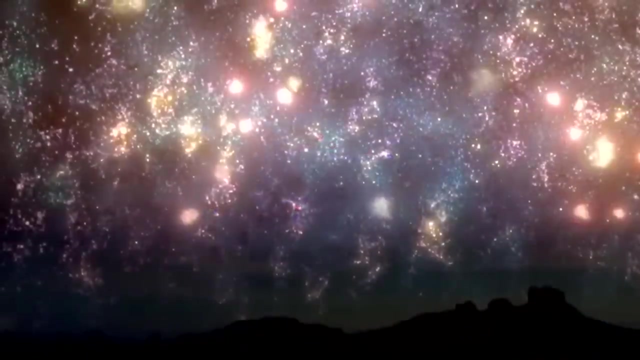 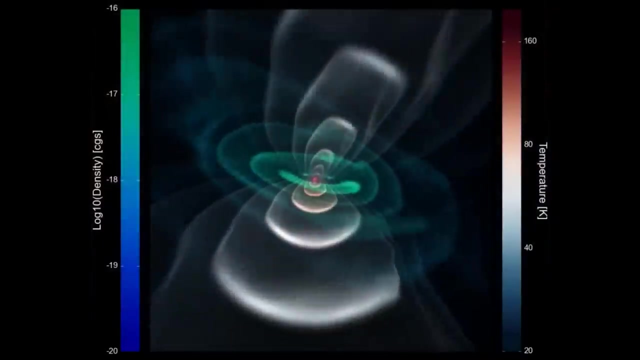 About 50 new stars flare up in the Andromeda galaxy per year, and at least 800 such objects have been registered here. At the same time, the ratio of the frequency of outbursts of new stars to the luminosity of the galaxy is quite low compared to other galaxies, which may be due to the low rate of star formation. 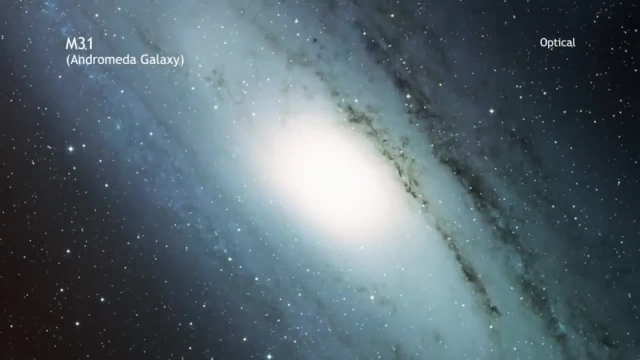 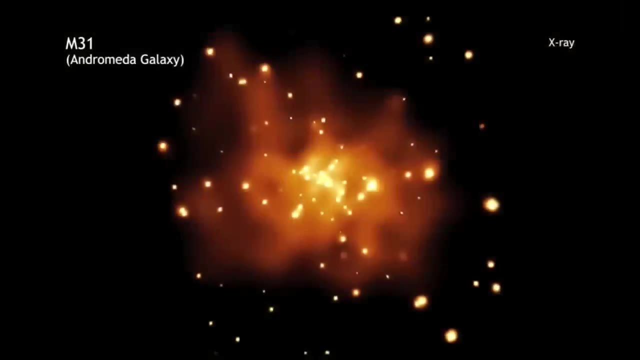 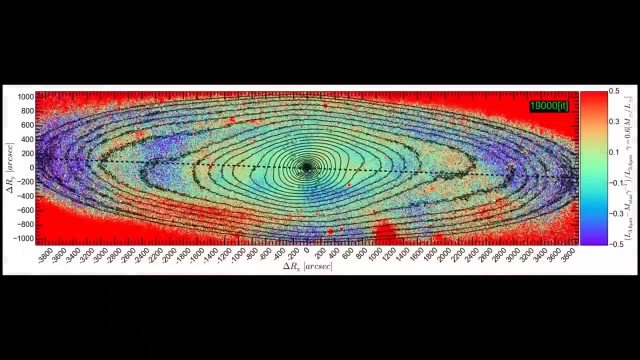 About 2,000 sources of X-ray radiation are also known in M31.. X-ray binaries and supernova remnants, as well as angry stars. Some sources are observed in the globular clusters of the galaxy. The bright cluster M31 is higher in the X-ray range than in the globular clusters of the Milky Way. Another difference between the sources in the Andromeda galaxy and the sources in our galaxy is that they are concentrated in the center. Currently, only one candidate exoplanet has been discovered in M31, the temporary name Pi-H99N2.. But there is no doubt that in the Andromeda galaxy there are millions or even billions of planets orbiting its numerous stars, filled with a lifeless atmosphere or possibly other flora, fauna, organisms and creatures. 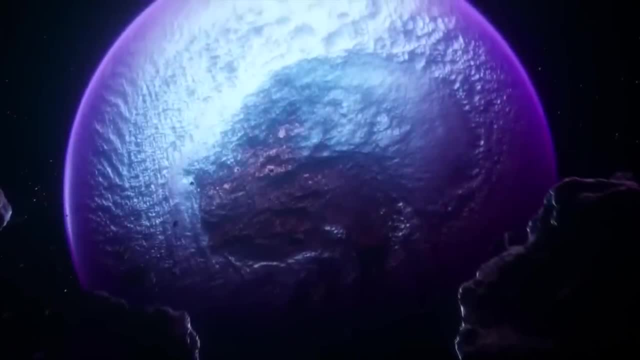 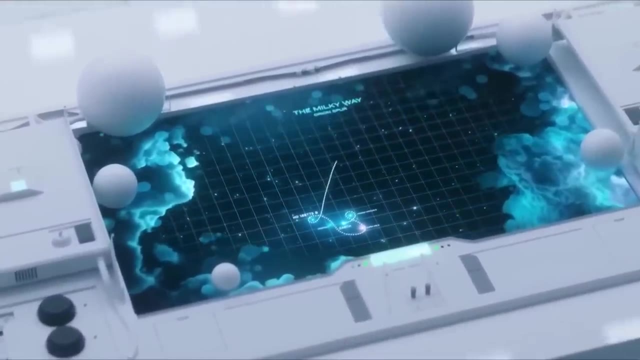 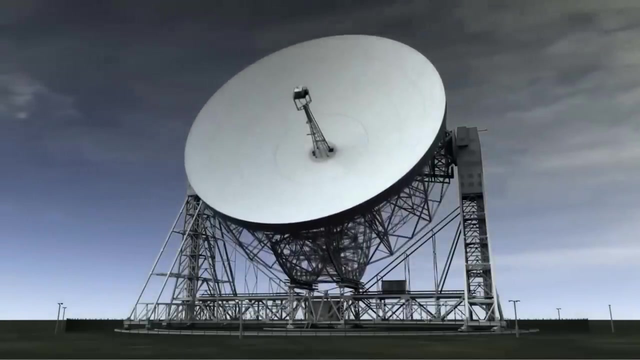 Finding planets outside the solar system is extremely difficult because the planet does not emit light. All exoplanets whose existence has been confirmed are located within our galaxy, But with the development of optical technologies and data processing methods, we will be able to find more planets every year located further in the universe. 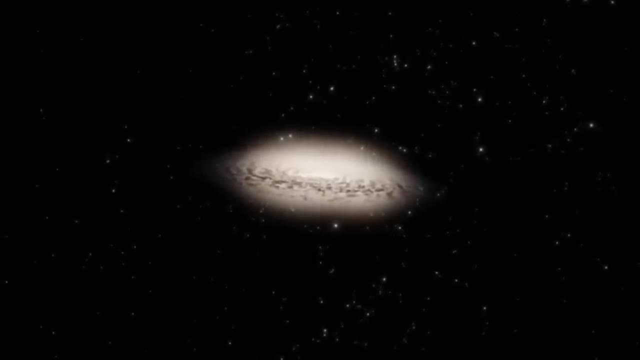 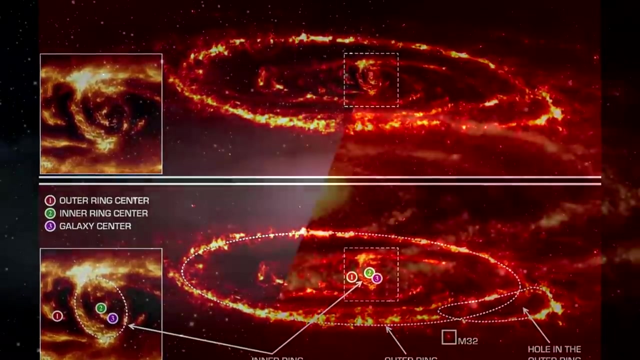 Meanwhile, we have approached the central part of Andromeda, called the bulge, or spheridal densification in stars in the center of the galaxy, as well as the brightest part of the spherical subsystem of the galaxy. This image, taken by an orbiting telescope, shows the crowded 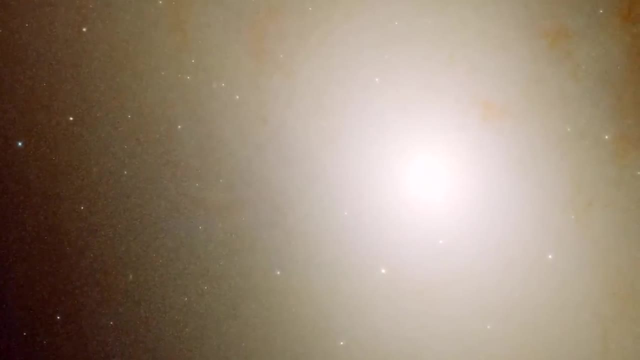 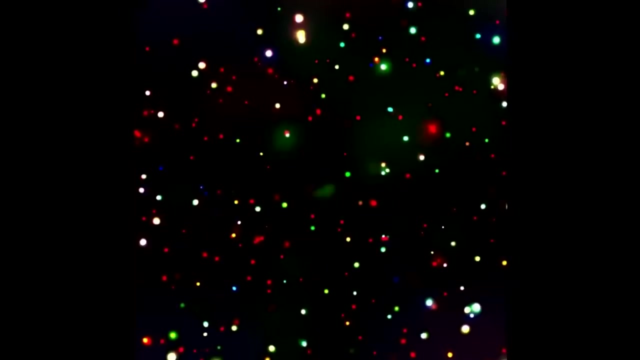 like a space bus and very bright central region of the Andromeda galaxy. The bright dot to the right of the center is a group of stars located around the galaxy's black hole. The blue dots scattered throughout the image are ultra-blue stars that prematurely shed their outer layers of matter, exposing extremely hot cores. 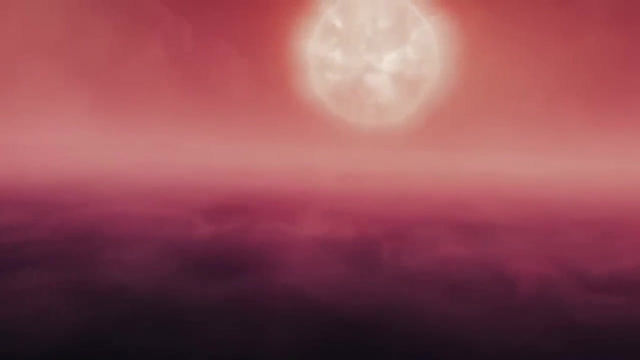 It is likely that there are many other similarly hot stars in this central part of Andromeda that are in earlier stages of their lives. It is likely that there are many other similarly hot stars in this central part of Andromeda that are in earlier stages of their lives. 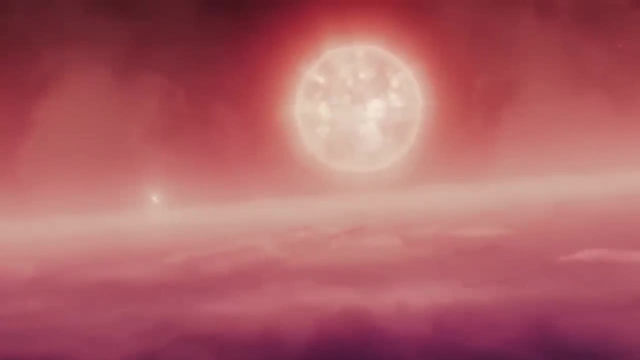 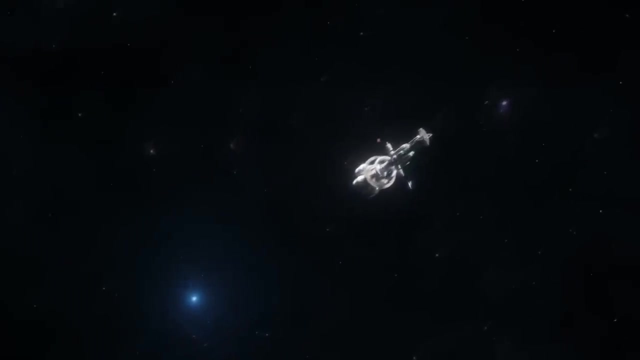 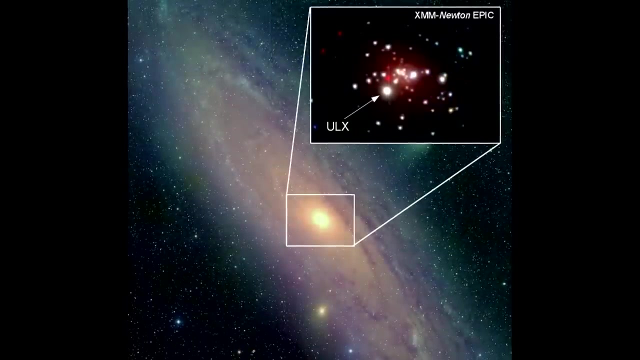 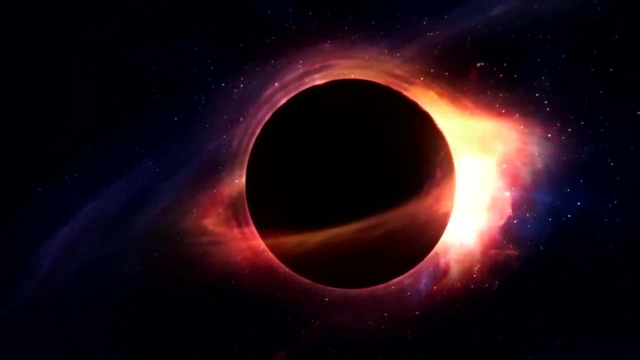 But they are too dim for us to detect them right now. On our journey through the Andromeda galaxy, we have come close to its very heart. This image shows the clearest image of the galaxy's core ever taken in visible light. A supermassive black hole with a mass of more than 100 million solar masses is located in the center. 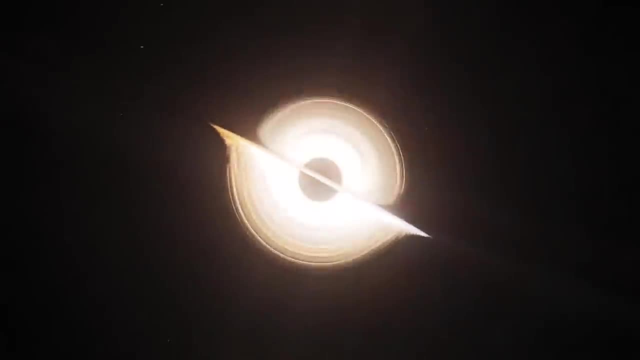 Event horizon. The nearest area around the black hole where light savvyady has been located is known as theicopter. The nearest area around the black hole where light savvyady has been located is known as theicopter, where light can still penetrate, is too small to be seen, but it is located near the center of a. 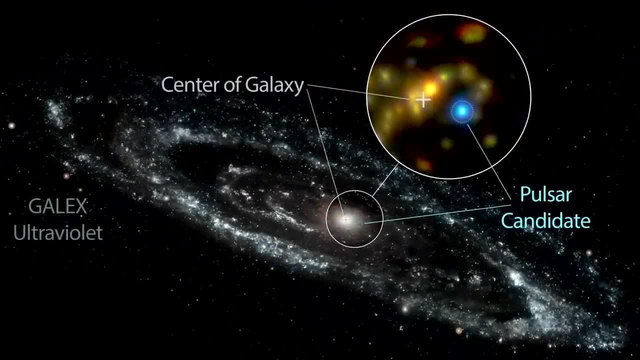 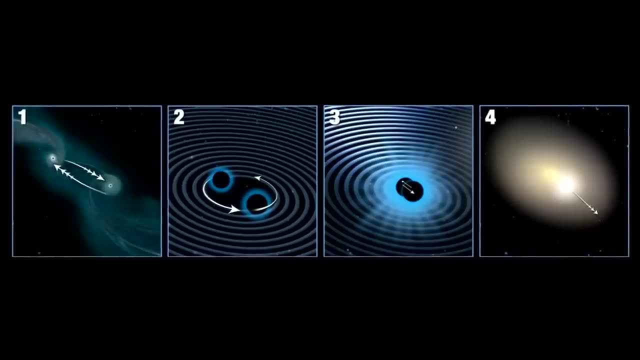 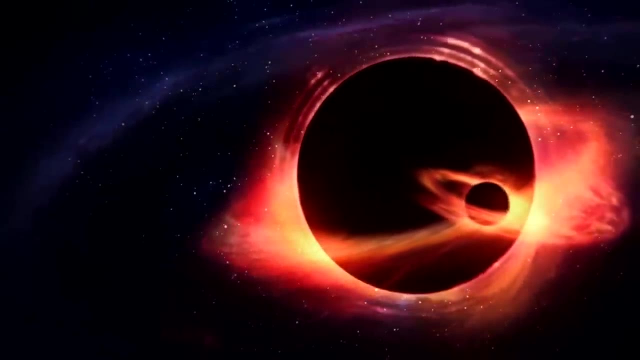 compact cluster of blue stars in the center of the image, A compact cluster of blue stars surrounded by a larger double core, M31.. A double core is an elliptical ring of old reddish stars orbiting a black hole, but more distant than blue stars When the stars are at the farthest point of their orbit. 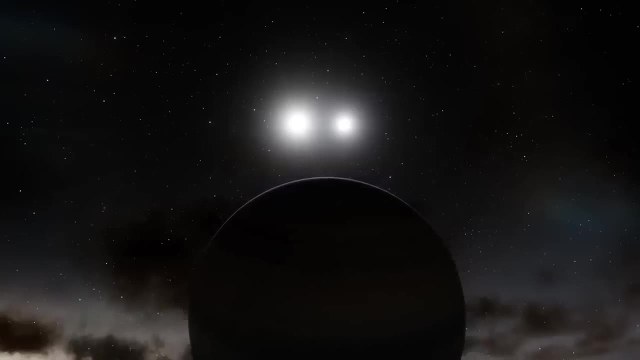 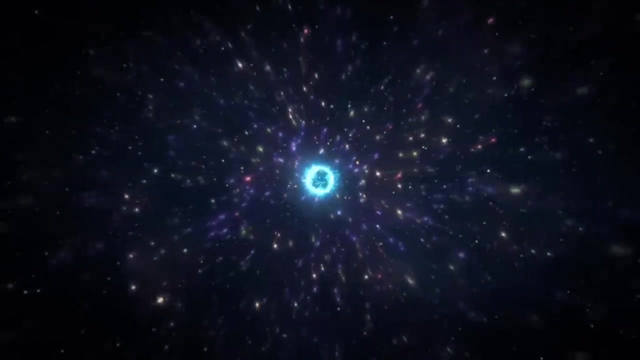 they move slower and create the illusion of a second core. The age of the blue stars surrounding the black hole does not exceed 200 million years, so they must have been formed near the black hole as a result of a sharp burst of star formation. 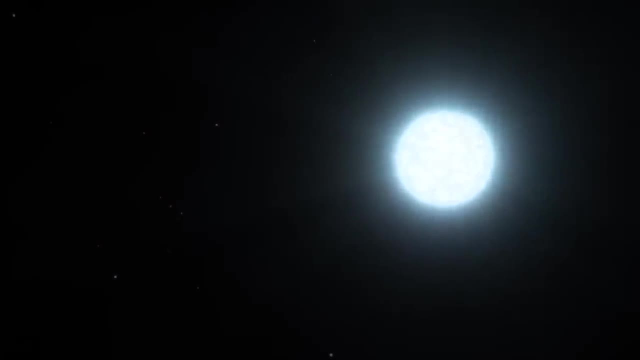 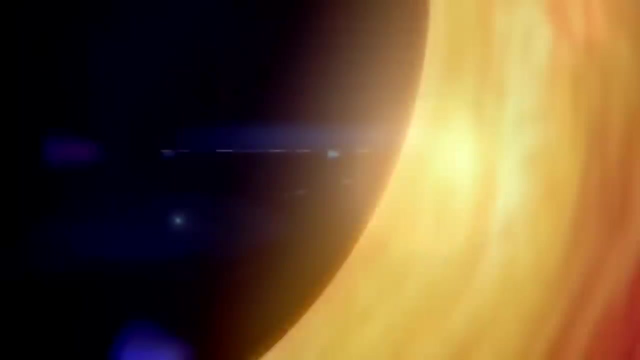 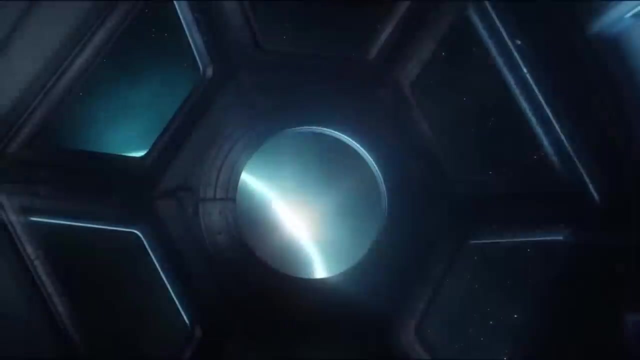 Massive blue stars are so short-lived that they would not have enough time to migrate to a black hole, if, of course, they formed elsewhere. Astronomers are trying to understand the relationship between the two stars. They understand how apparently young stars formed so deep inside the gravitational grip of a black hole and how did they survive in such an extreme environment at all. 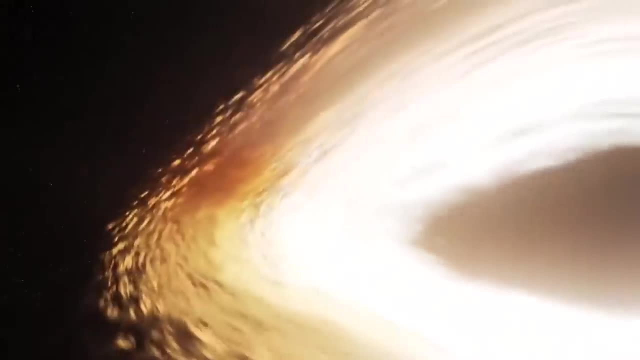 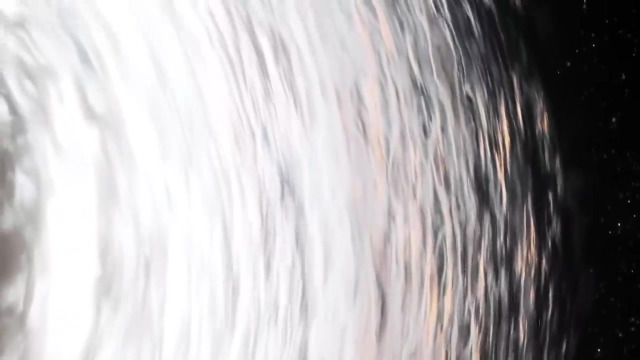 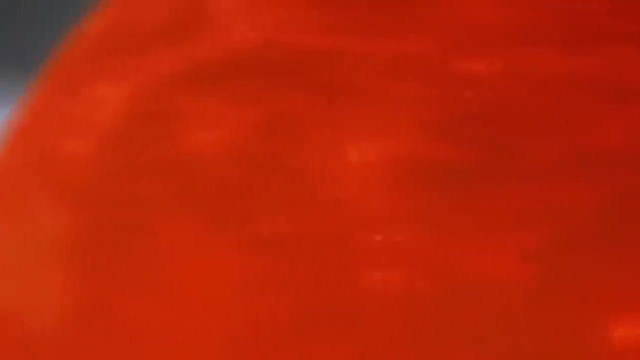 As we delve deeper into the mystery that is the black hole at M31, its enormous size, power and complexity are revealed, giving us amazing insights into its fantastic role in shaping the cosmic landscape. Its irresistible gravitational force not only attracts stars, but also makes them more and more powerful. 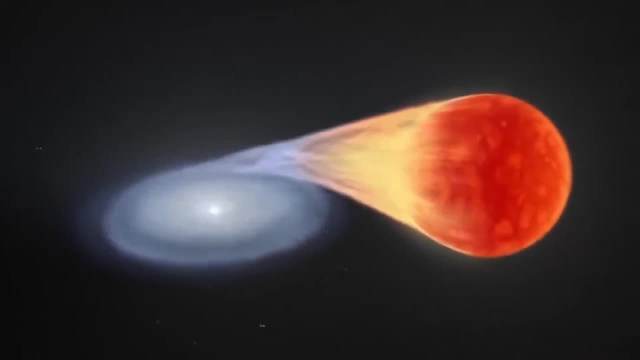 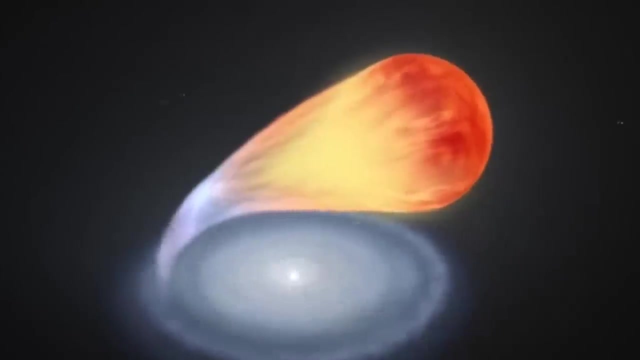 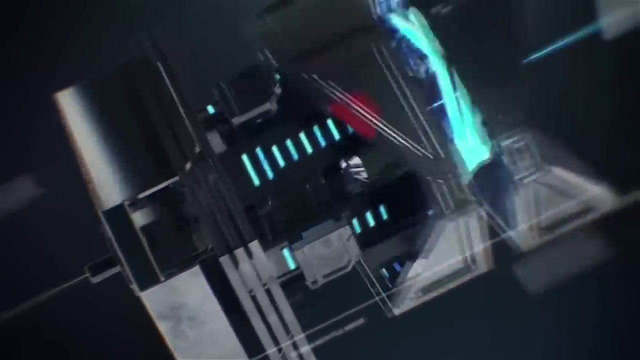 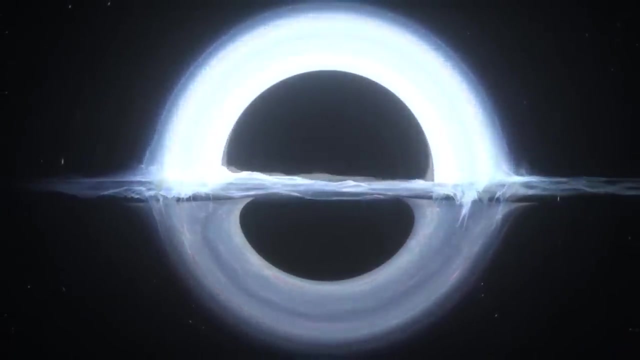 It has massive energy, iron, gas and dust, but also forces them to move in an orbit in spiral to the event horizon, an invisible boundary where nothing, not even light, can escape its capture. As technology advances and our ability to explore the universe expands, the supermassive black hole at the center of the Andromeda galaxy will become an even more exciting object for scientific research. 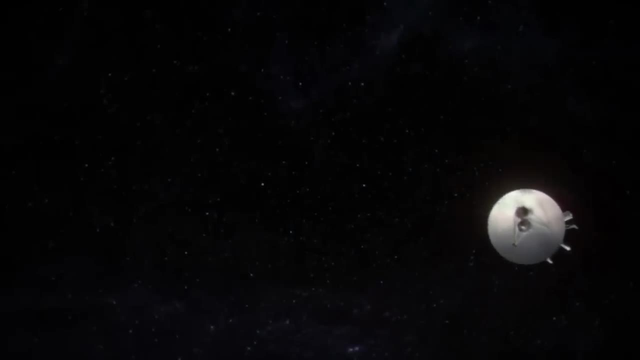 As we continue to unravel its mysteries, this complex and profound scientific research will become even more exciting for us. We will continue to discover the mystery of the black hole at the center of the Andromeda galaxy. cosmic miracle will undoubtedly be a beacon of knowledge for many generations of astronomers. 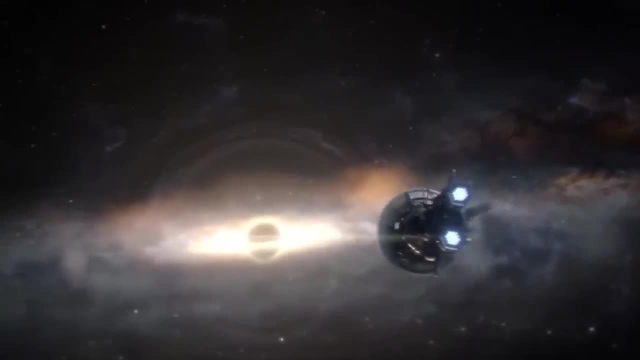 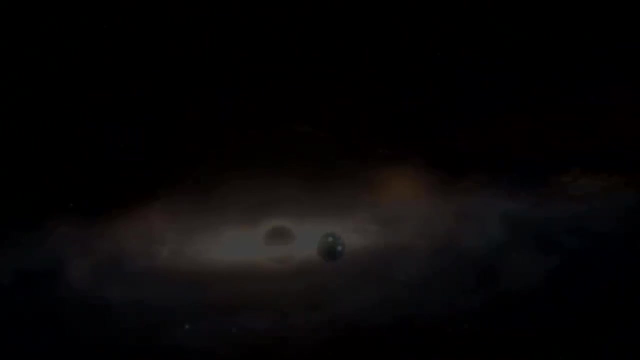 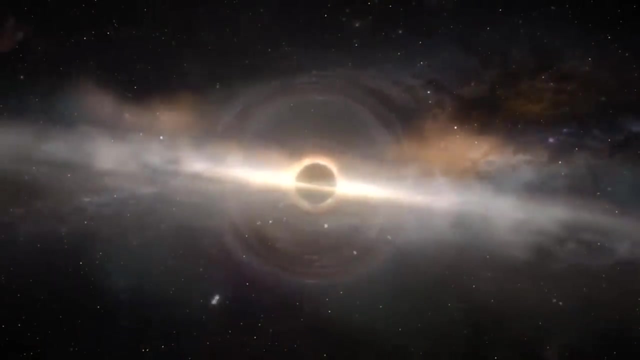 and enthusiasts, But our goal is to dive into the black hole of this galaxy, possibly by sending an umbrella there, A moment and the device disappears from the radar. Nice try, It seems. our journey has come to an end. Today, we crossed the vast expanses of space in the Andromeda galaxy. 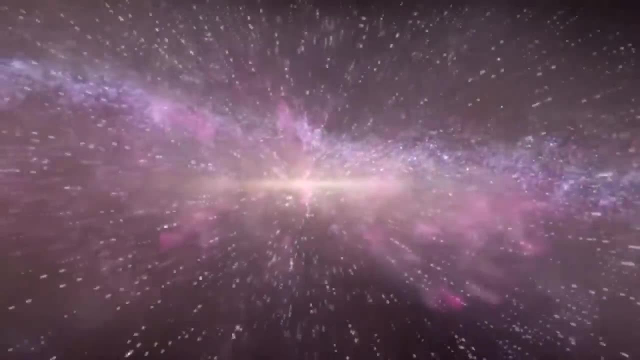 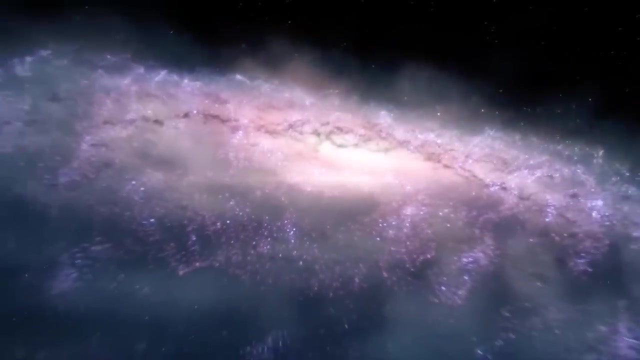 encountering wonders that are difficult to imagine: Supernovae emitting unearthly light, nebulae swirling like heavenly smoke, newborn stars emerging from their gaseous manger and, of course, a huge, supermassive black hole playing the main part in the symphony of cosmic. 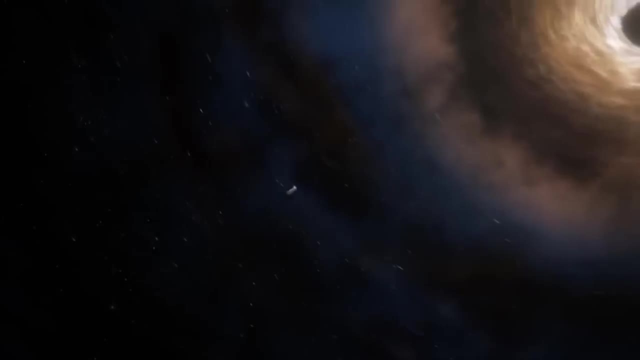 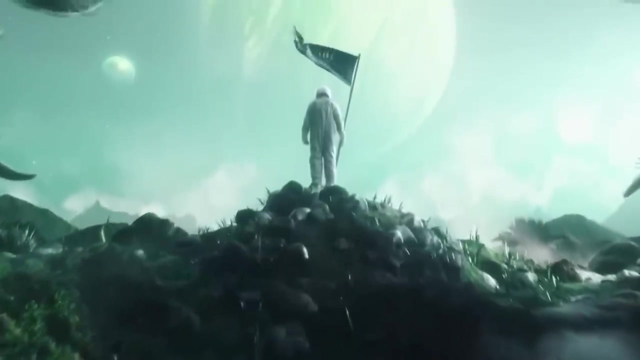 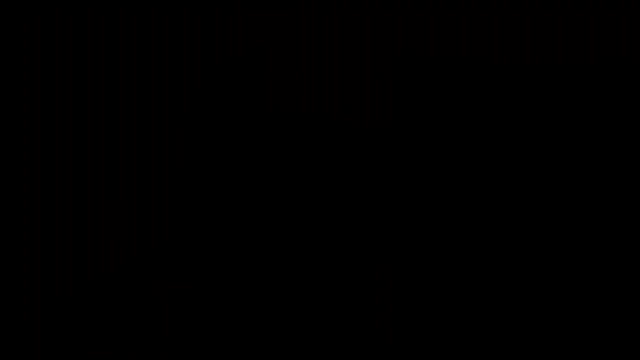 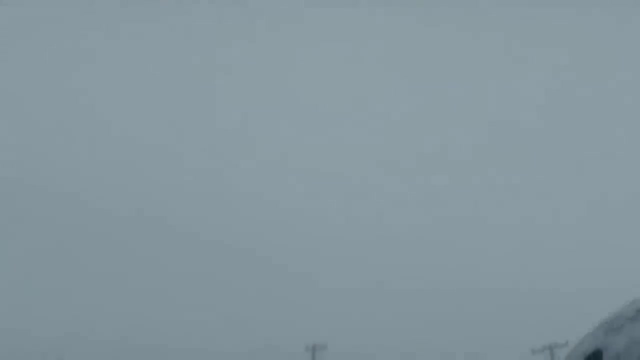 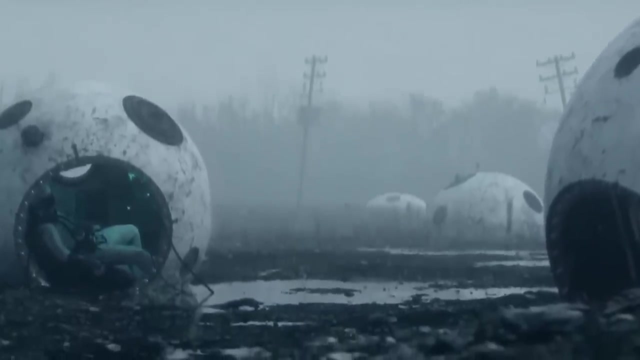 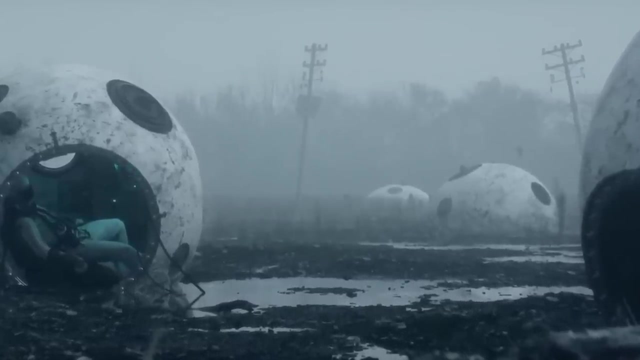 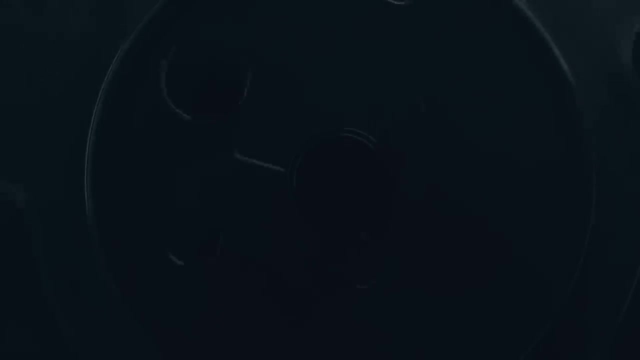 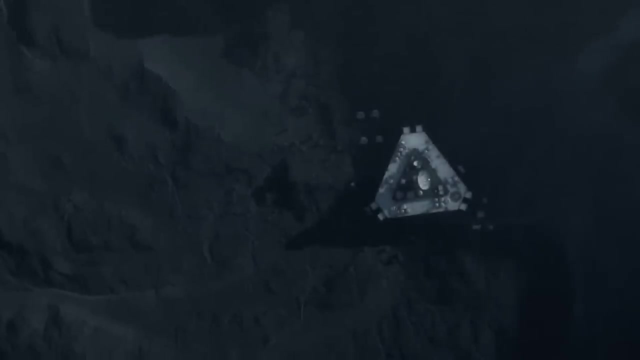 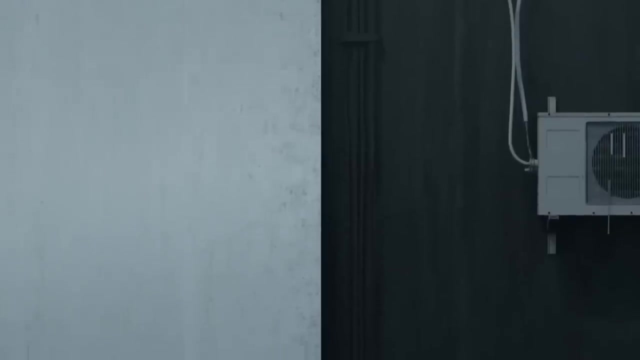 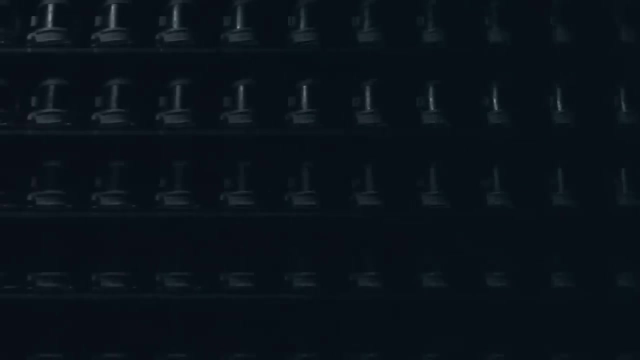 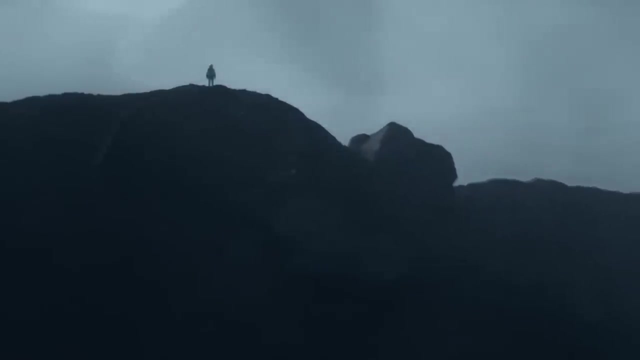 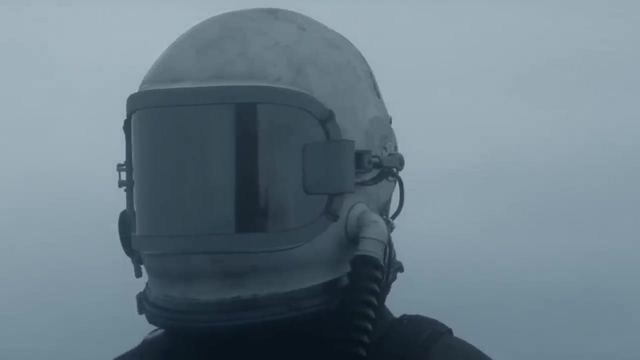 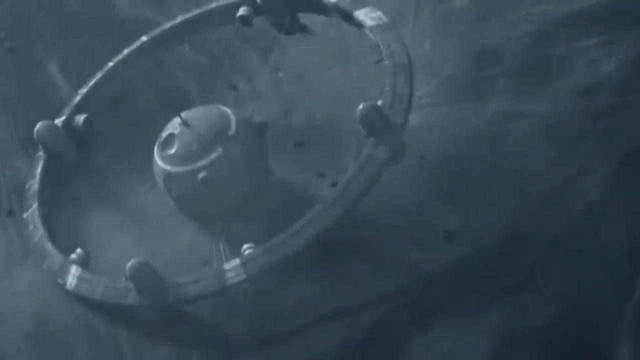 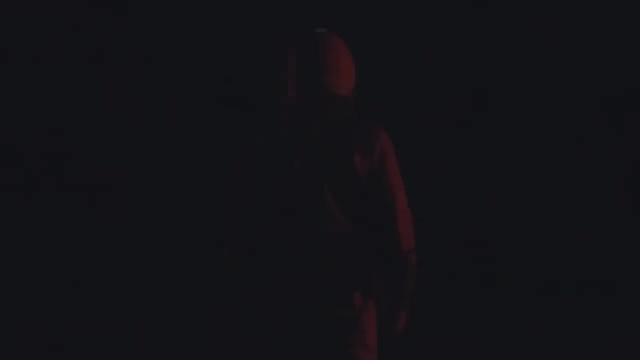 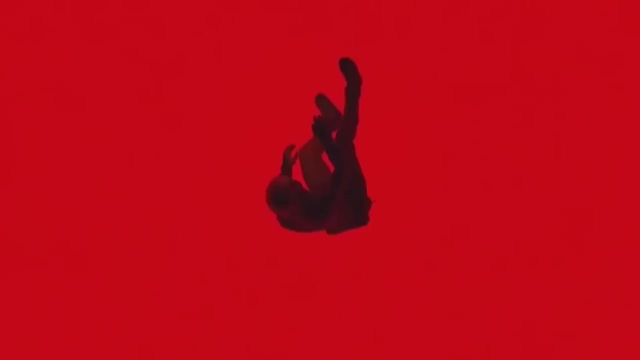 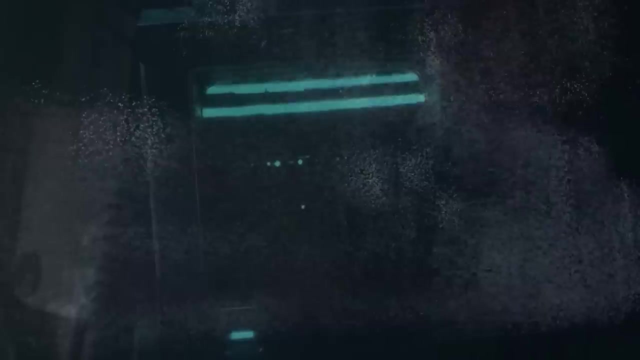 evolution. The journey to the center of Andromeda was just the beginning and we are ready to chart a new course for the next great adventure and new day Discoveries. It is well known that our universe has dimensions, or a number of position. 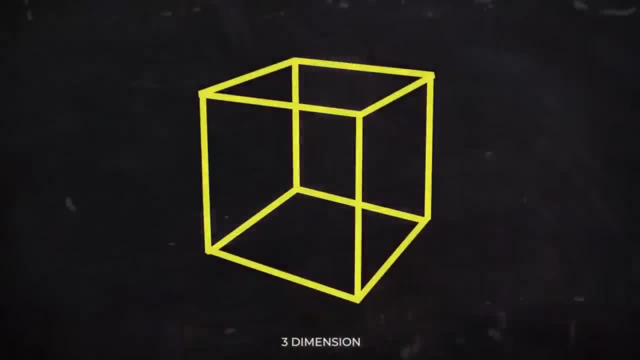 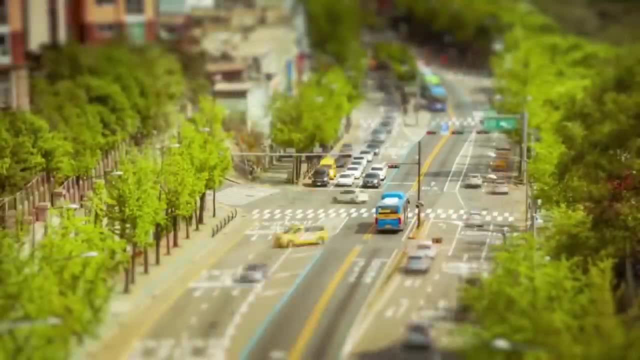 coordinates by which it can be measured: Length, height and width. In other words, These are measurements that put bounds on the universe that is known to us. Multi-dimensional space turns out to be more concentrated in terms of informational and energy capacities. 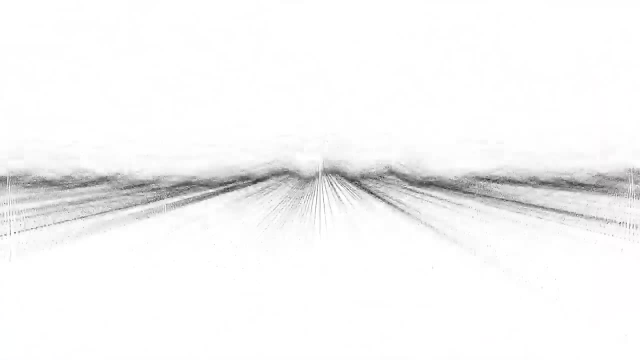 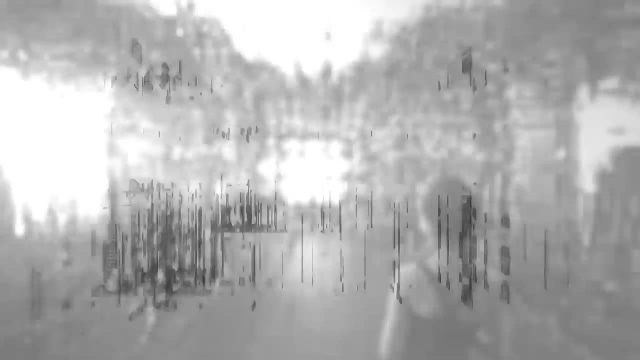 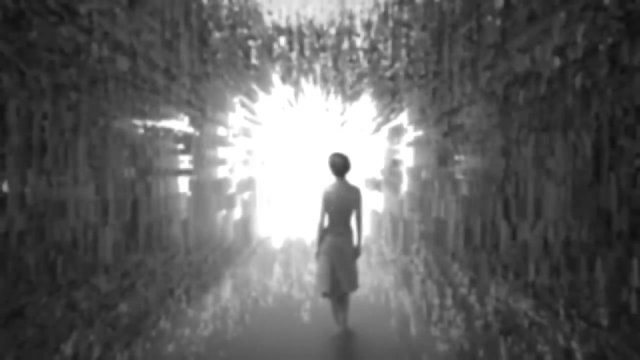 At one point of space. a higher dimension may be the concentrated information of all the other layers of reality of the lower dimensions. Is it possible to discover that most inaccessible fourth dimension, And what does contact with it change in our world? If we ponder it for a while, we may possibly succeed in finding the answers. 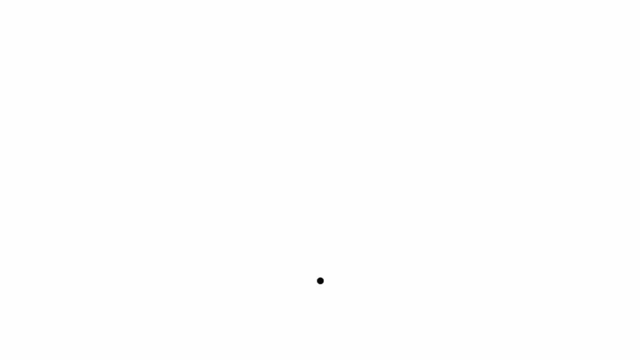 Simply stated, if you place a cube in front of you, then you won't see its backside, since vision is two-dimensional. If the cube begins to rotate, then the brain analyzing it will understand that it is a cube and that there is a backside. 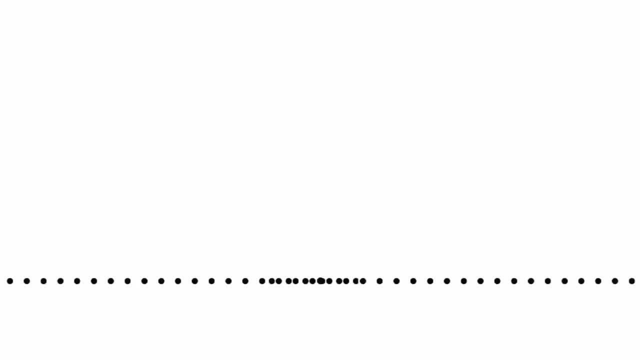 But what our brain knows is one thing and how it is seen by the eyes is another. If our vision were three-dimensional, then we would see the cube simultaneously From all sides, like a scanner at an airport. We would see all of space in its entirety and nothing could be hidden from us. 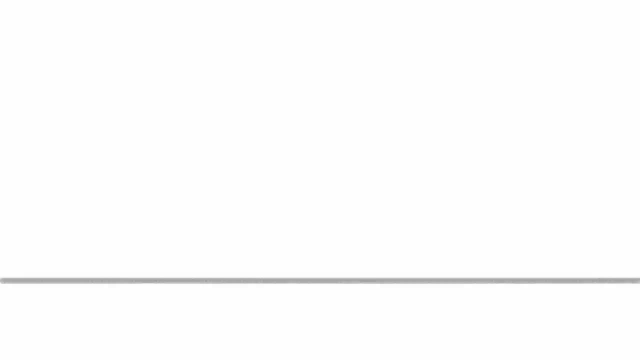 That is to say, we must observe from without, as if we are watching a movie, or even our own dream, in which we can sometimes evaluate ourselves from the sidelines. Indeed, if we were to live in a two-dimensional space on a flat plane, we would have to stretch our imagination considerably in order to think of how to move a rectangle off of the flat plane. 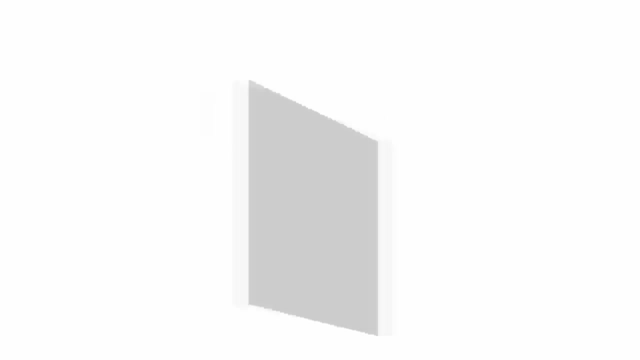 Well, conceptualizing a four-dimensional space is also quite difficult. for us, A three-dimensional space is a space in which the position of a point is designated, as we have already said, by three numbers. For example, the position of an aircraft is indicated by longitude, latitude and altitude above sea level. 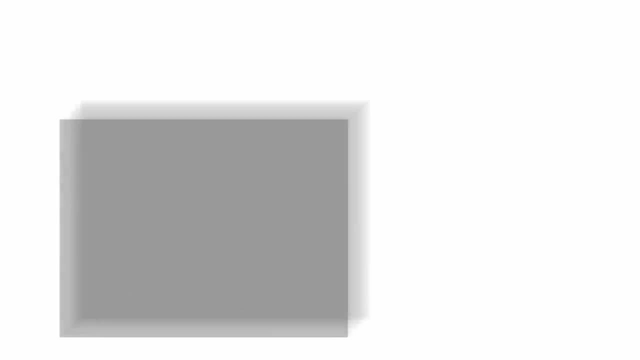 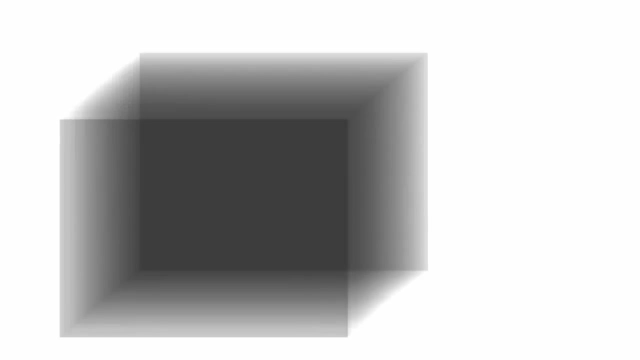 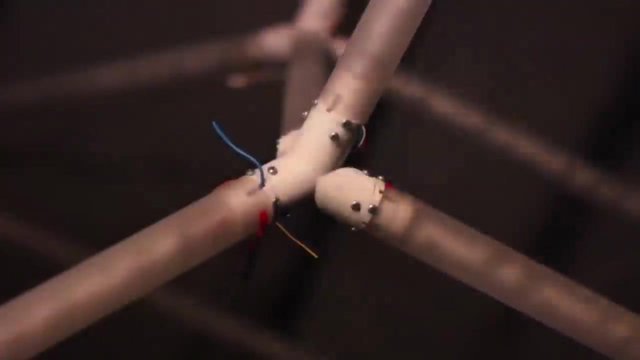 In a four-dimensional space, an object corresponds to a four-number coordinate. A four-dimensional cube is obtained by sliding an ordinary cube along in a particular direction that doesn't lie within our three-dimensional space. Where this direction is or how to transcend our limits, is difficult to say as well as to perceive. 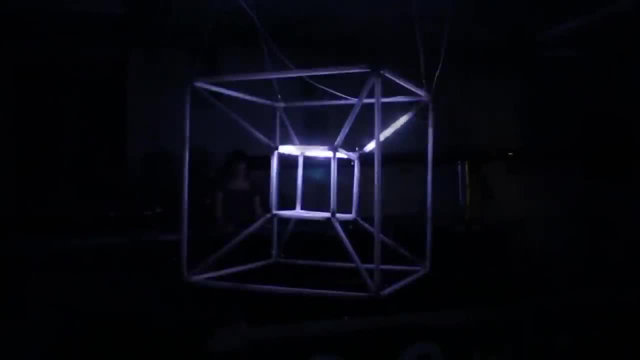 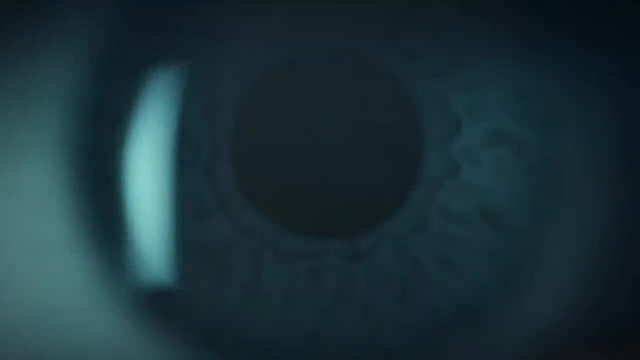 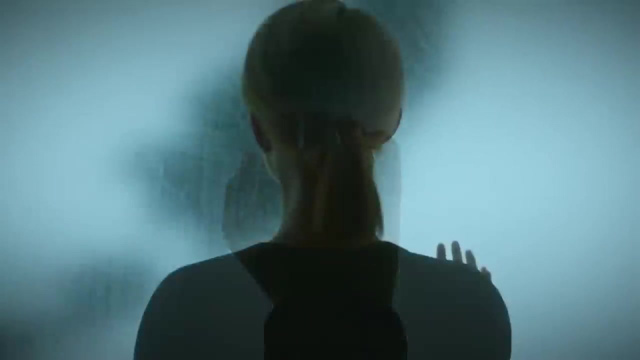 But use your imagination and indulge in fantasy, and why not? Often this type of four-dimensional cube is called a tesseract, the equivalent of a usual three-dimensional cube generalized in a four-dimensional space. Try to picture the properties of a hypothetical 4D space. 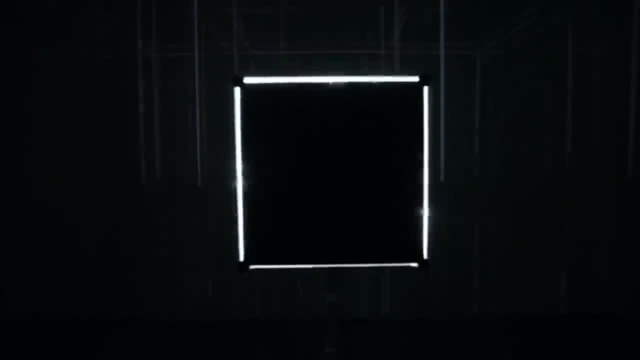 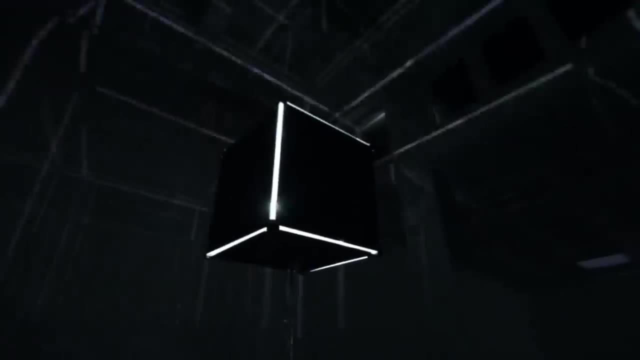 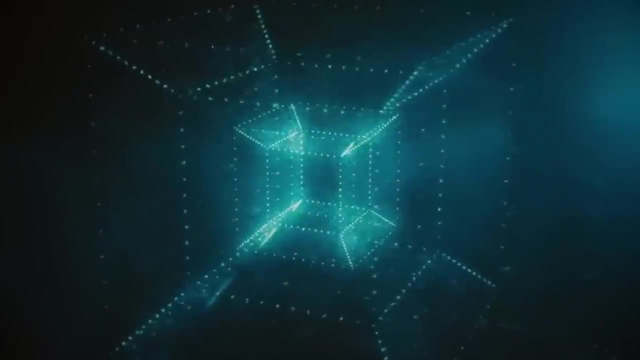 To begin with, we need to understand if a fourth orthogonal axis is feasible in the coordinate system and, if so, where is it located? Indeed, for us, our familiar three-dimensional space is associated with three axes of the coordinate system, And if we can't even imagine something that is, 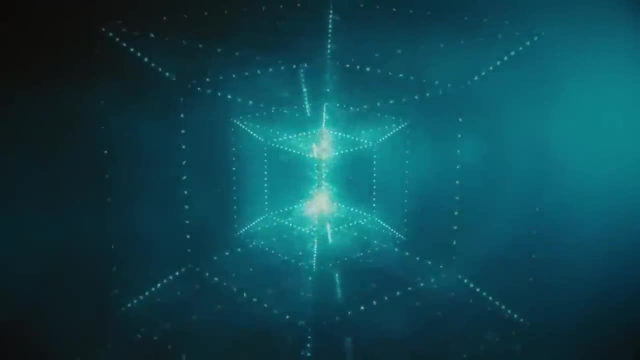 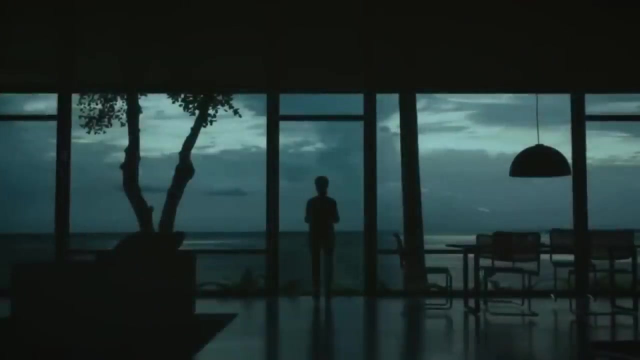 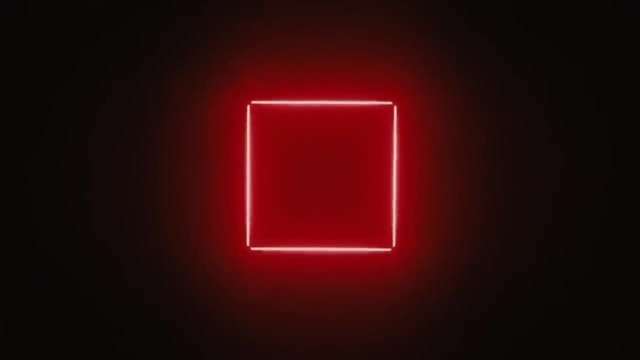 if we can't mentally create its corresponding image, does that then mean this something does not exist, It appears, so. This poses the question: why exactly are there three spatial dimensions? no more and no less? It is apparent because the atom, and along with it all the rest of matter, has precisely three spatial characteristics. 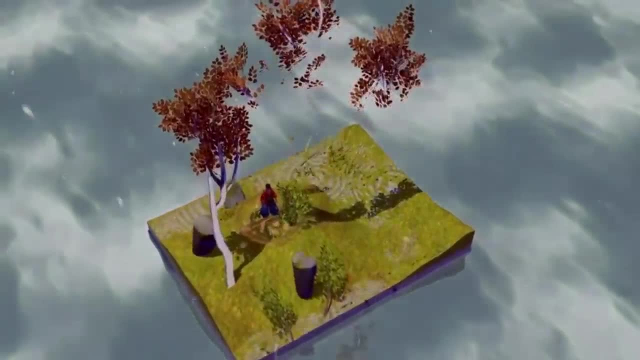 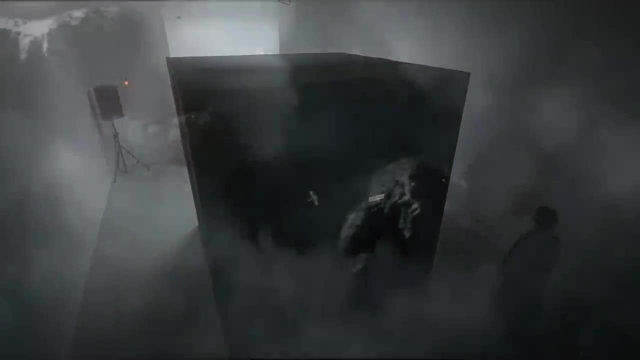 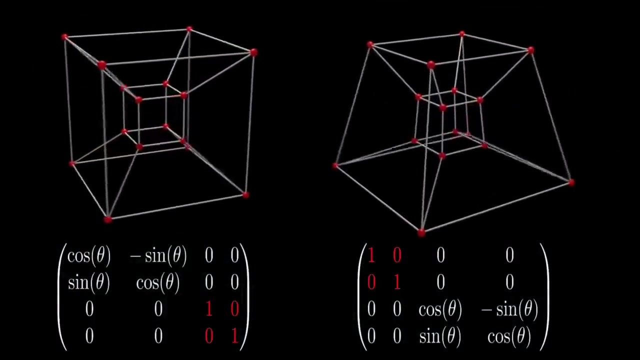 length, width and height. What characterizes these three attributes of space? Naturally, the spread of tangible objects in three possible directions: Forward-back, left-right, up-down- The usual pattern for a kangaroo. Is it possible to see something from the fourth dimension? 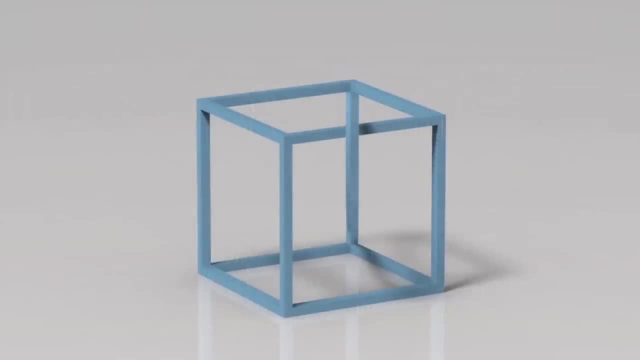 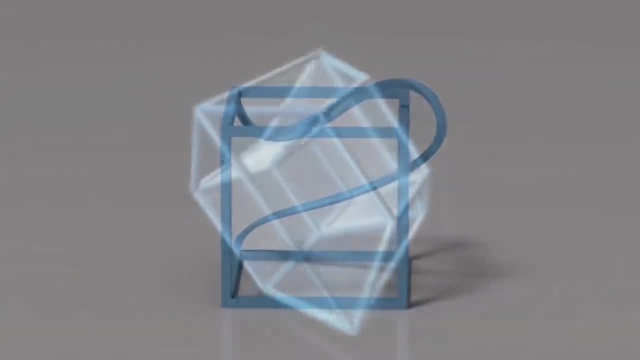 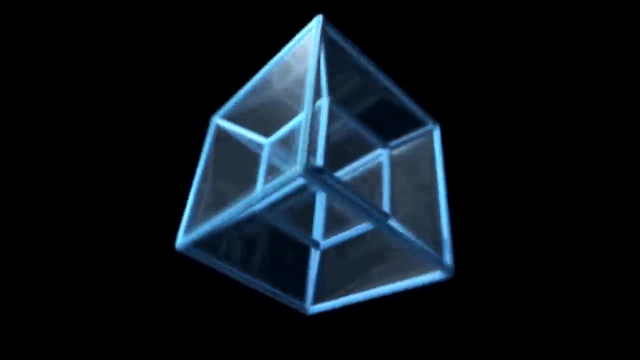 Most likely, yes, But it will only be a projection, a part of what it really is. That is, for inhabitants in a one-dimensional existence, a line, any two-dimensional beings would be perceived merely as complete objects. They are perceived merely as component parts of one dimension. 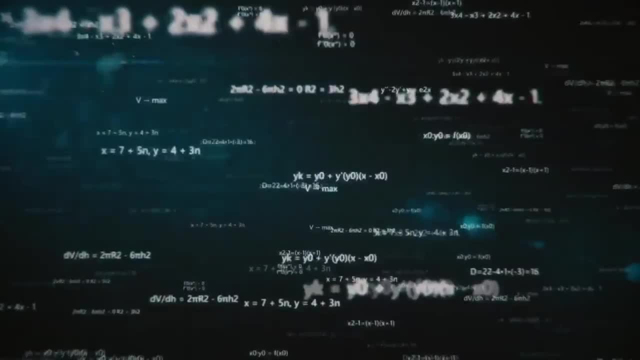 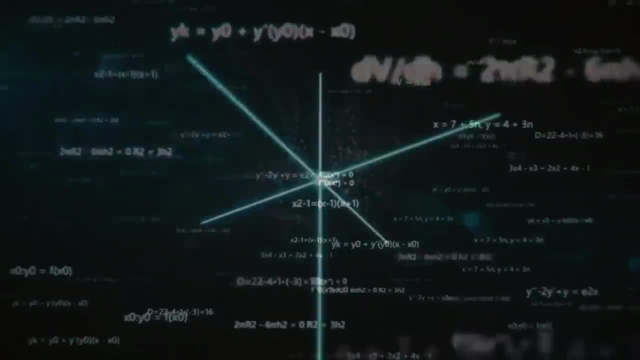 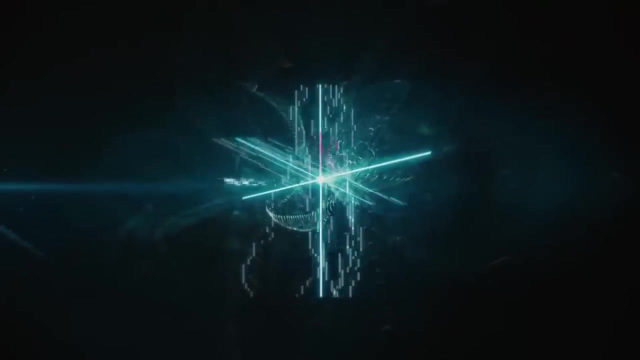 Whatsoever transcends the bounds of this dimension won't be noticed, as the eyes are already out of the picture. In the same way, the inhabitants of a two-dimensional space- a flat plane- can see the inhabitants of a three-dimensional space only in the form of their two-dimensional imprints or projections. 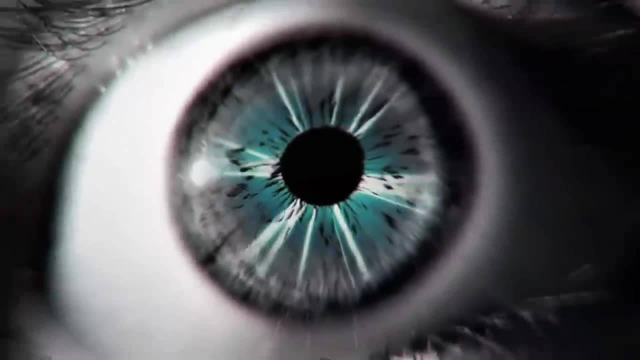 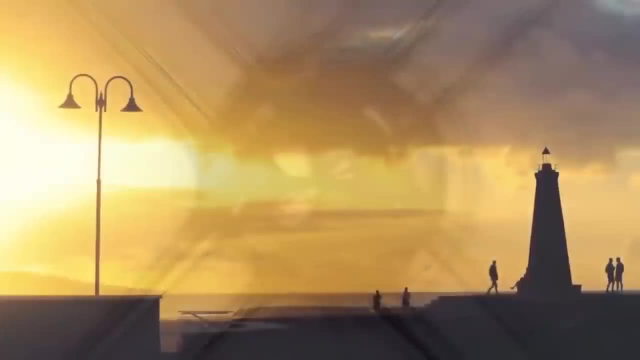 They also simply don't see anything in the third dimension. This means if one were to end up in this two-dimensional space, then in the best-case scenario, the local inhabitants of the flat plane would become acquainted with his footprints and, in the worst case, his cross-section. 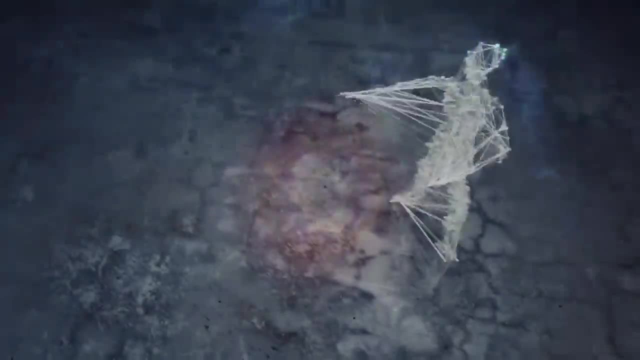 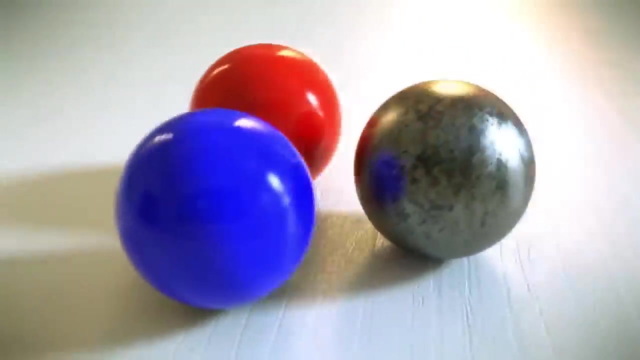 But if a fourth dimension does exist, then what would creatures or life look like on another world? In order to answer this question, we need to imagine: how would the space of our world change if it became four-dimensional. It's logical to assume. 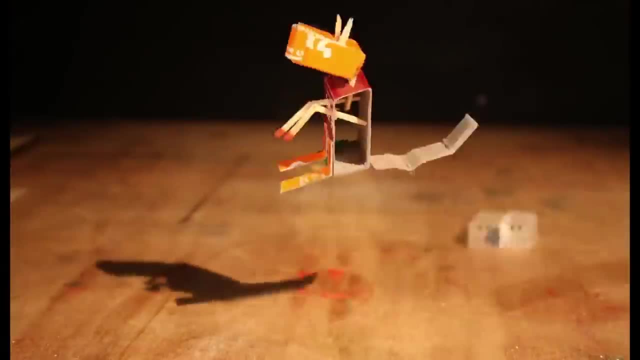 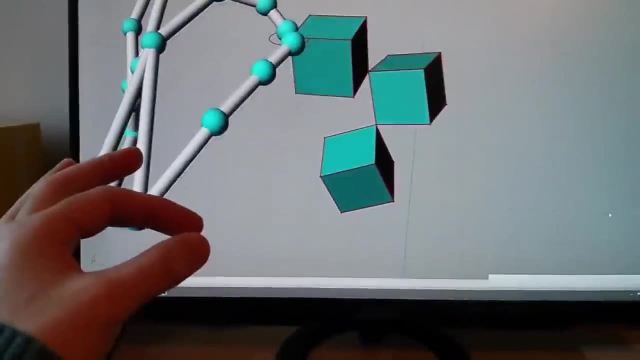 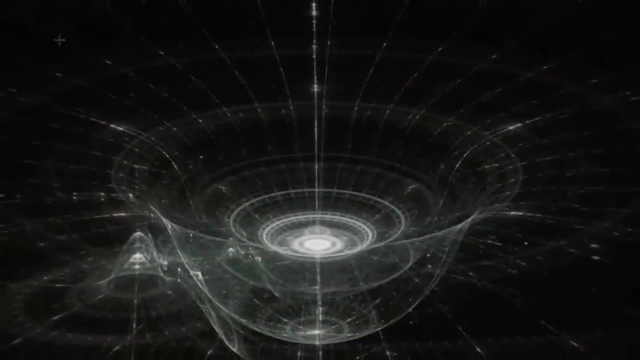 that an additional side would appear in which movement is possible and a restructuring of configuration at an atomic level would begin. The electrons around the nuclei of atoms, having received an unrestricted new side, will begin to rotate in the fourth direction. The nucleus of the atom will also be restructured. 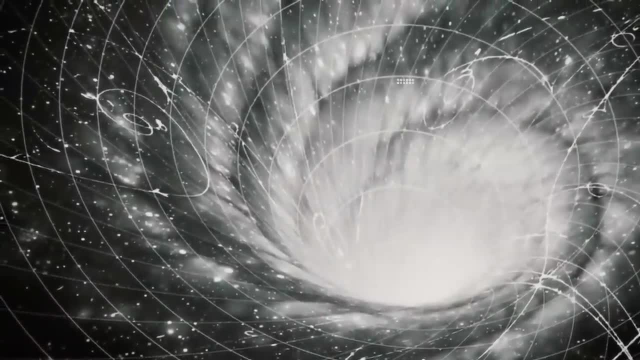 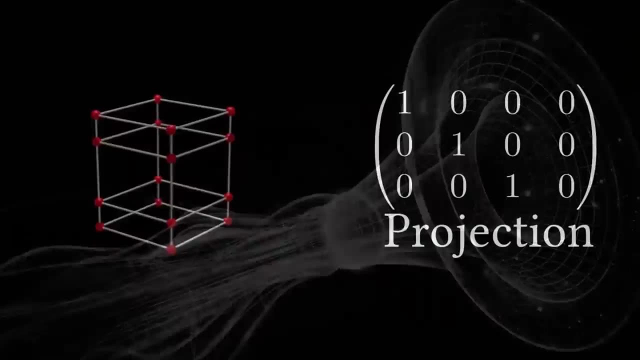 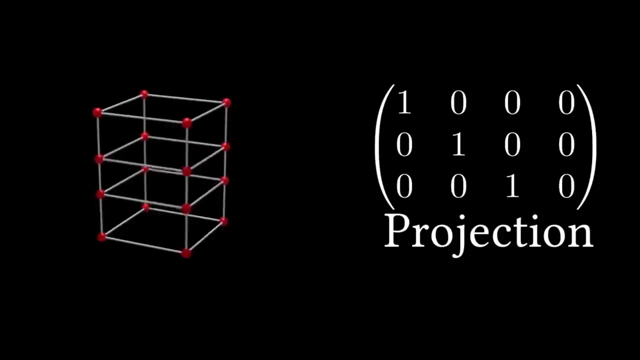 and the chemical properties of the elements will change, which of course will fatally split all forms of 3D life. Meanwhile, after the restructuring of atoms in the fourth dimension, our planet Earth will be only one atom in thickness, but the Earth's mass will remain the same as it was in the three-dimensional space. 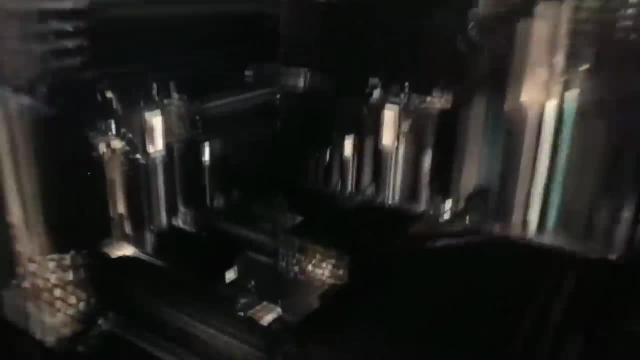 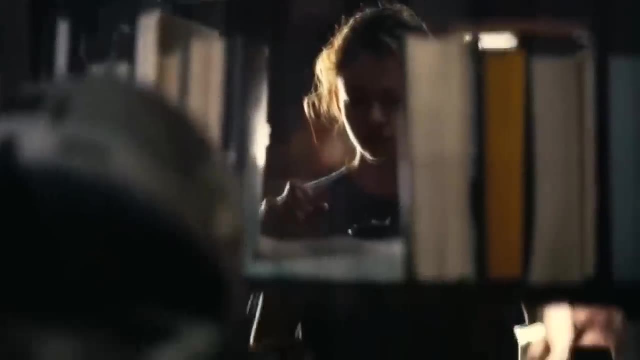 due to which it will collapse in the fourth dimension under the weight of its own mass and, in the end, form a four-dimensional hypersphere. The same will happen to the Sun and the other planets and stars. Gravity will begin to spread out into the new direction. 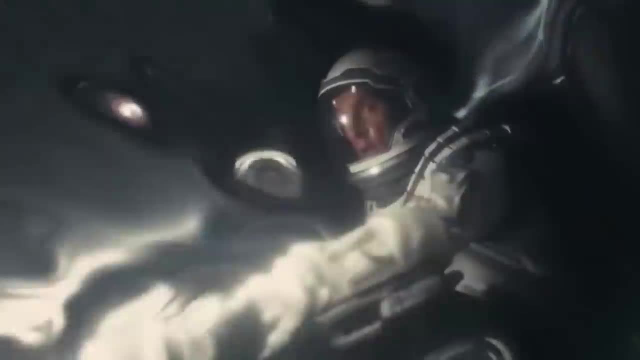 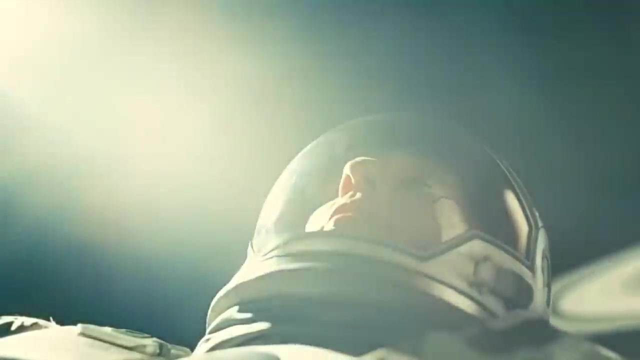 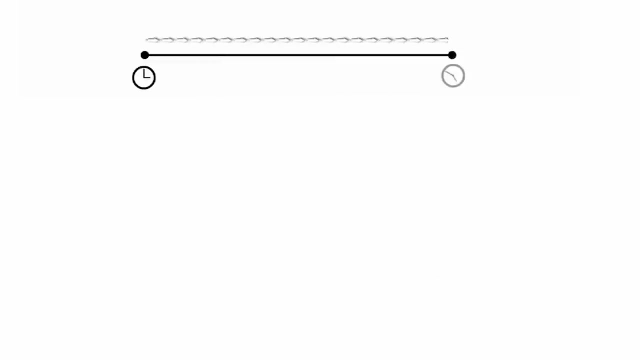 due to which there will be a chaotic change in the orbits of all of the celestial bodies in the entire universe. Ultimately, after a catastrophic restructuring, everything will stabilize and there will be a new universe. True, nothing living on it up to that moment will remain. 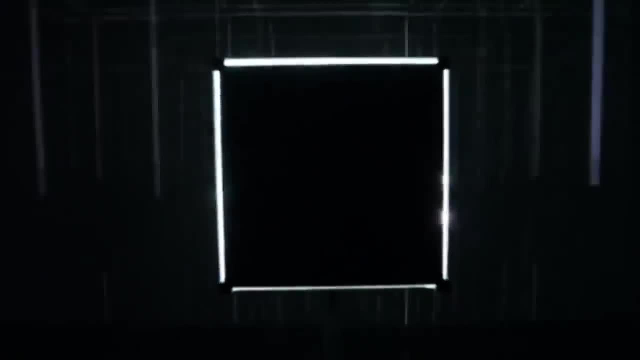 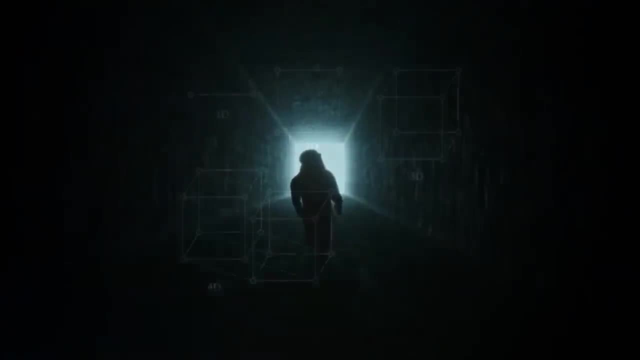 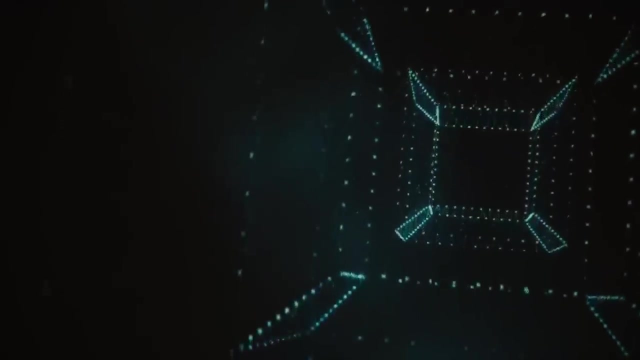 How many dimensions are there beyond our perception? For now, it remains a mystery. In the meantime, the world truly is multidimensional. Based upon a mathematical hypothesis, an infinite number of spatial dimensions can exist. Modern physics also adheres to this logic. 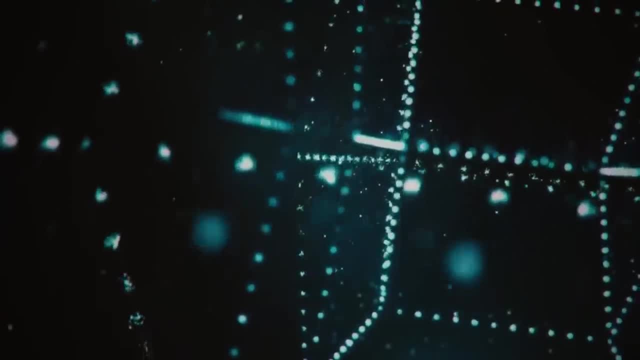 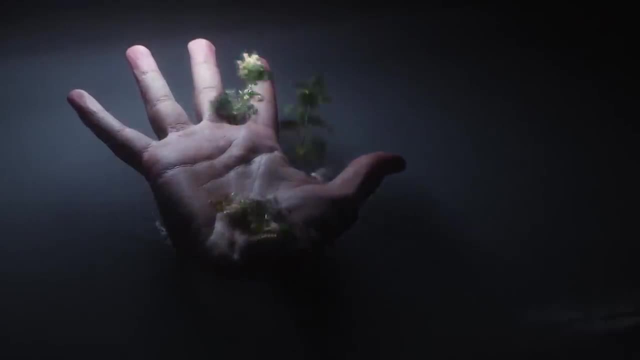 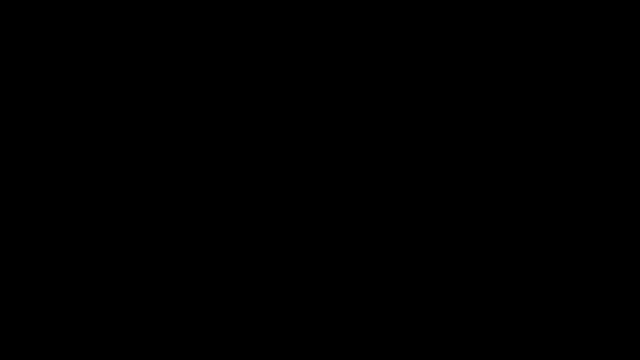 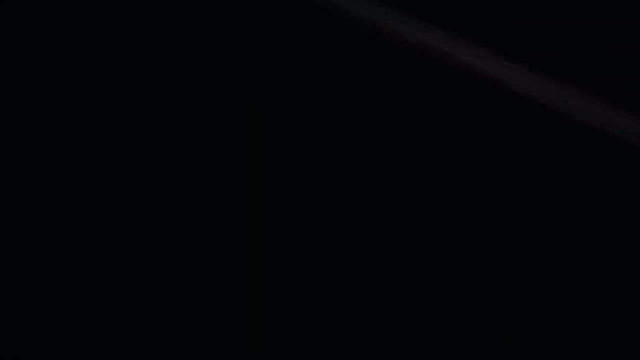 only it is impossible to count the number of these types of dimensions, But owning to the understanding of at least a few of the additional dimensions, we would obtain a good tool for managing the world around us. The Earth is a bigger than human. 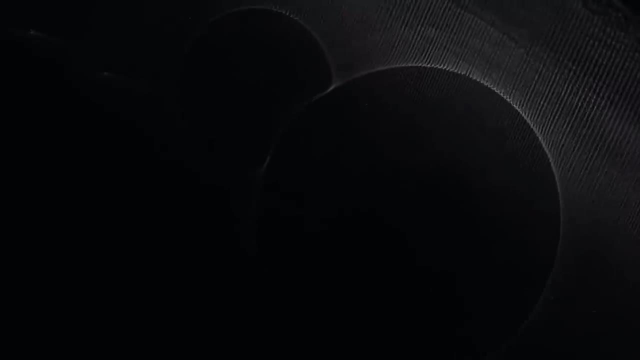 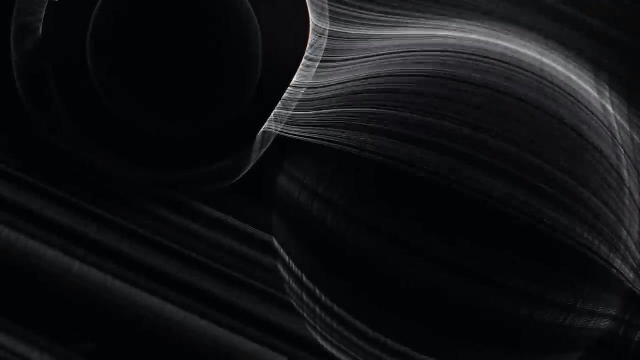 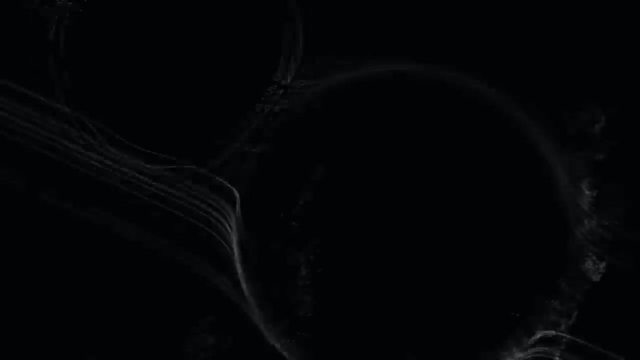 The earth is just a small, tiny part of the universe. The planet is just a small part of the universe. The earth is a small part of the universe. The earth is also a small part of the universe. Everything is so small that it can only be called a small part of the universe. 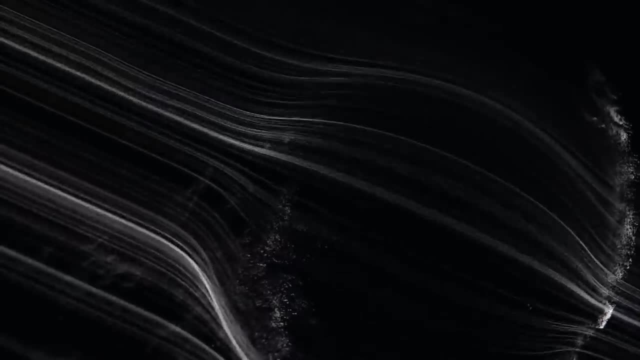 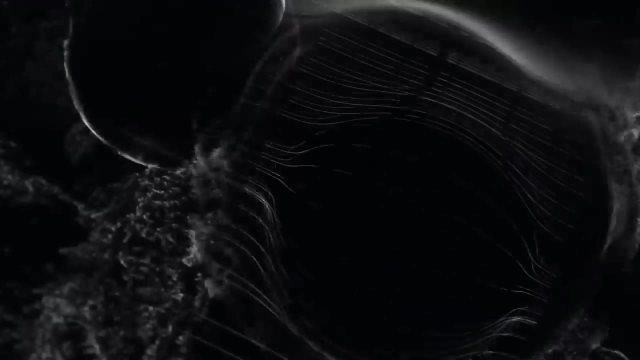 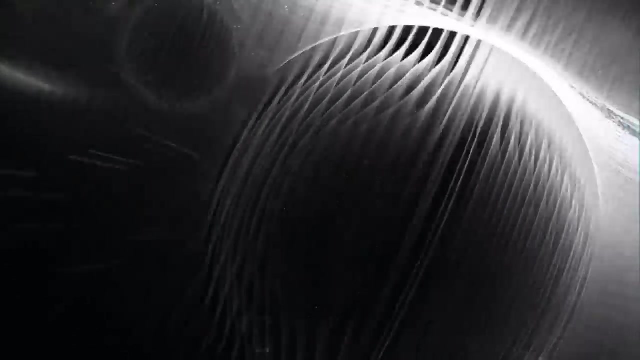 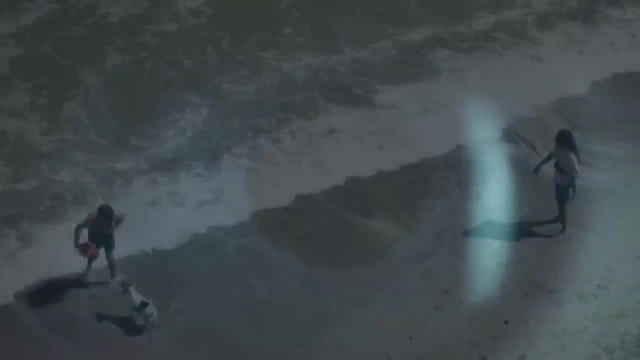 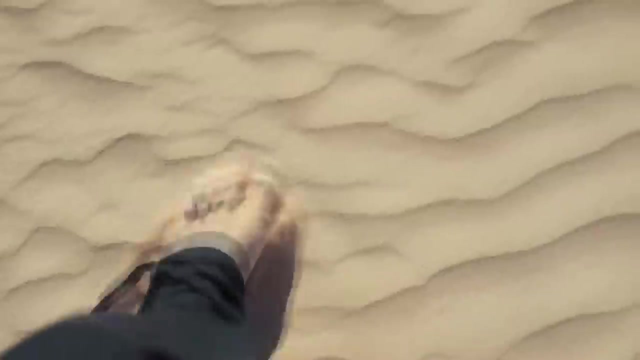 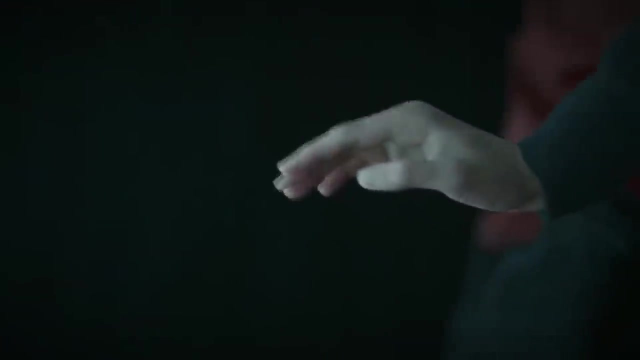 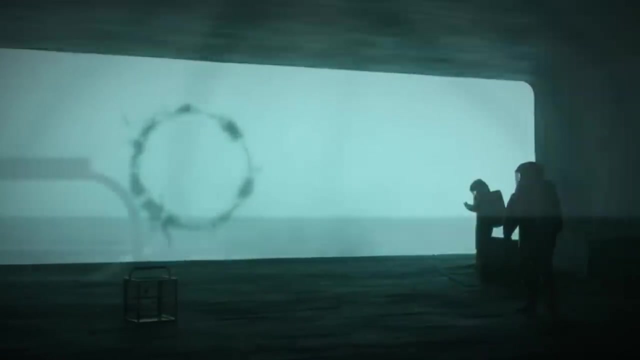 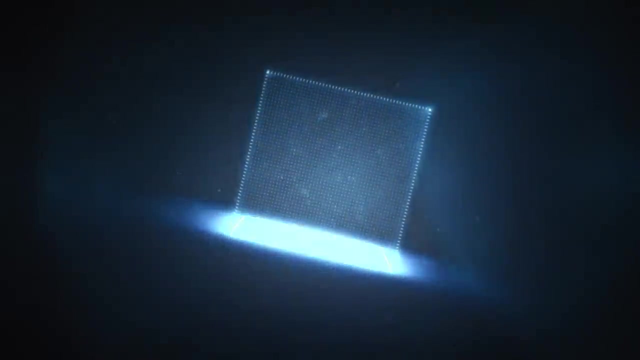 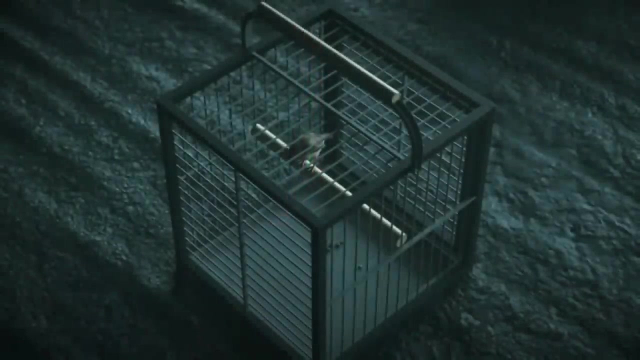 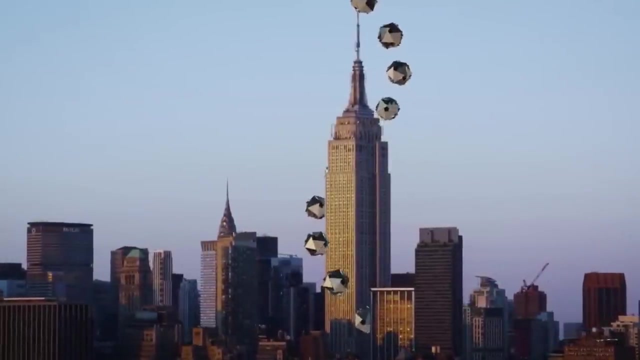 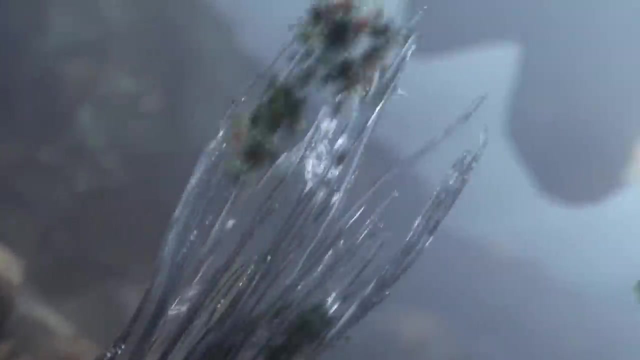 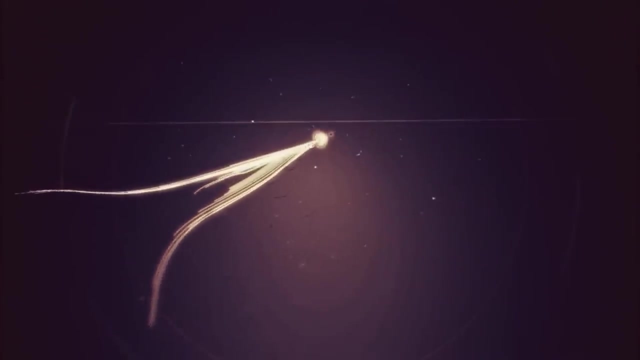 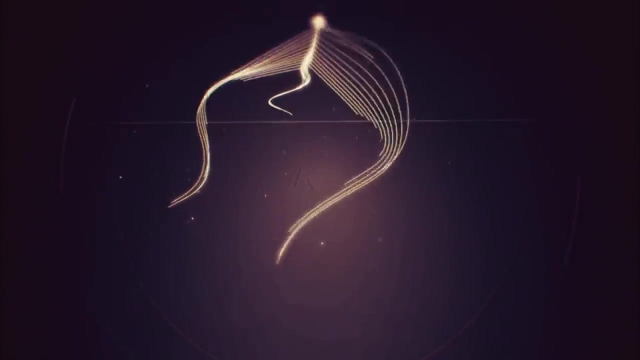 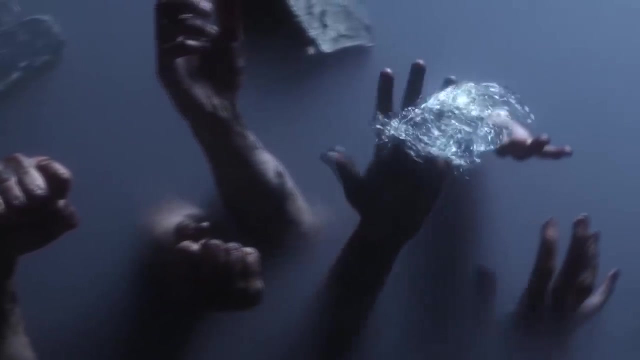 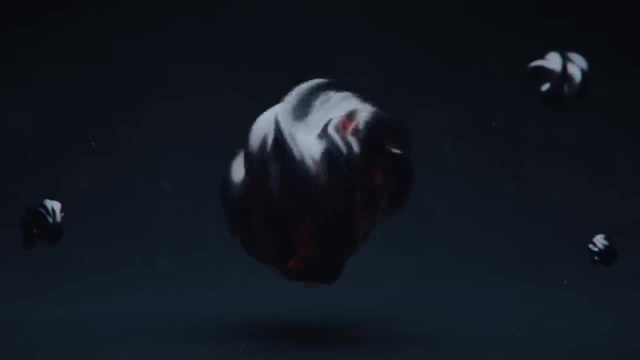 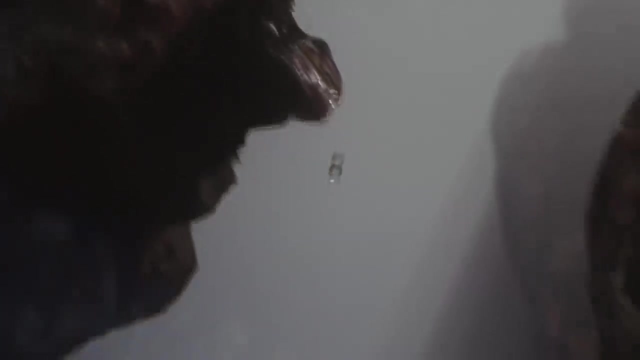 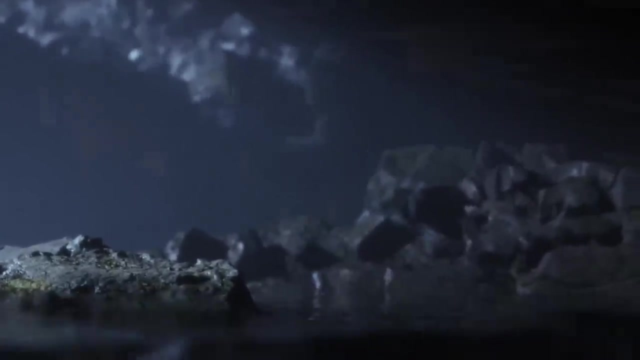 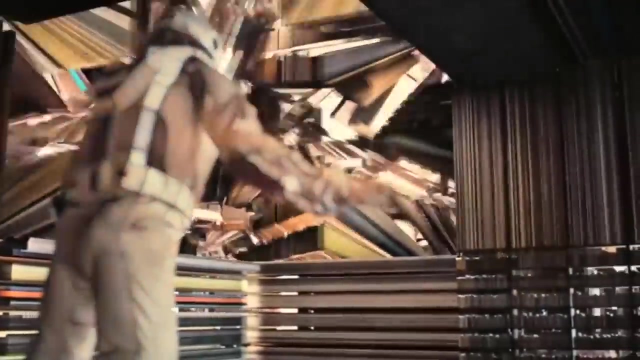 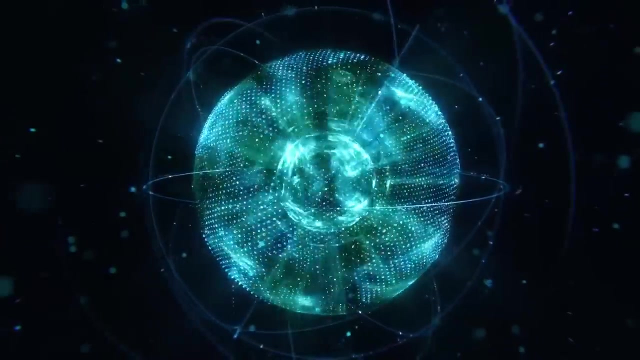 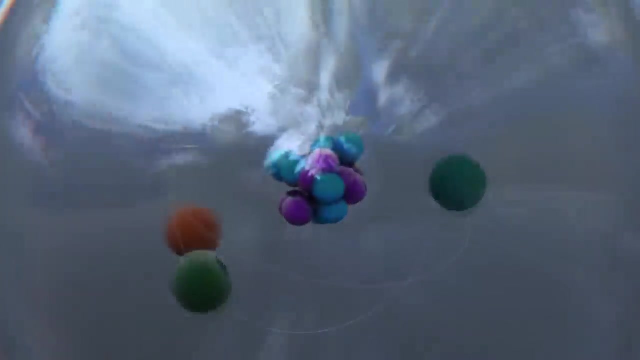 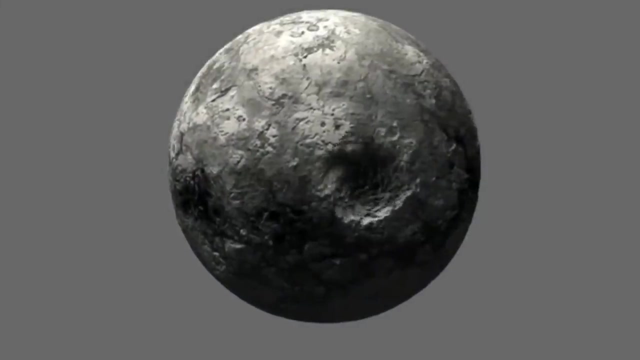 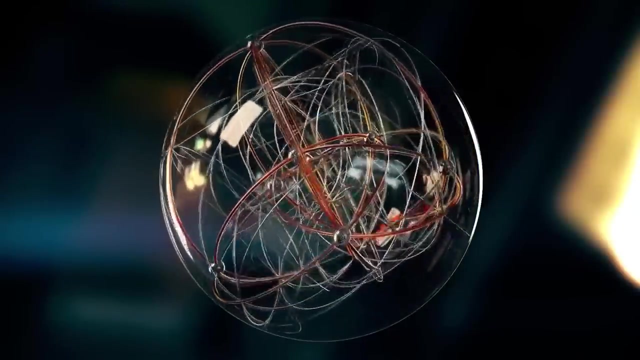 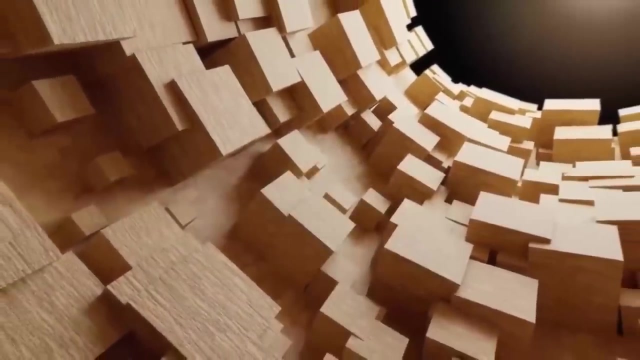 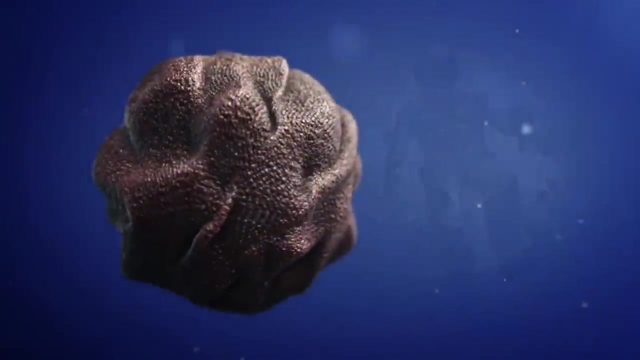 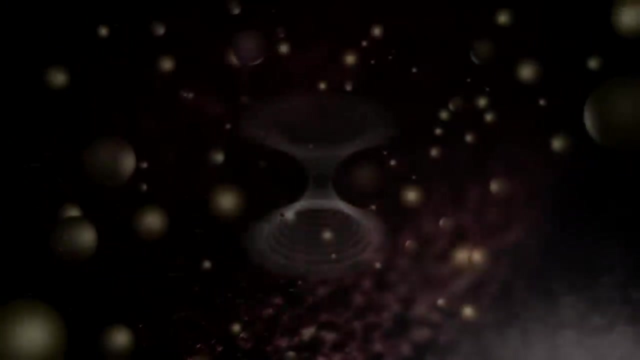 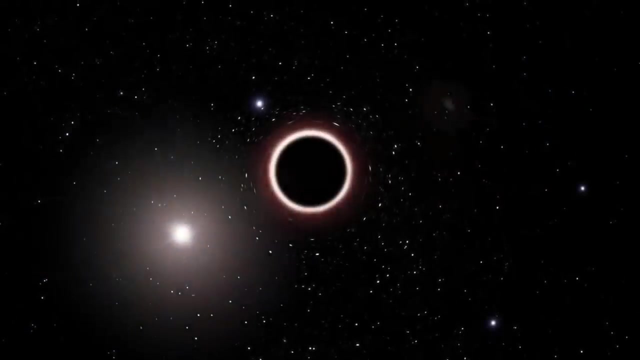 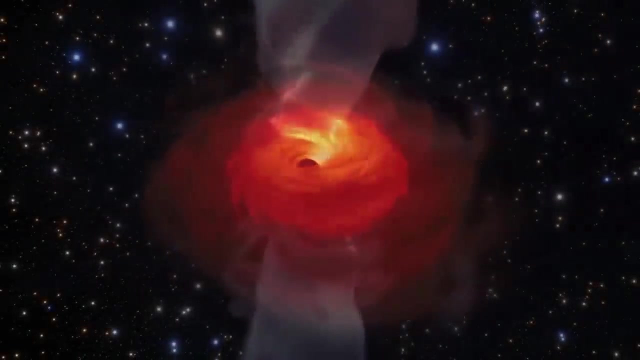 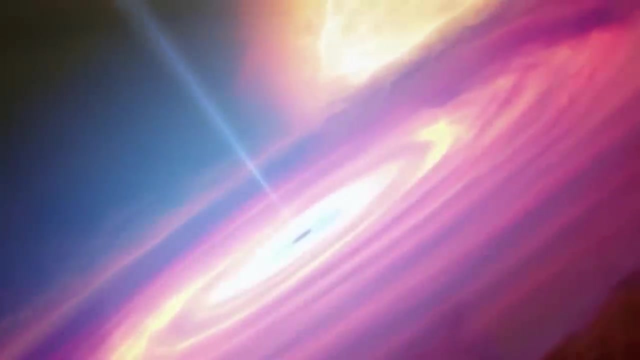 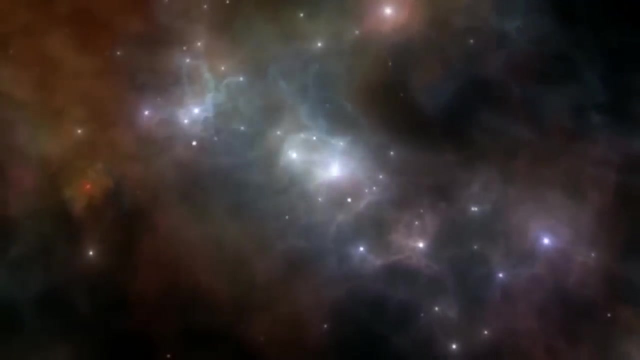 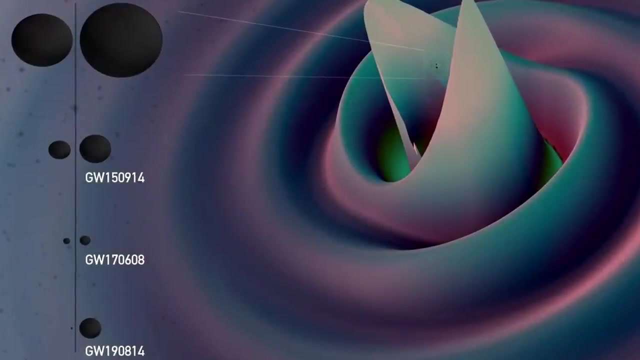 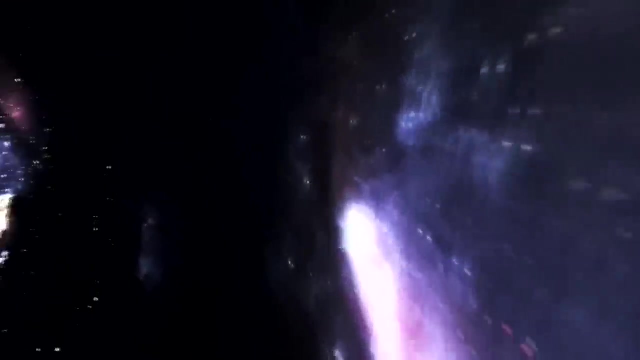 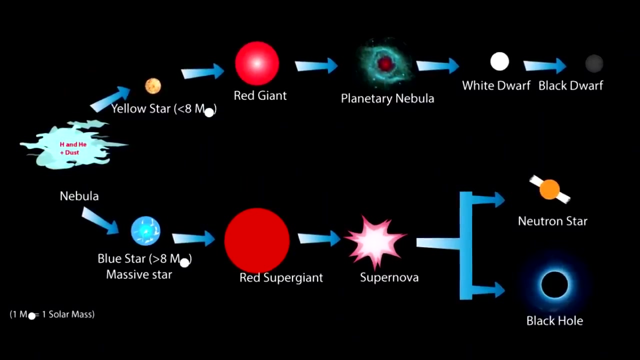 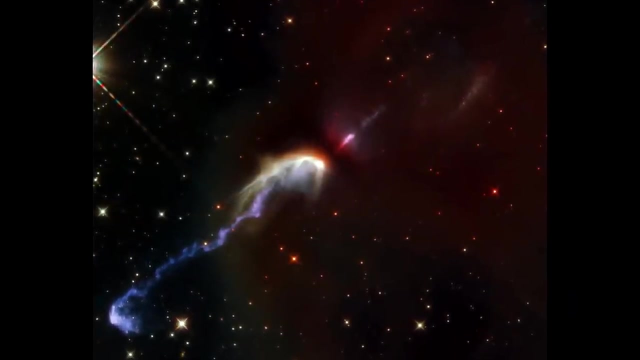 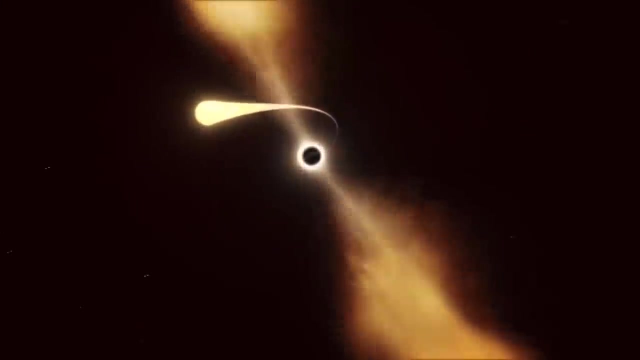 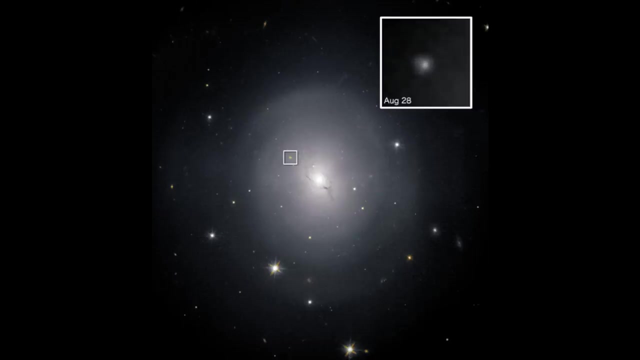 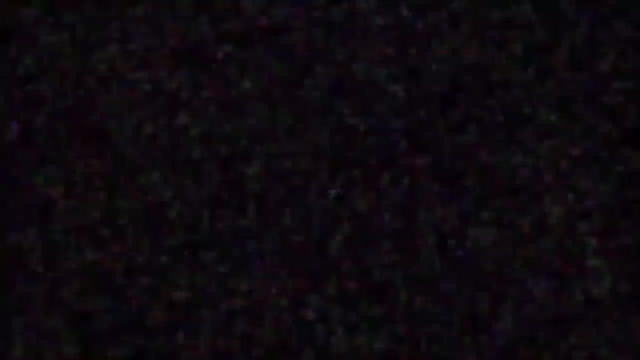 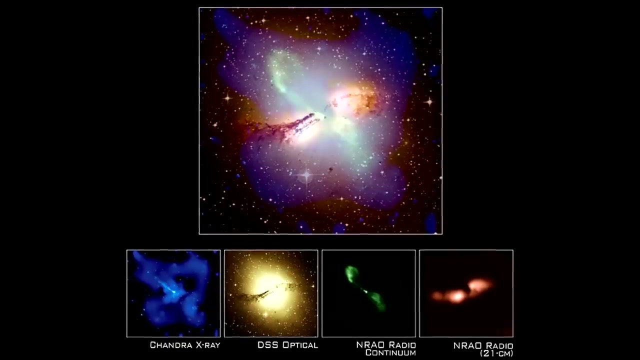 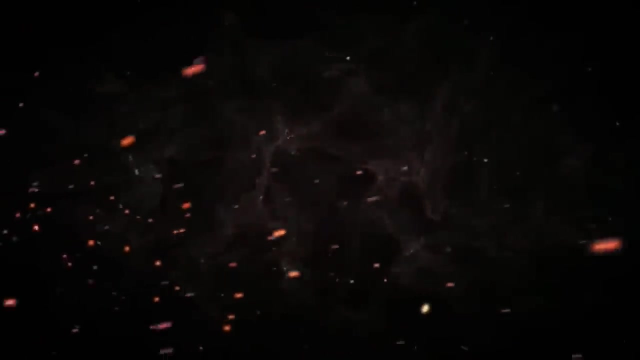 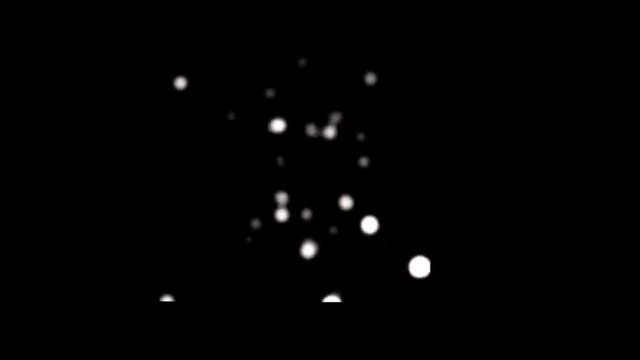 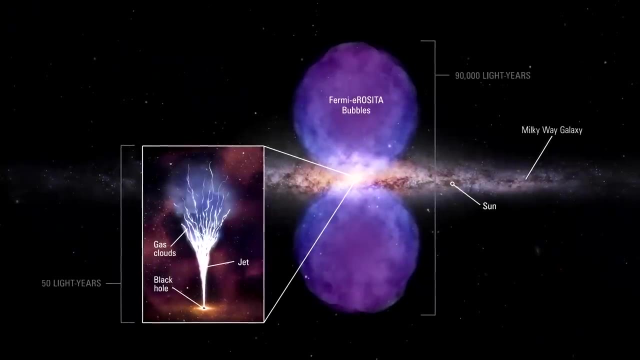 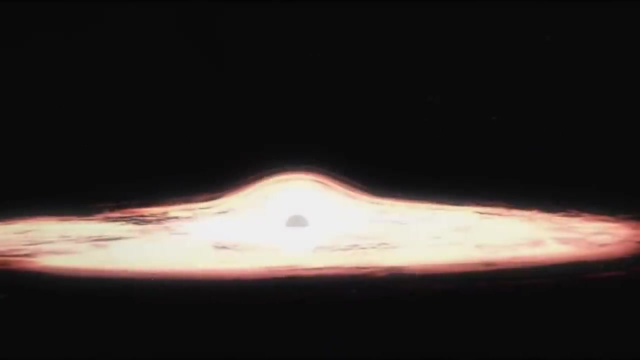 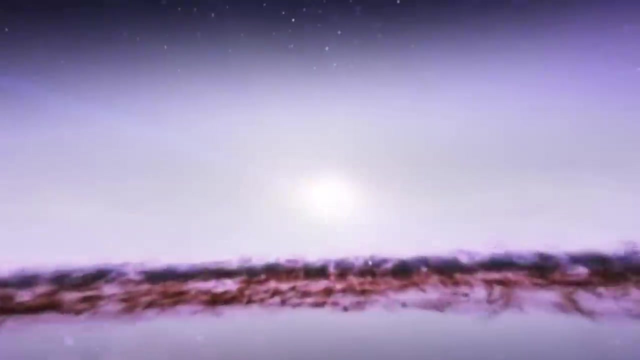 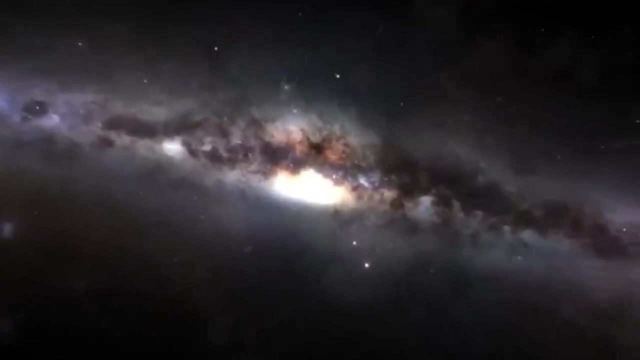 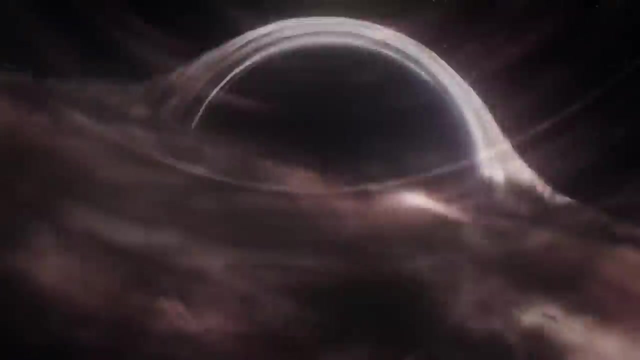 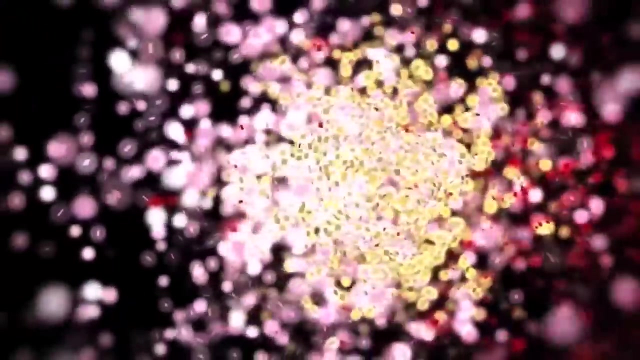 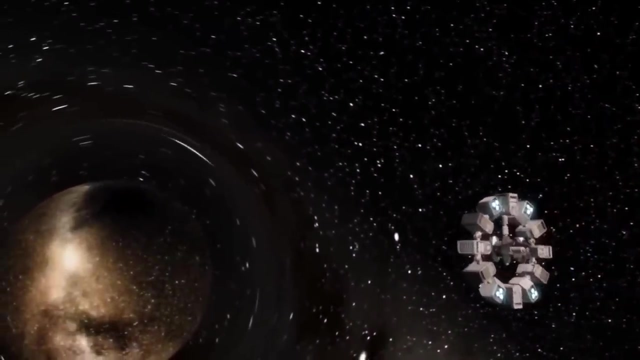 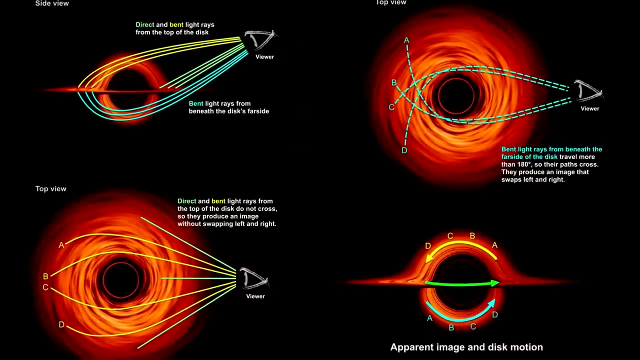 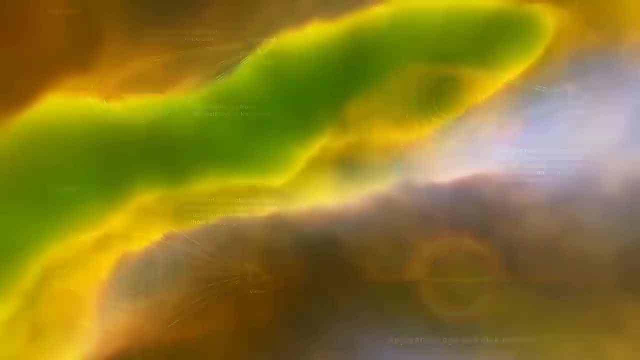 We'll be right back. We'll be right back. Quasars are galactic nuclei and have a black hole in their center. Quasars are incredibly luminous and small in size, and they can be observed at a distance of 10 billion light-years. 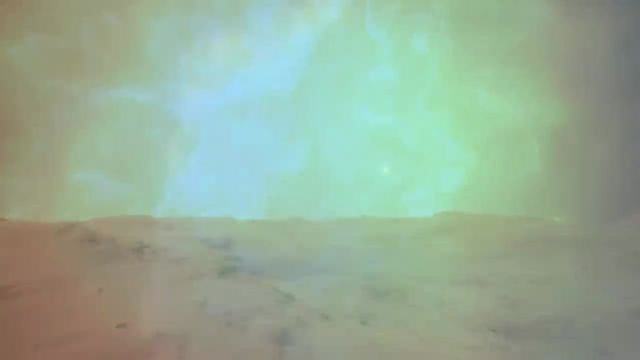 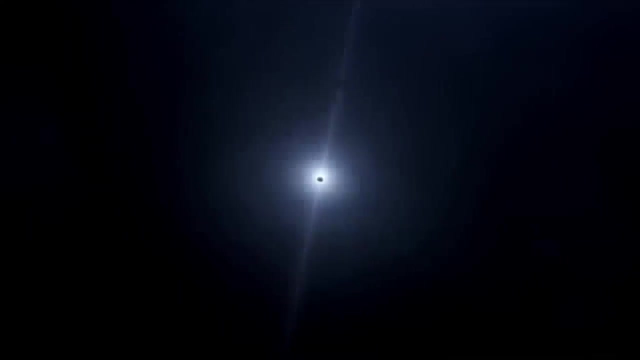 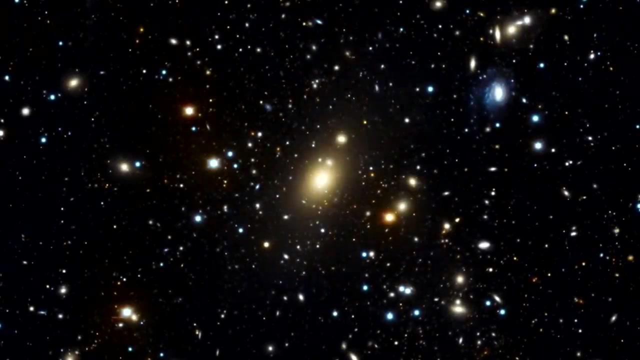 These objects emit a tremendous amount of energy in all of the regions of the electromagnetic spectrum, and especially in the infrared region. It is precisely this type of massive black hole that interests us. However, as a rule, a commonly accepted theory of the formation of black holes of this sort of mass 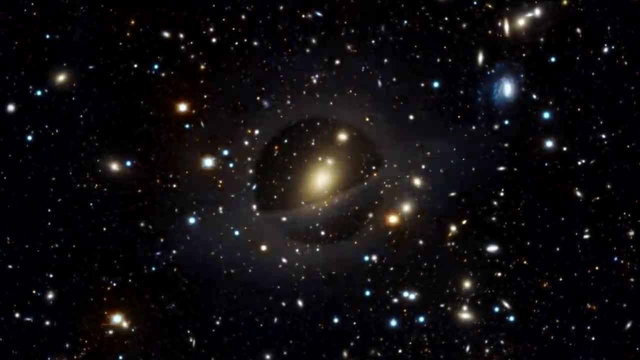 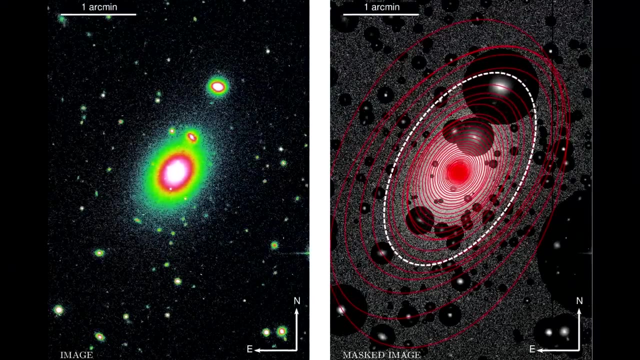 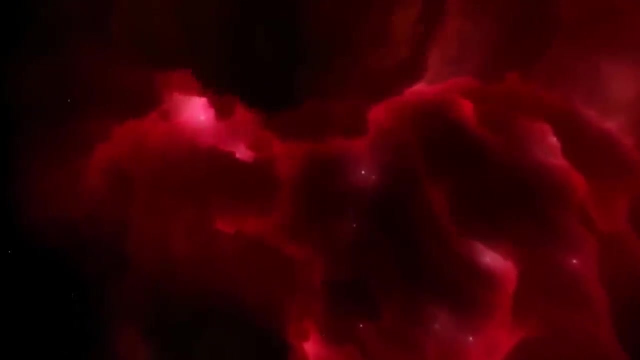 similar to that in the center of galaxy CID 947, does not yet exist. Galaxy CID 947 is a most ordinary galaxy. The total mass of its stars is just 45 billion times the total mass of its stars is just 45 billion times the total mass of its stars. 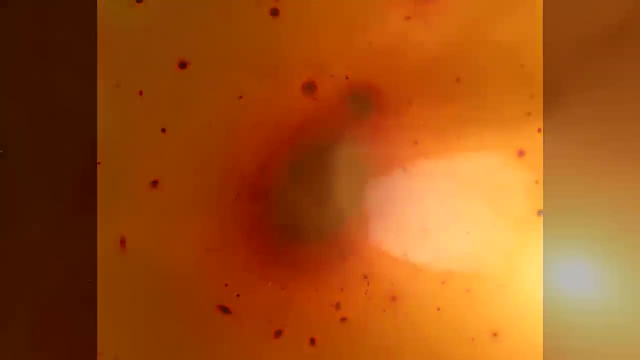 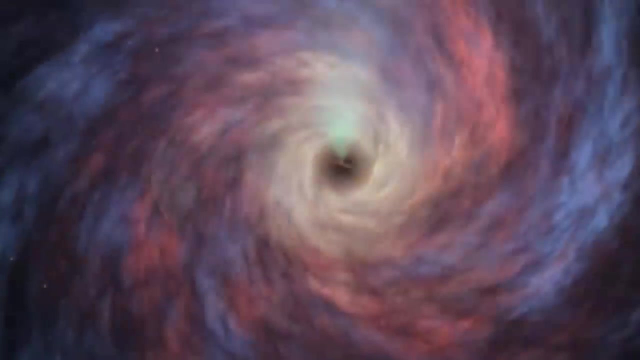 greater than that of our sun. For comparison, this figure for the Milky Way, which is considered a fairly small spiral galaxy, is 64 billion solar masses, But at the same time the mass of the supermassive black hole at its center. 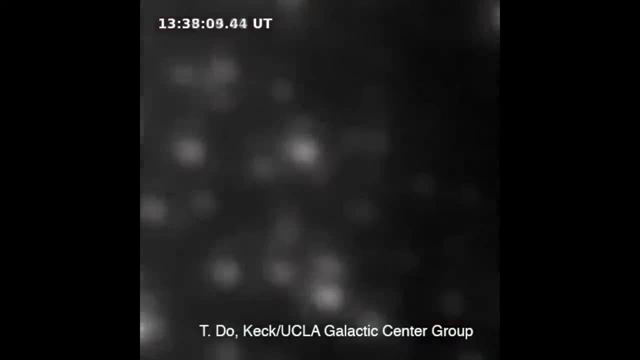 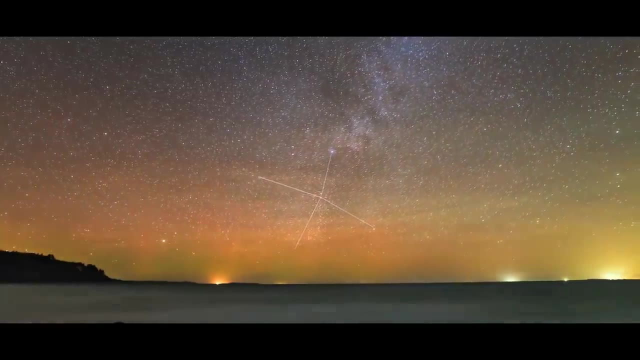 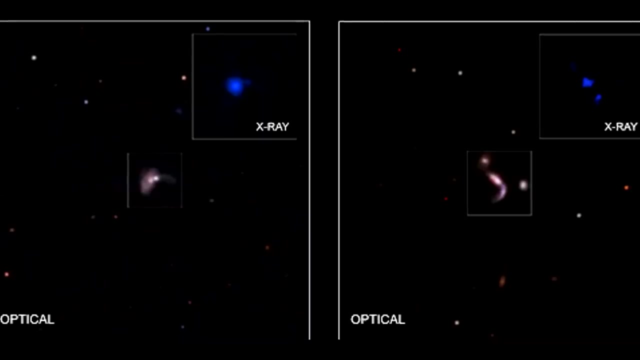 turned out to be inordinately large. According to the calculations, its mass exceeds that of the sun by almost 7 billion times, which makes this object one of the largest black holes in the universe- early universe- and makes it the leader in the weight category of galaxies of this size. 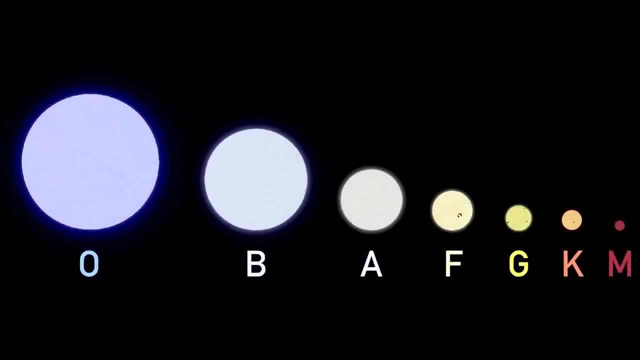 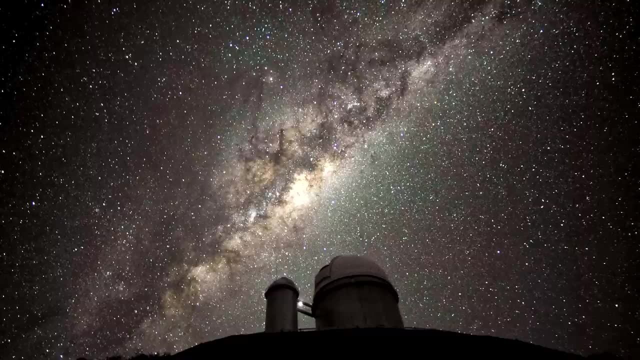 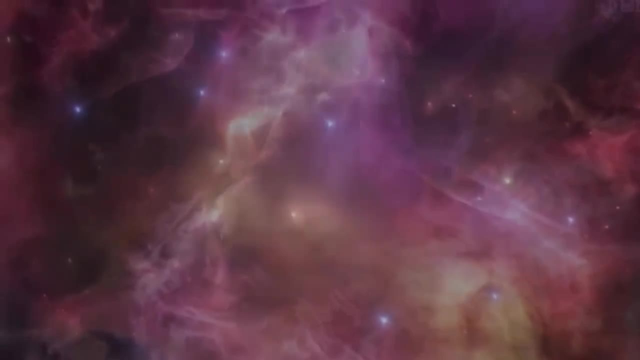 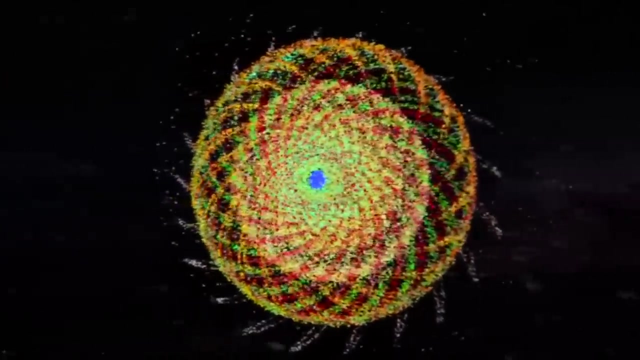 This sort of a finding completely contradicts the well-established theories about the growth of black holes in the centers of galaxies, which postulate that the stellar megapolises and the heavyweights living in their centers grow approximately the same rate and that their masses always maintain the same ratio of 1 to 500. 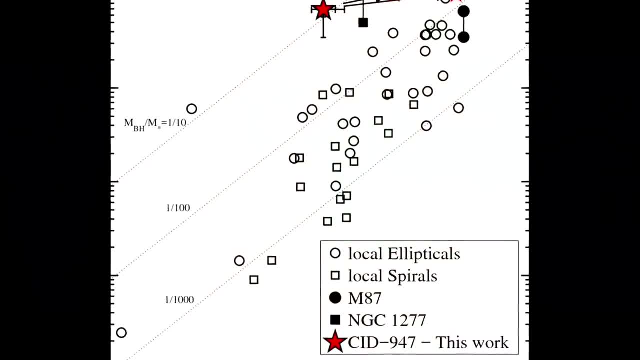 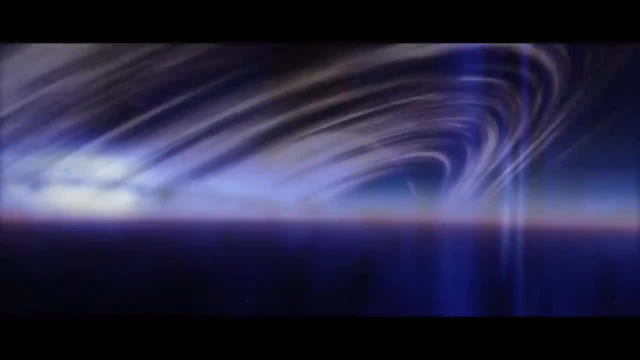 In the case of CID 947,, the black hole is only 8 times lighter than the entire galaxy. This means that it was growing much faster than the rest of the stellar megapolises, literally eating up almost all of the gas that fell into CID 947.. 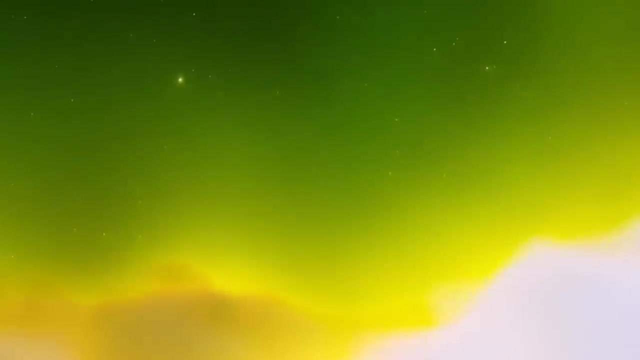 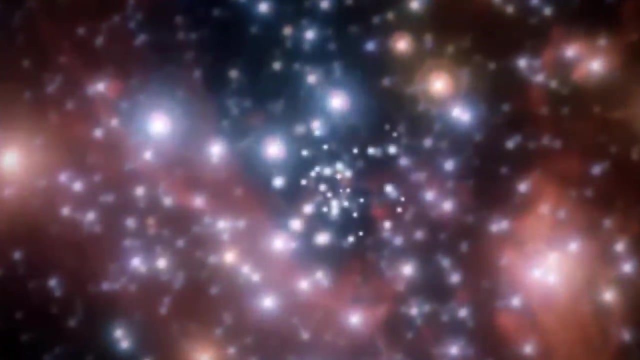 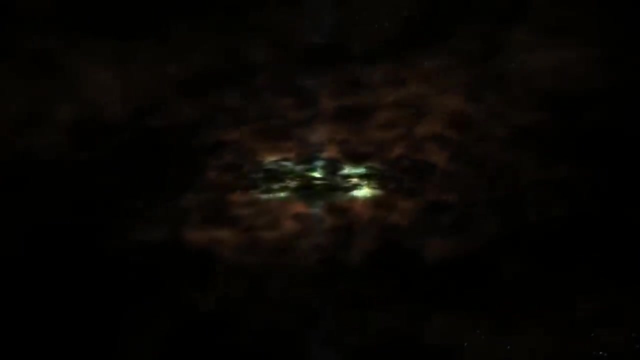 CID 947 from the intergalactic environment, which was relatively rich and dense compared to today. There is yet another oddity: CID 947 has already reached the limits of its growth, but new stars continue to be born in the surrounding galaxy. 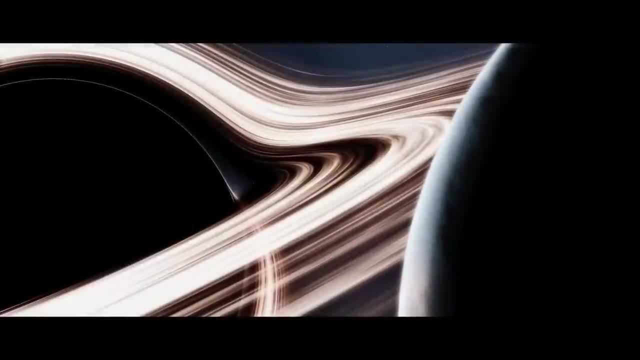 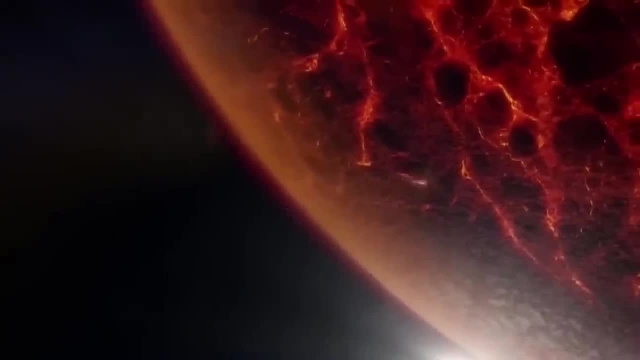 Until now, this was also considered impossible, since the radiation of the black hole and the gas flows surrounding it, in theory, should prevent the birth of new stars. But… It turns out to be a strange paradox, since a black hole both devours stars and facilitates. 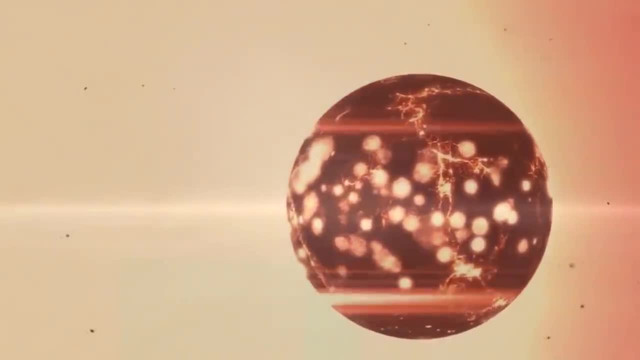 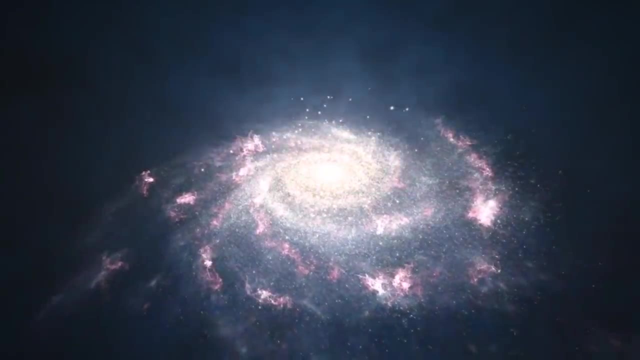 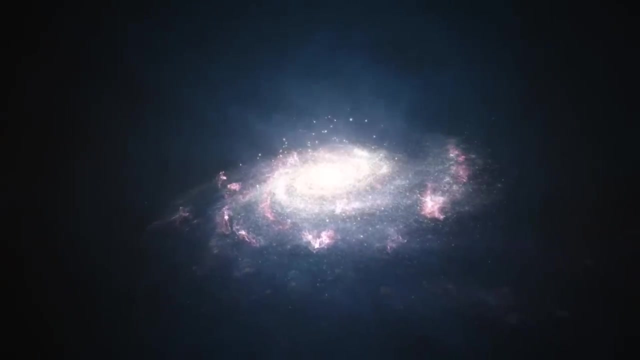 their birth. With the help of the Hubble Space Telescope, researchers mapped out the huge shell of gas that surrounds the Andromeda Galaxy, and they were astonished to find that this thin, almost invisible halo of diffused plasma extends 1.3 million light-years in space. 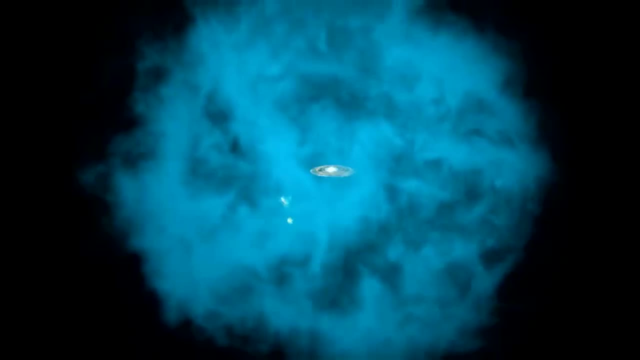 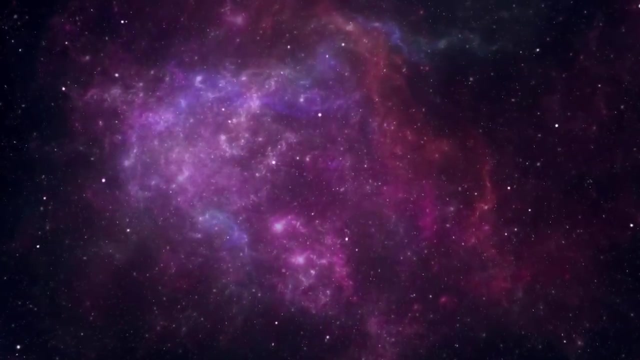 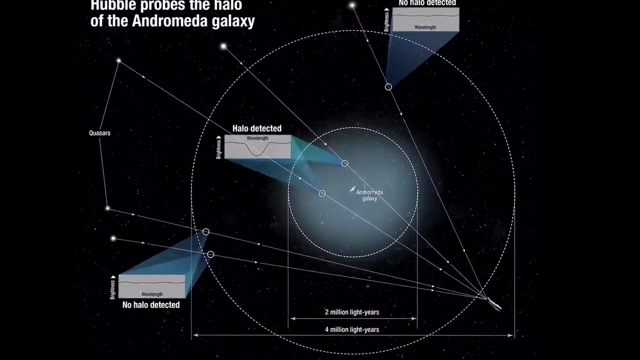 The galaxy is about half the size of our Milky Way and for 2 million light-years in other directions. This means that Andromeda's halo is already coming into contact with the halo of our galaxy. They also discovered that the halo has a layered structure, with two main layers and separate. 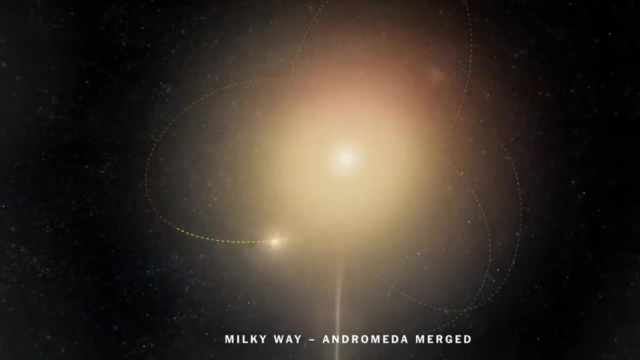 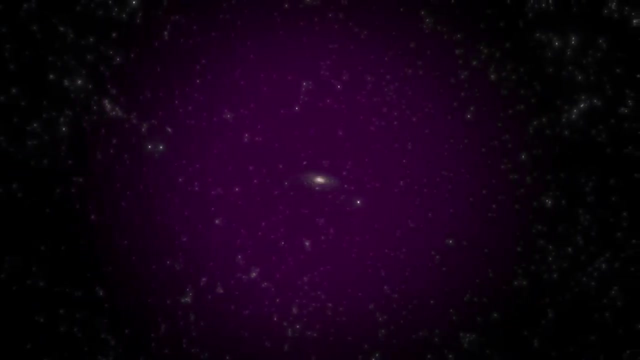 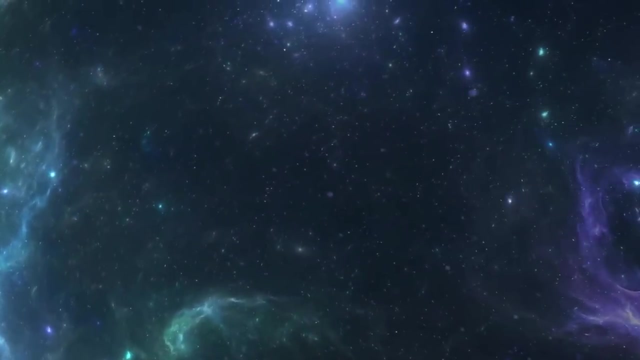 shells of gas. Understanding the huge gas halos surrounding galaxies is of crucial importance. The galaxy is a large galaxy. This reservoir of gas contains the material for future star formation in a galaxy, as well as the remnants from events such as supernovas. 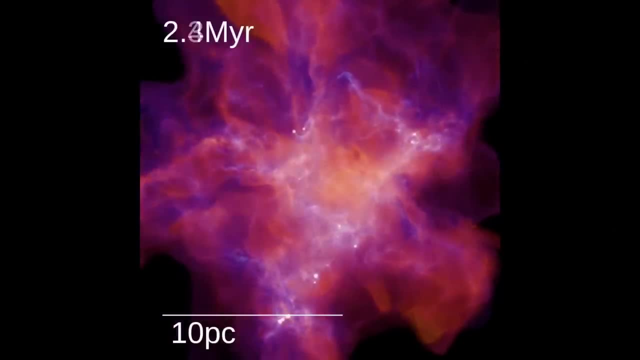 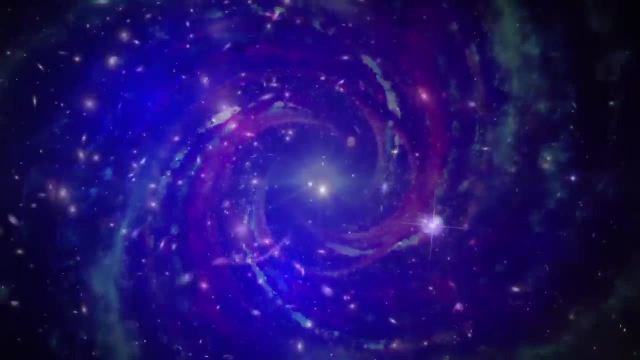 It is filled with clues to the past and future evolution of the galaxy. It became clear that the inner shell, which stretches out about half a million light-years, is much more complex and dynamic, while the outer shell is smoother and hotter. This difference is likely the result of the activity of supernovae. 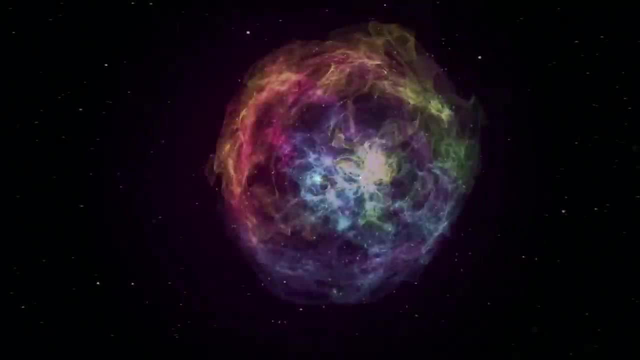 The galaxy is also known as the Milky Way. The fact that the inner circle of this galaxy is the center of the galaxy is a reference to this. If this is not the case, as a result, there may be some negative evidence that, more than one in a million light-years of its own universe exists in the galaxy. The galaxy is also known as the Jupiter or our galaxy's star. This is the definition of the activity of supernovae in the galaxy's disk. having a more direct 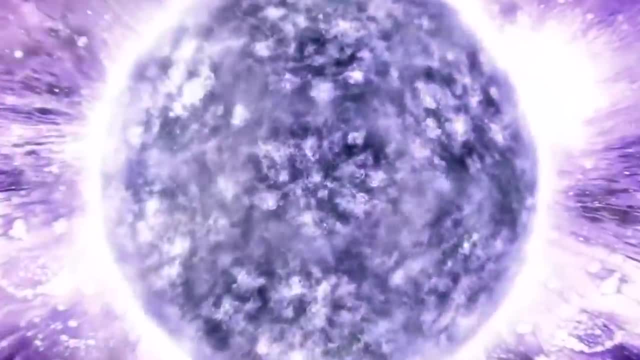 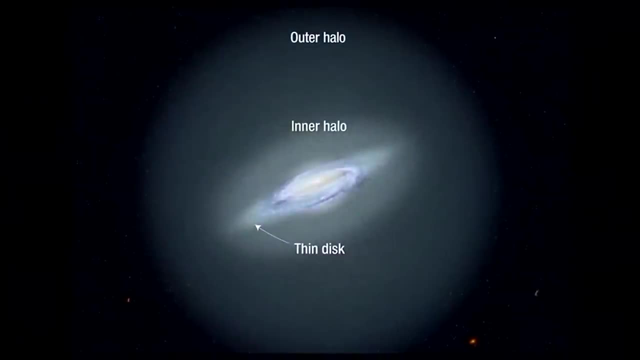 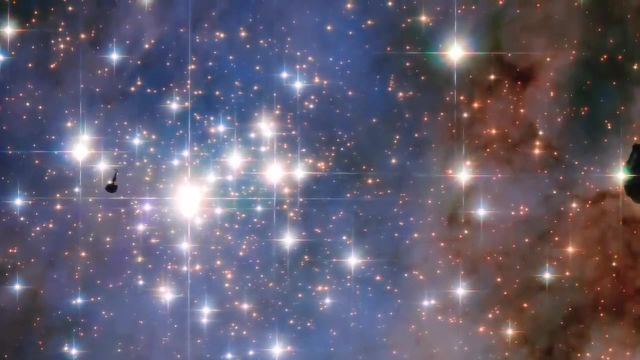 effect on the inner halo. However, since we live within the Milky Way, it is not easy to deduce the profile shape of the halo of our own galaxy. It is presumed that the halo of Andromeda in the Milky Way must be very similar. 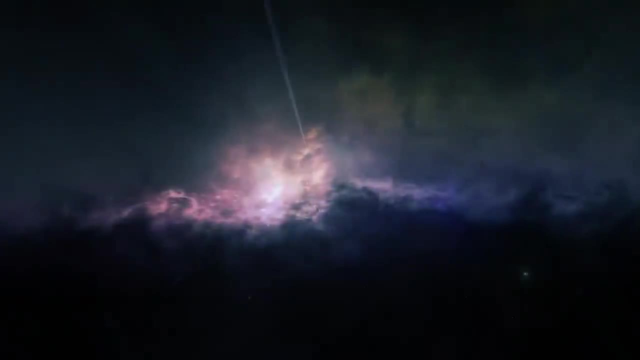 Since these two galaxies are similar in shape, we should try to identify a similar form of Andromeda. This might be possible in the case of Oresean. This might be possible in the case of Oresean, Since these two galaxies are also incredibly alike, both in relative size and in appearance. 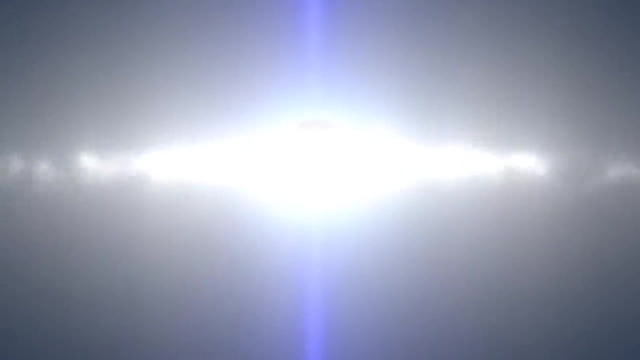 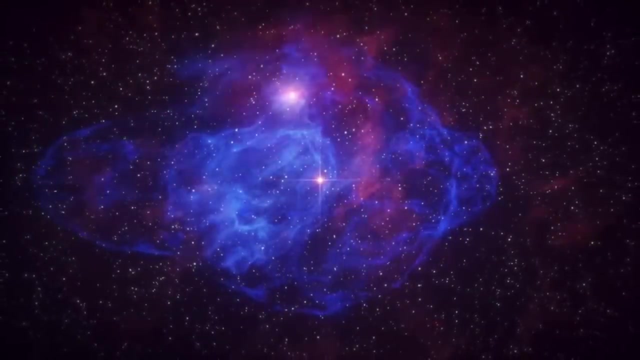 as modeling of the movement of the galaxies has indicated, they are both on the path to collision and will merge, forming a giant elliptical galaxy, in about 5 billion years, But their weak halos have indeed already begun to come into contact with each other. 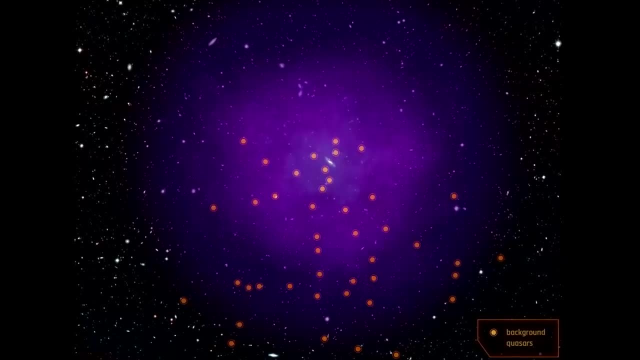 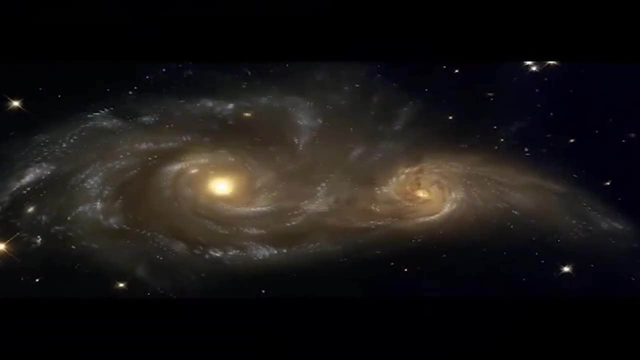 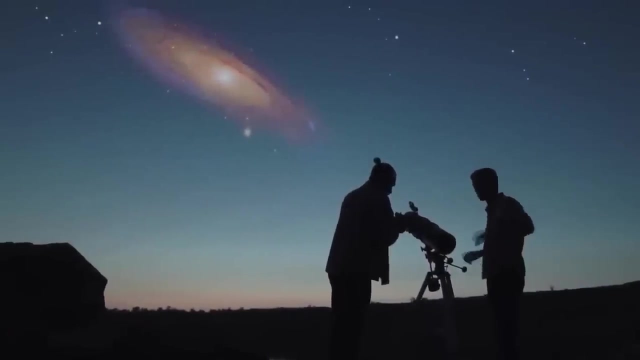 Thus we can say that the merger, although almost insignificant, has already begun And there is no force that can stop this merging. But the question then becomes what will happen to the galaxies if they are viewed from the side? In a collision, large galaxies absorb smaller ones entirely. and it practically does not affect their structure. However, when galaxies are close in size, like the Milky Way and the Andromeda, the collision causes their structure to collapse. A number of stars will be ejected from the galaxies, Others will be swallowed up by the merging of supermassive black holes. 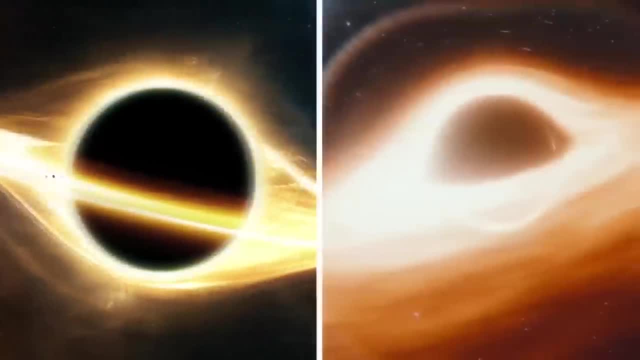 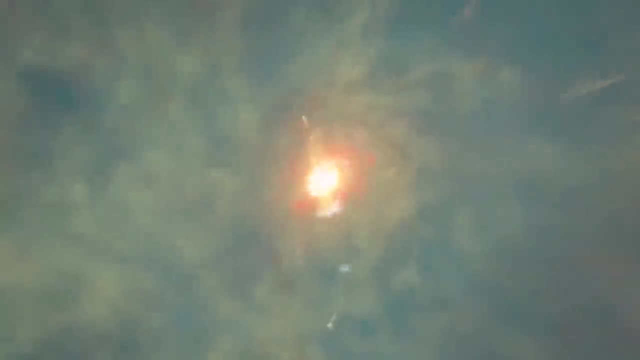 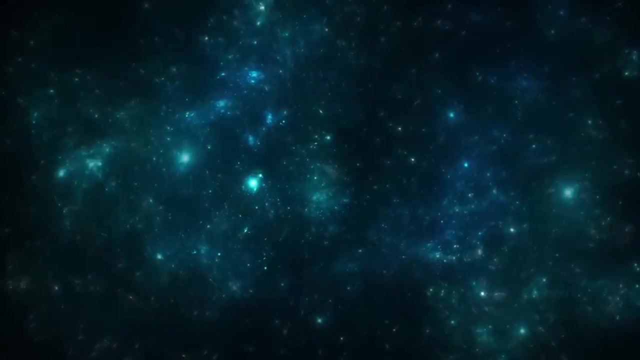 At the same time, the beautiful spiral structure of both galaxies will be disrupted and a new giant elliptical galaxy will form in their place. These kinds of mergers could bring about a small upsurge in the formation of stars. The collision of galaxies forms vast hydrogen clouds. 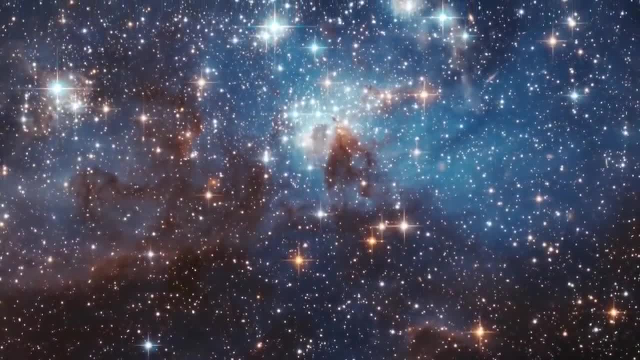 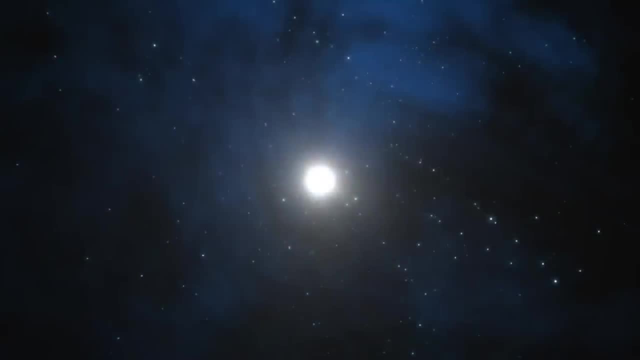 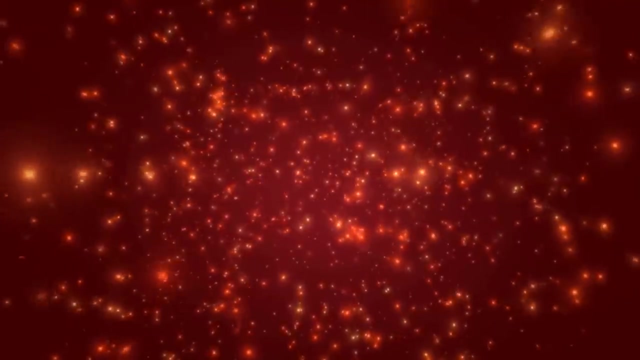 which can trigger a series of gravitational collapses. In addition to that, such mergers can be responsible for the premature aging of galaxies, as most of the gas turns into stars After a burst of star formation, the galaxies run out of fuel. The youngest and hottest stars explode as supernovae. 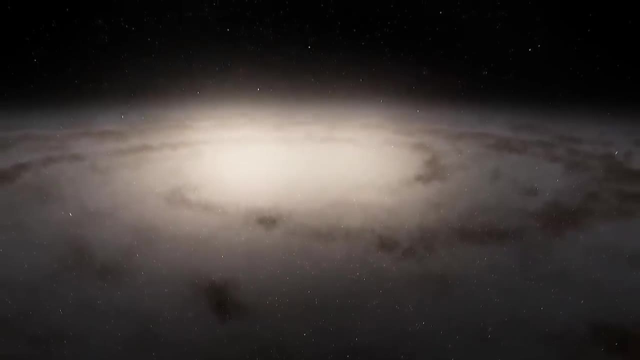 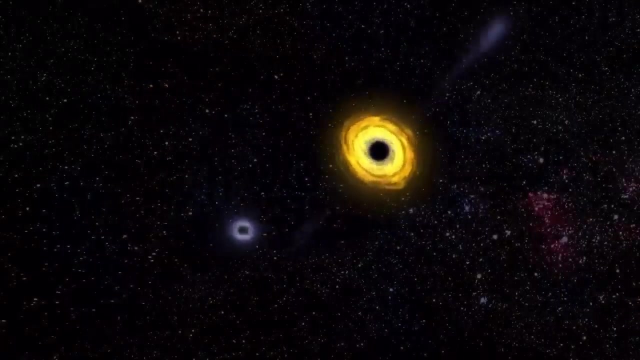 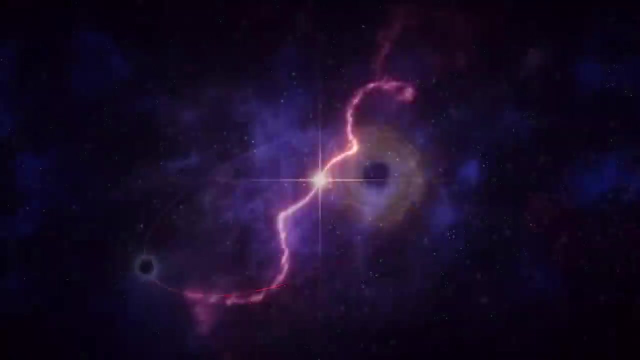 and all that remains are the old, cold red stars which leave for a very long time. This is why giant elliptical galaxies, the result of collisions, contain so many red stars and so few active star-forming regions. By the way, the merging of black holes will cause orbital energy to be transferred to the stars. 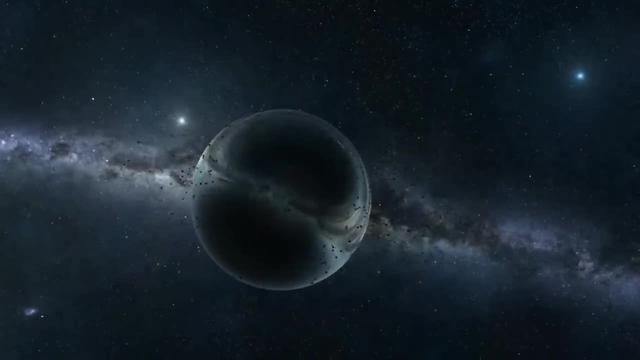 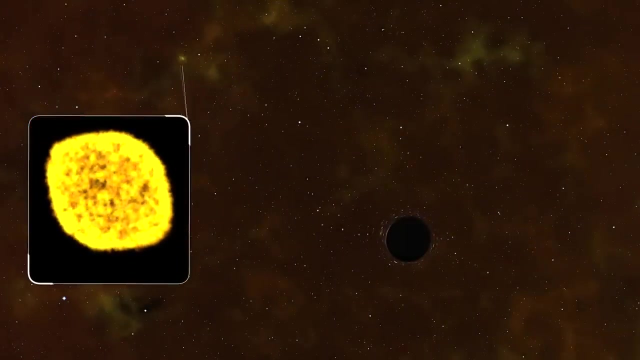 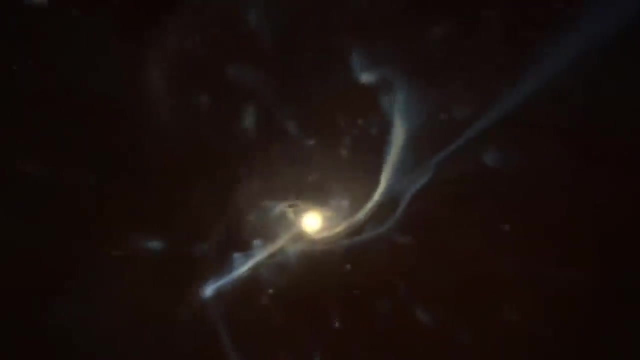 which will subsequently move the stars to higher orbits over millions of years. When two black holes come within a light year of each other, they will start emitting gravitational energy, which will cause the stars to turn into gravitational waves. The gas caught up by the combined black hole could create a glowing quasar. 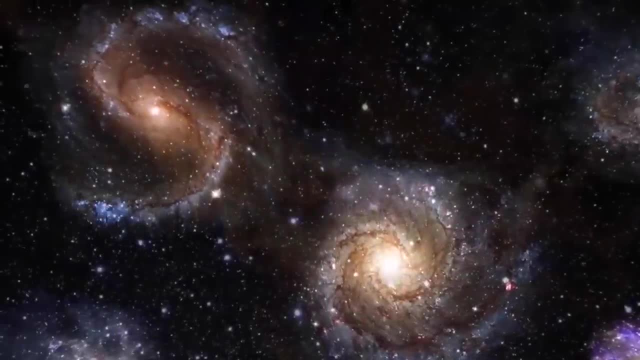 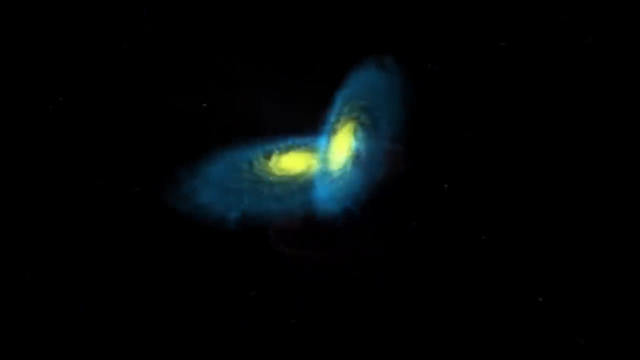 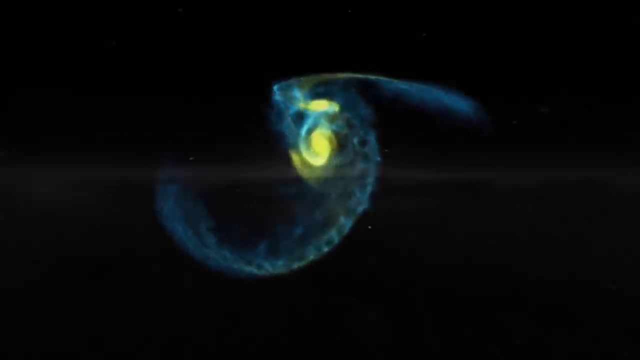 or active nucleus at the center of the reformed galaxy. And finally, an effect of the merger of black holes can be to give a good cosmic kick to some stars which will become genuine castaways, taking their planets with them. Who knows, maybe the universe will cast us off. 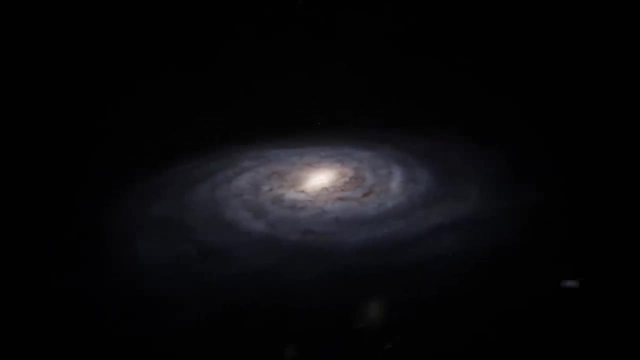 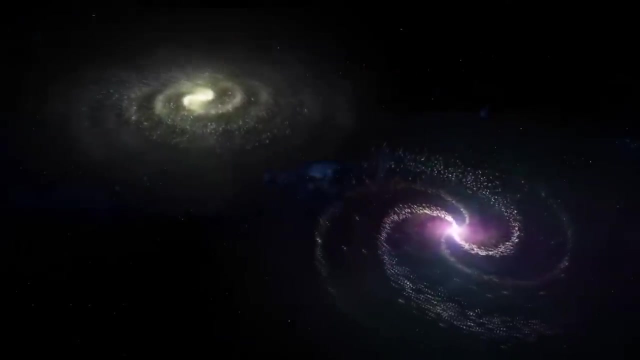 Well, the collision of galaxies will happen to any of them as soon as they inadvertently graze each other. In some cases, the galaxies merely brush each other in passing. In others, direct impacts follow, like a head-on collision of cars. 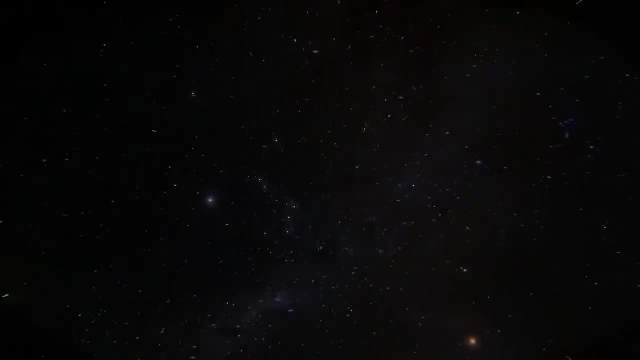 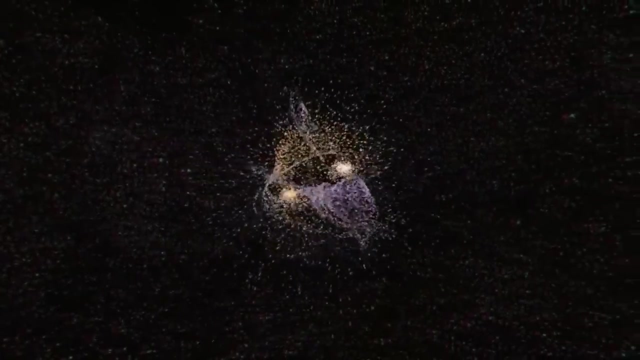 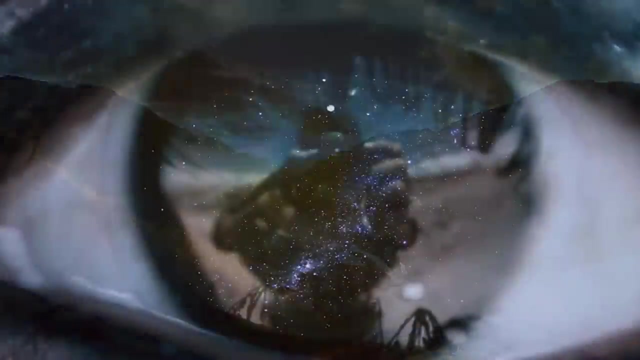 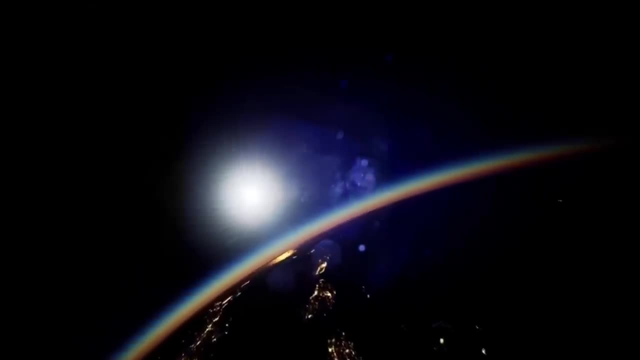 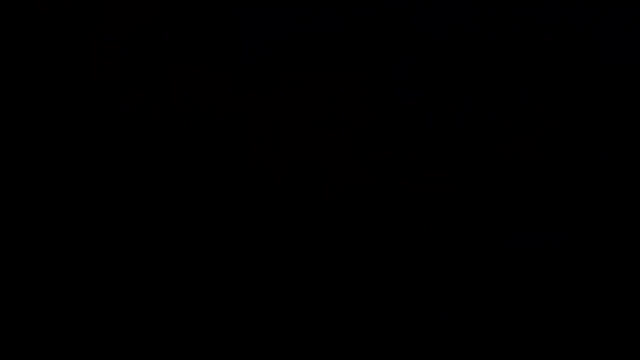 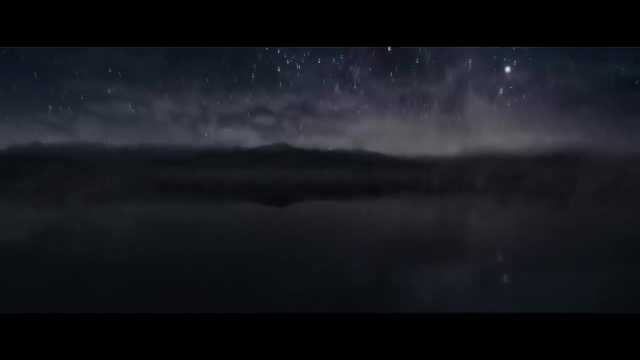 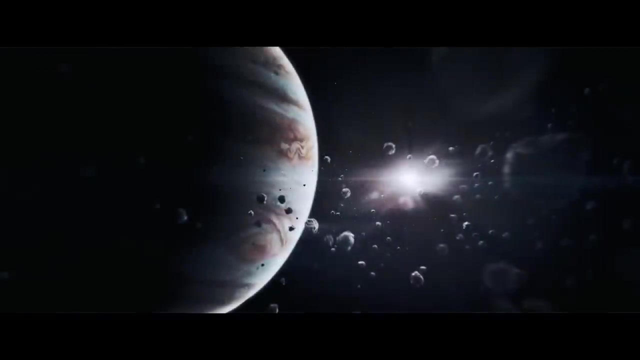